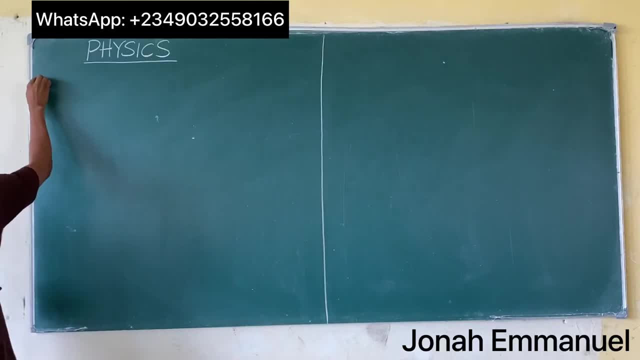 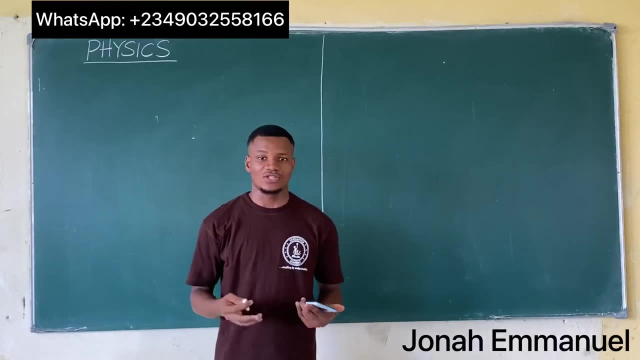 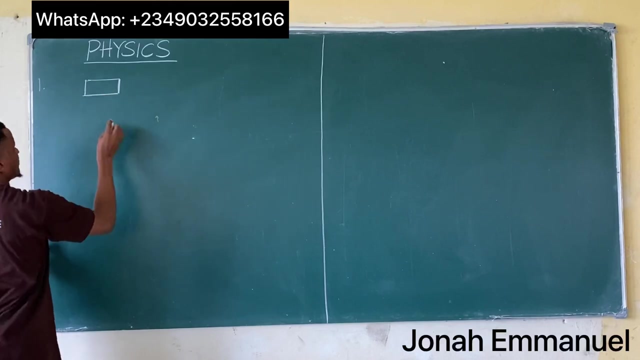 First of all, we said a resistor is the device used to measure resistance. Of course, resistance is simply the opposition to the flow of electric current in a circuit. Now, usually for a resistor, the circuit symbol is this. So this is the circuit symbol for a resistor. 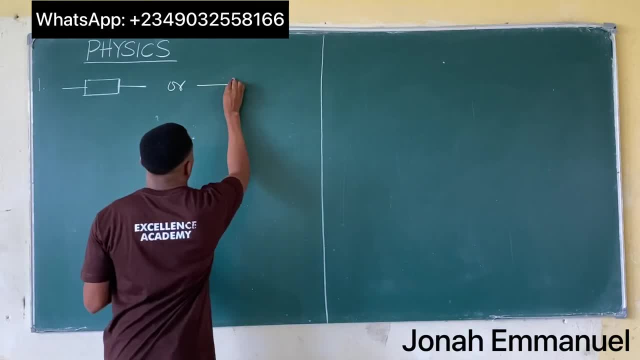 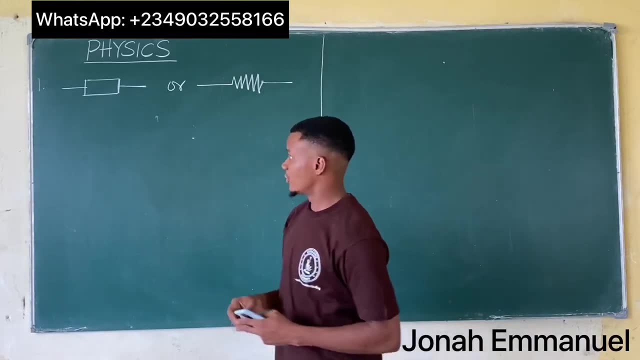 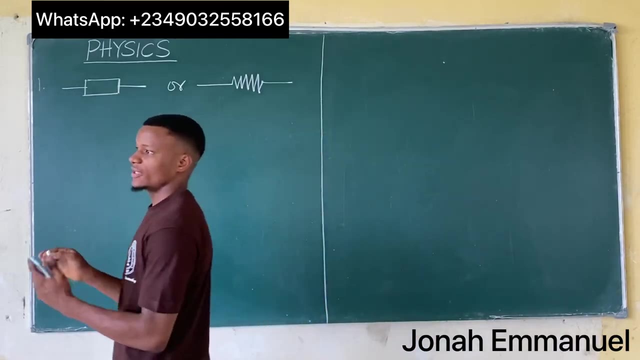 This, or In fact, we have this Alright. so this is your resistor circuit symbol. Can we see any of these? It represents a resistor, Also for a resistor. note that when resistors are connected in series, in series, resistor in series. 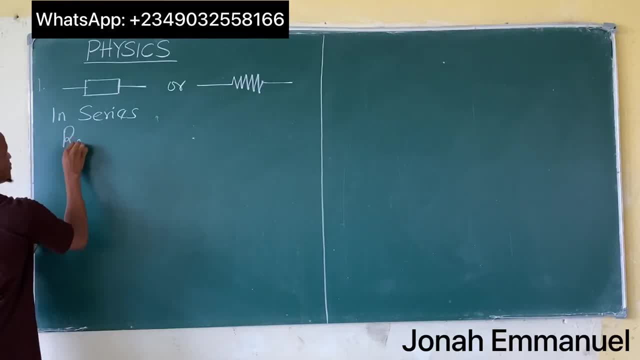 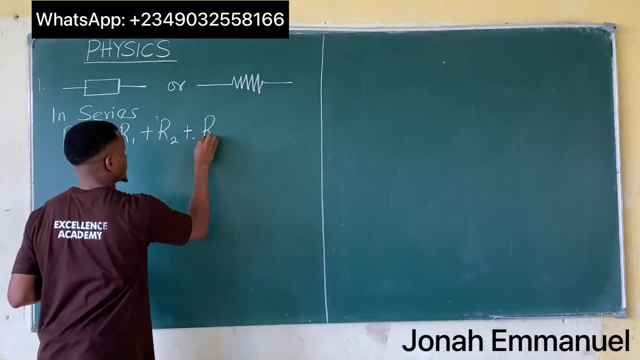 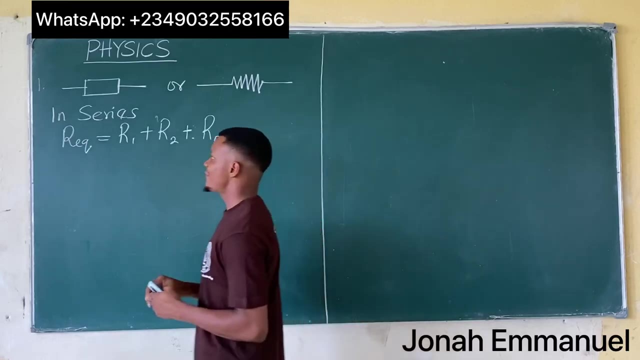 that the equivalent resistance- let's say Req equivalent resistance- is equal to the sum of all the resistors up to N. So just simply sum them up. that's for resistors, If you have resistors in parallel, in parallel. 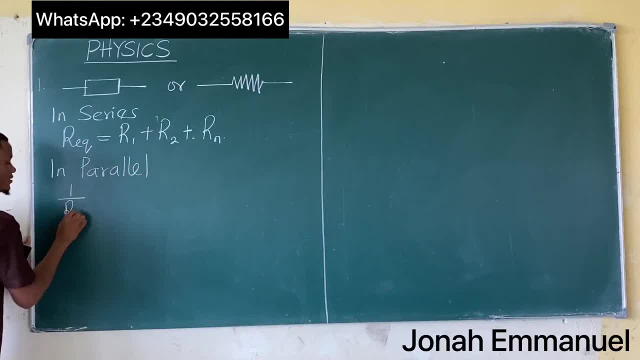 for parallel condition of resistors, we have that to take the inverse, So the inverse of the equivalent resistance is equal to take the inverse of each of them and thus continue up to this right, So up to the number of resistors. 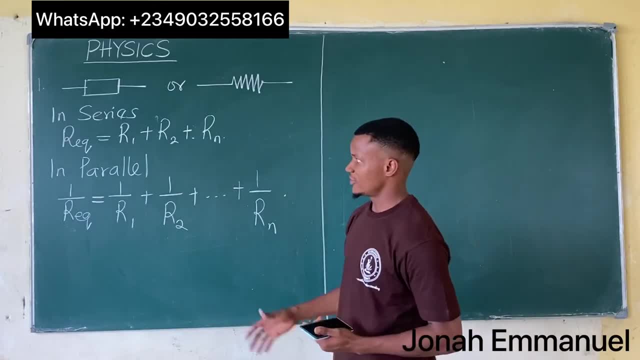 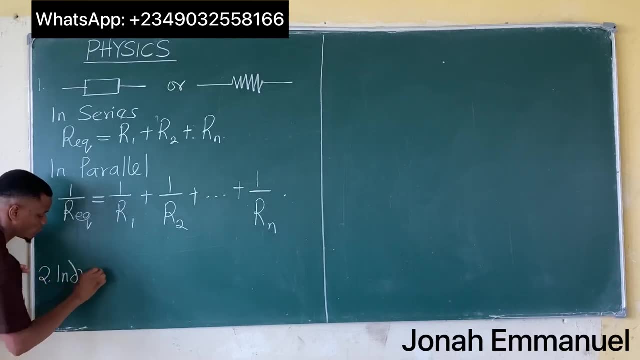 So if you take this in our previous classes- I'm just trying to refresh your mind- This is for resistors. Number two: let's look at inductors. For inductors, your circuit symbol for an inductor is this: 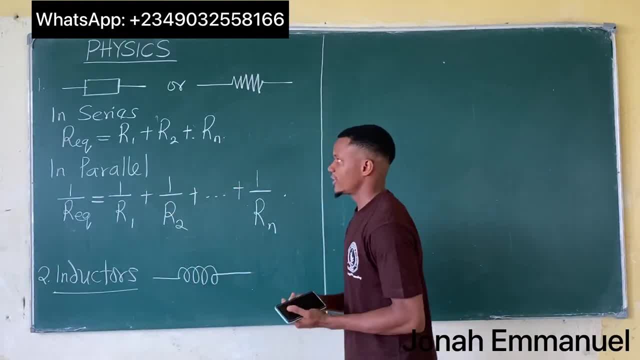 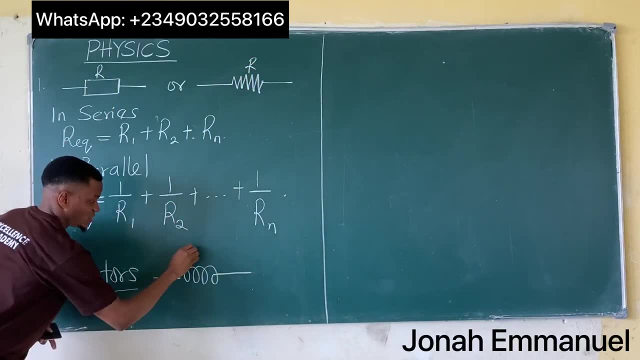 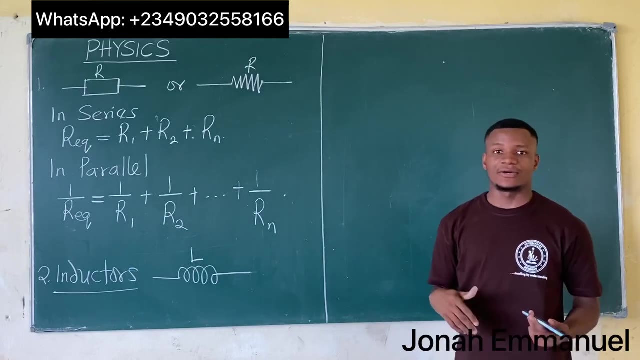 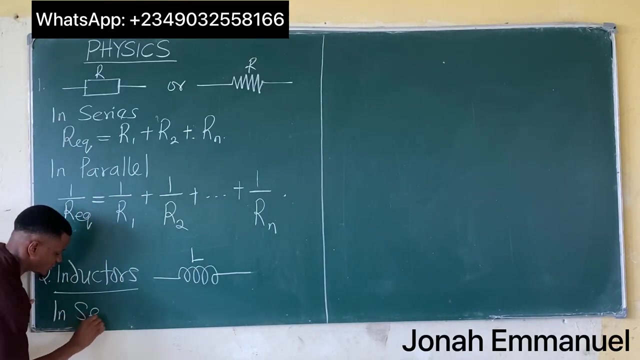 This. alright, This is the circuit symbol for an inductor. Usually, resistors are represented using R, Inductors are represented using L. Now the concept of adding resistors in series and parallel also works for inductors. That means for inductors in series, for inductors in series. 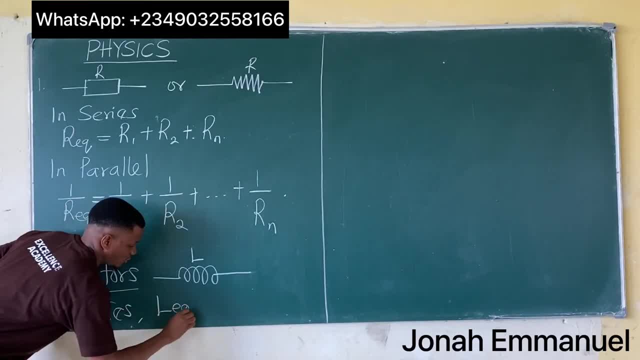 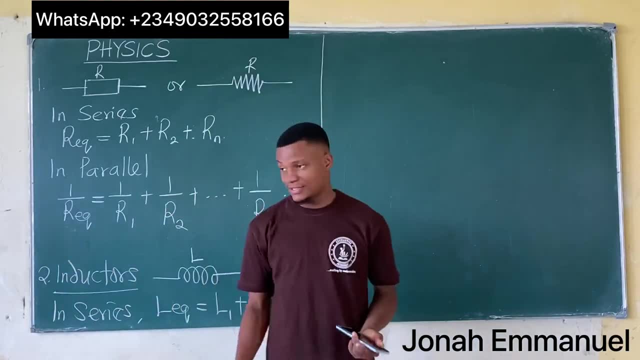 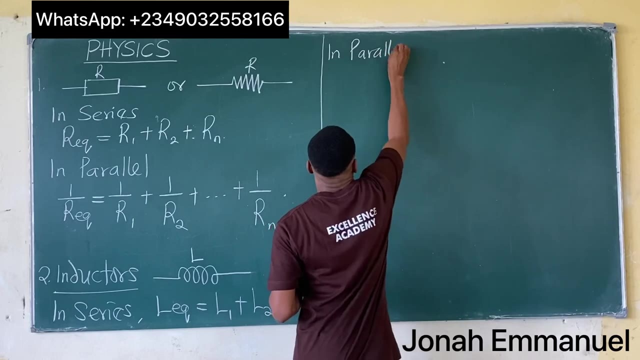 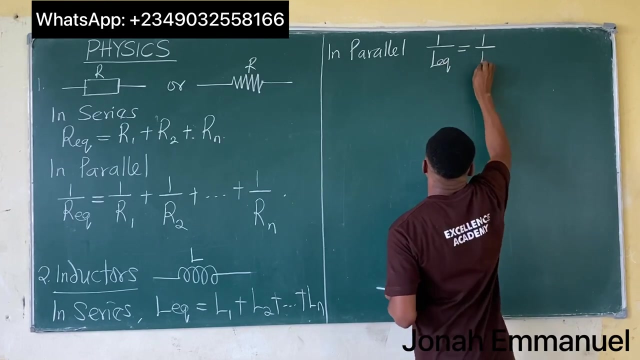 the equivalent inductor. let's say Leq is equal to L1 plus L2 plus, because we keep adding them up to the last one. So that is, inductors in series For parallel connection or in parallel. in parallel you have that, the inverse of the equivalent inductor. 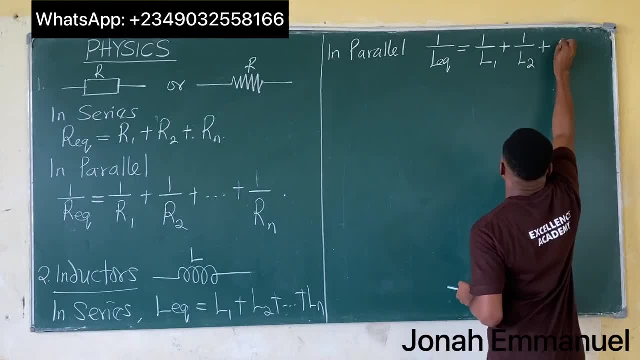 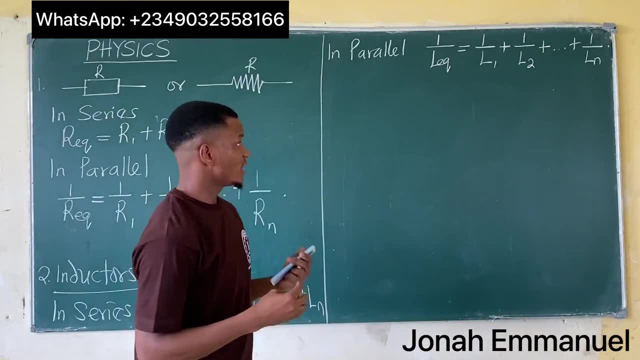 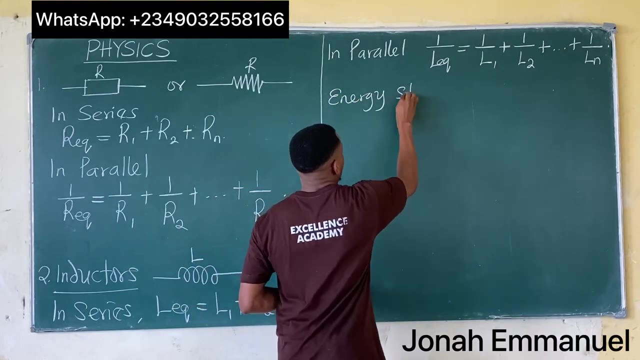 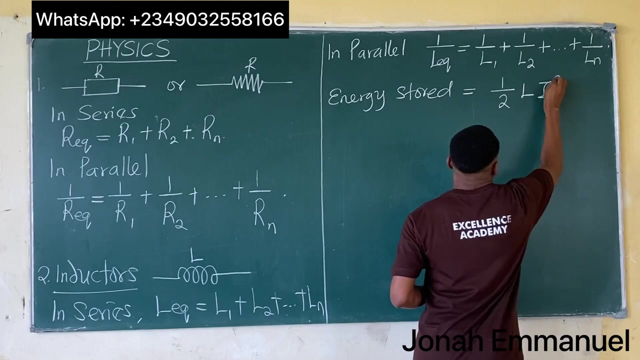 is equal to the inverse of each of them, just like this. Alright, so this is for inductors. A very important concept to notice is that the energy stored in an inductor, the energy stored in an inductor, is given by half Li squared. 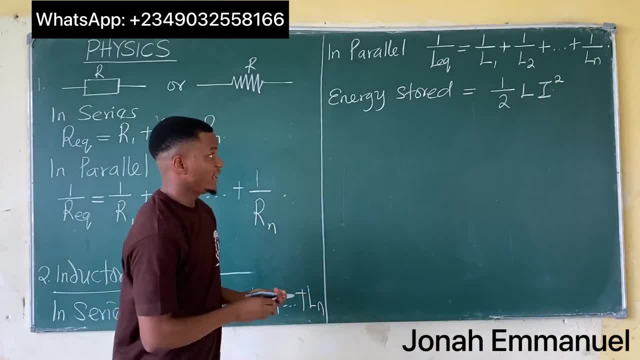 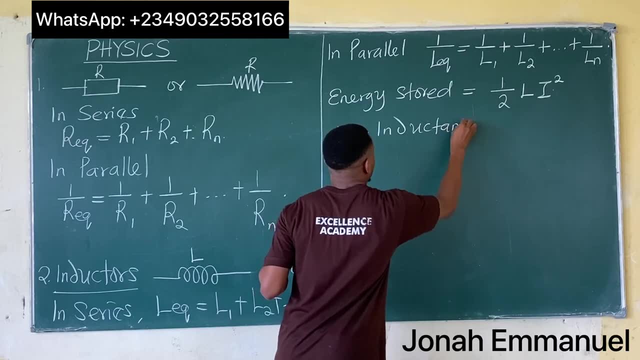 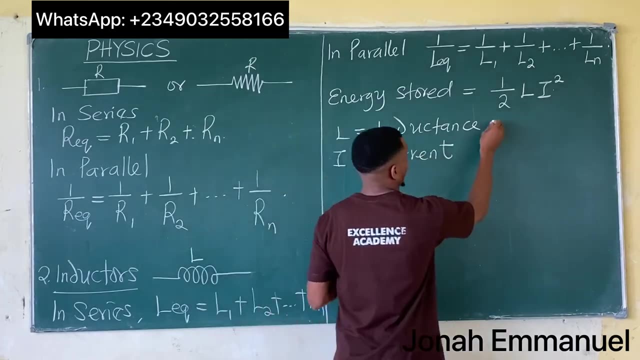 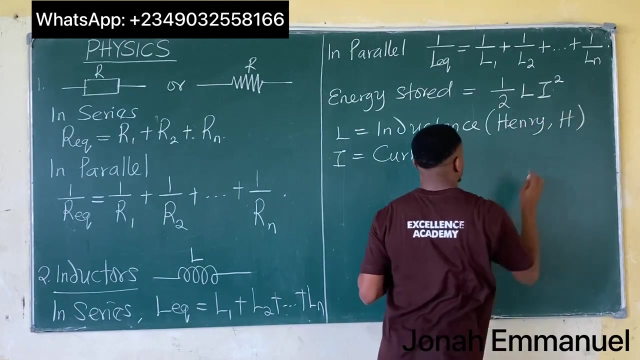 This is the energy stored in an inductor: L is inductance, L is inductance and I is current, Alright Inductance. inductance is measured in Henry H and then current, of course, in Ampere. 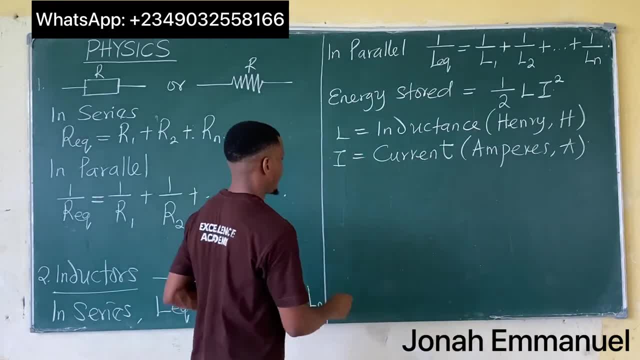 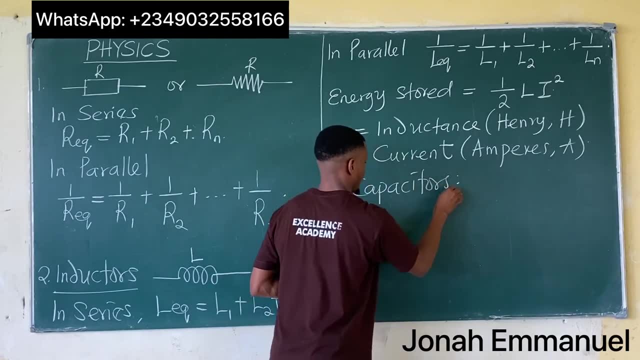 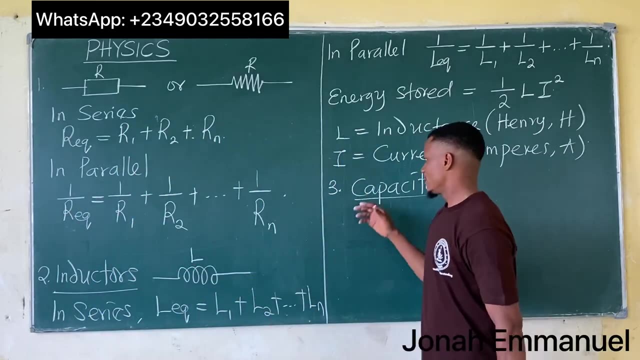 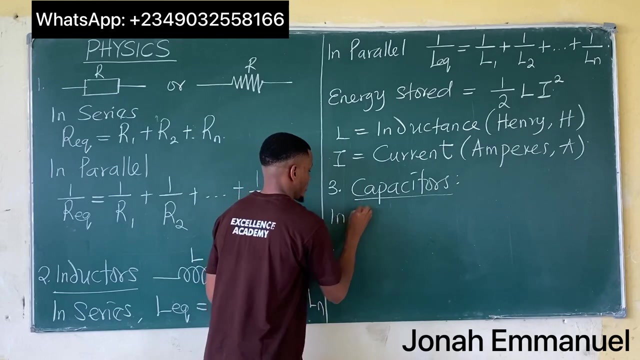 That's it, Alright. so finally, the third one. there is capacitors, Capacitors, Alright. so of course, inductors are used to store electrical energy. That's the function. Capacitor is used to store electrical charges. For a capacitor, the series connection in series. 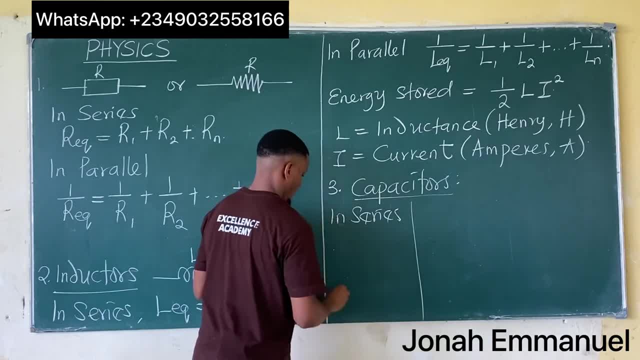 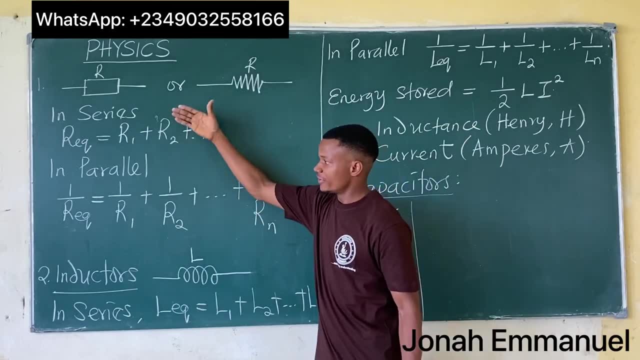 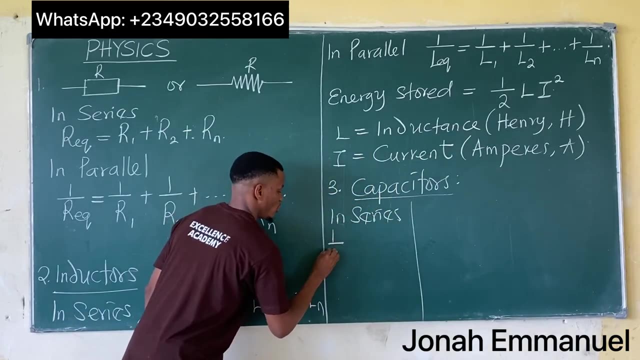 in series. we have that Now. the series concept of capacitor is the parallel concept of both resistor and inductor. So that means in series the capacitance, equivalent capacitance, equivalent capacitance is given by 1, all over cEq. 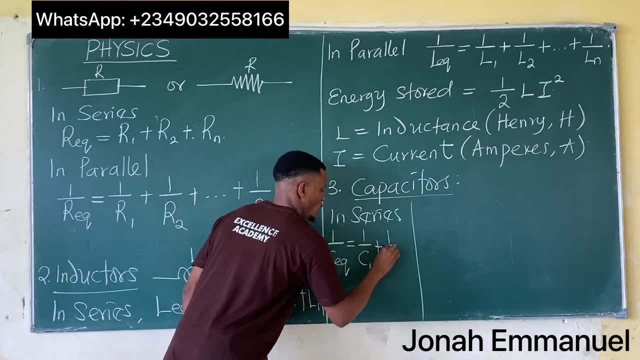 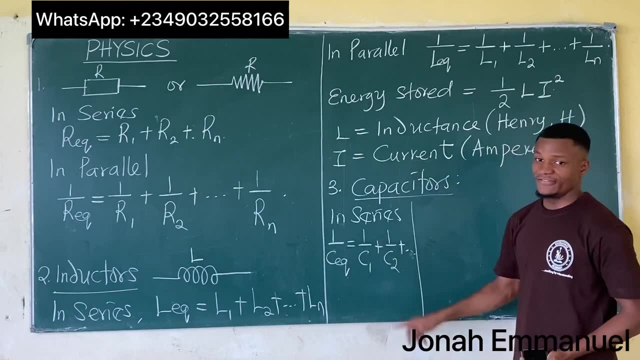 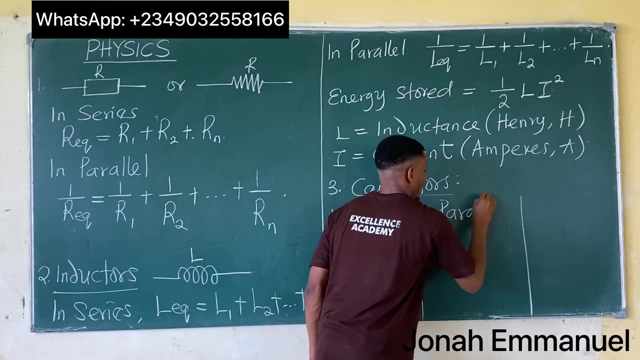 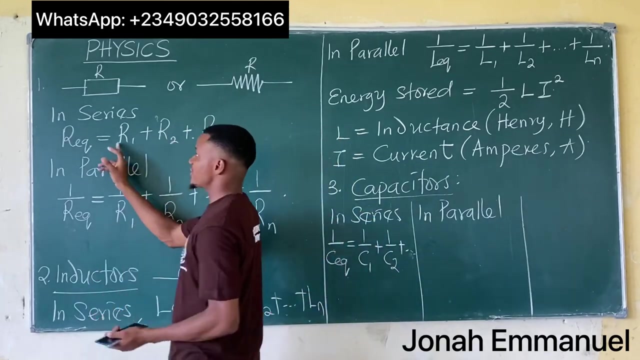 which is equal to 1 over c1 plus 1 over c2 plus continuous. So when it comes to capacitors, to get the equivalent, I will take the inverse of it Also in parallel, in parallel, for capacitor. the parallel concept of the capacitor is the series concept. 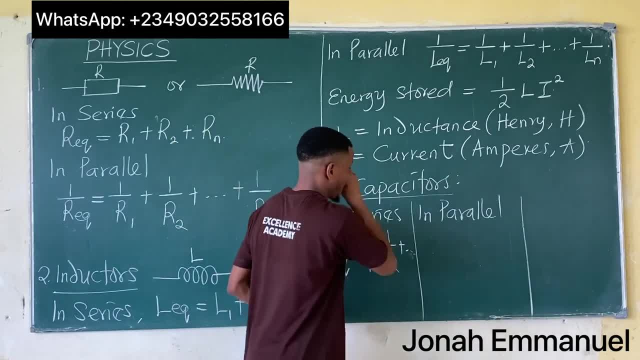 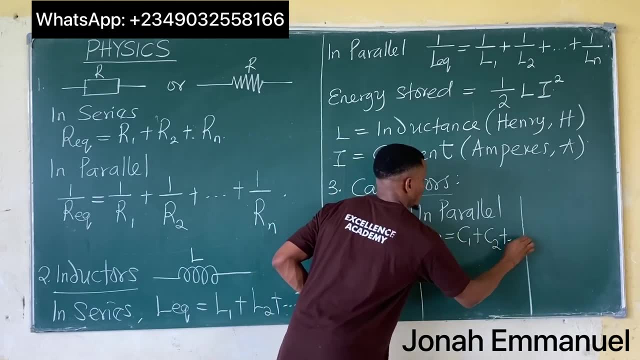 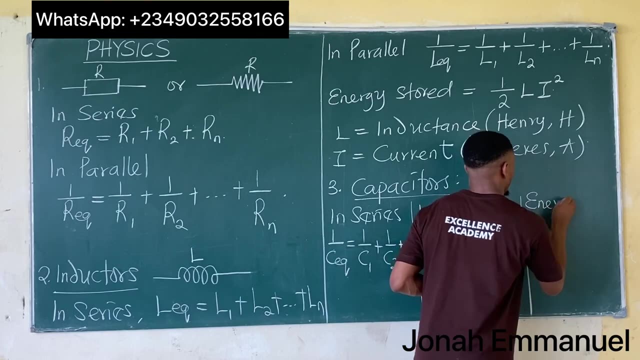 of both resistor and inductor. That means for parallel capacitor we have that the equivalent capacitance is equal to the sum of all that. Just like this. Just simply add them up straight. And then, finally, energy stored in a capacitor. Energy stored in a capacitor is E. 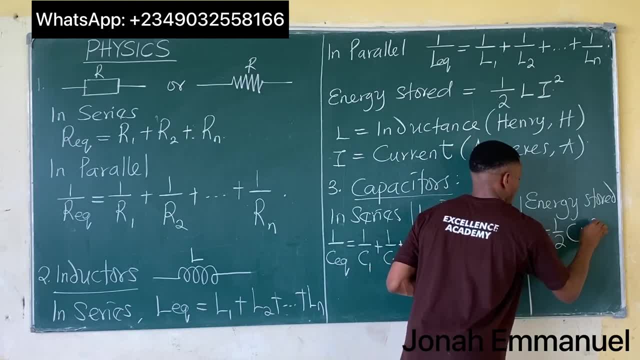 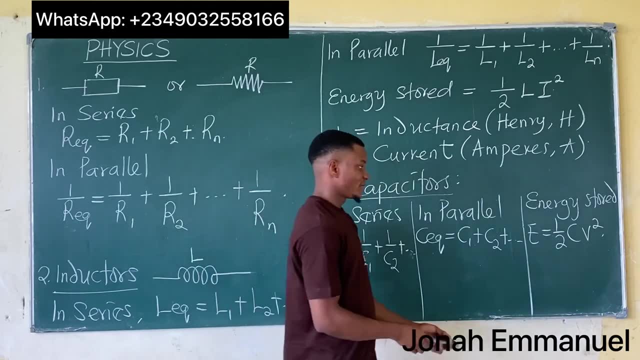 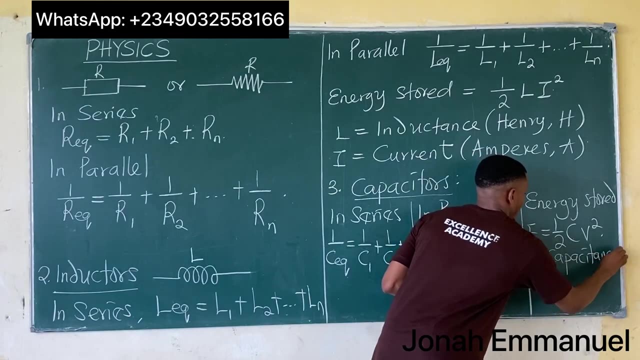 is equal to half cv squared, Please. this is the formula. This is the formula for the energy stored in a capacitor. All right, C represents capacitance, Capacitance is in farad And v is equal to pd. That's potential difference, of course, measured in volts. 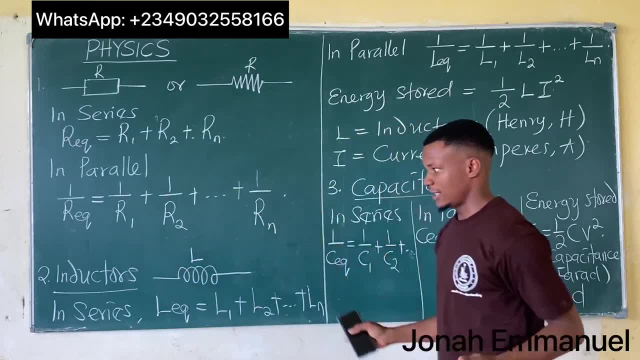 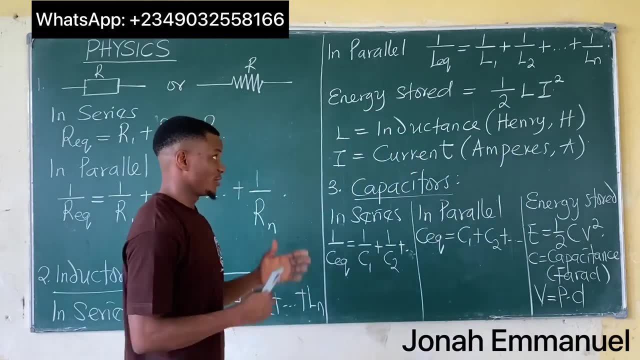 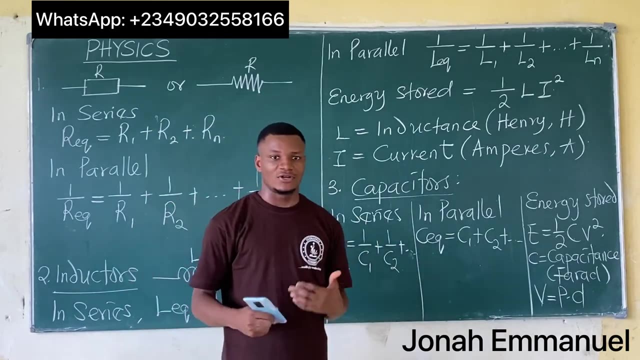 So these are like the formula we need to play around jump questions on Resistors, inductors and capacitors. So we need these formulas for both resistors, inductors and then capacitors. So we'll take some past questions. 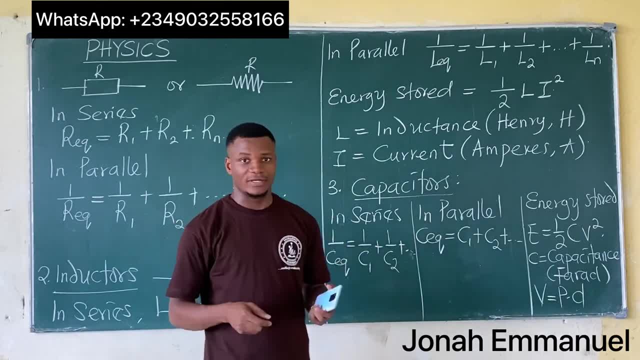 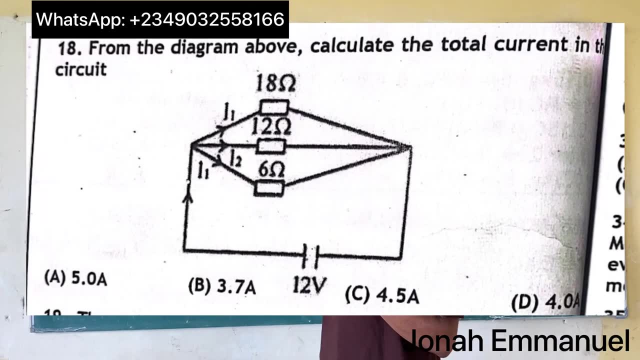 and revise them together and see how we solve them. Okay, So example one says from the diagram above: that's what you have there. calculate total current in the circuit. That's all. Calculate total current in the circuit, All right. 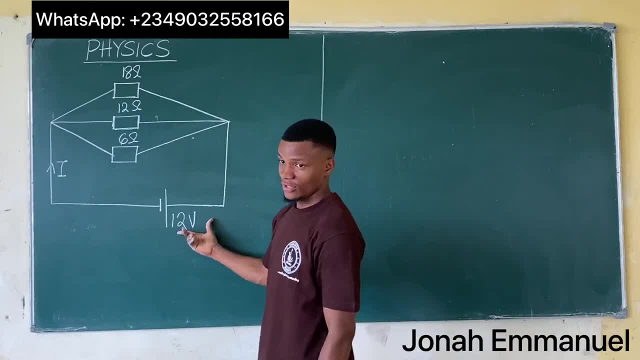 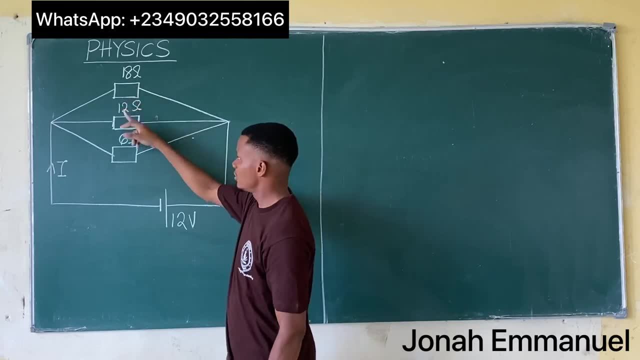 So we have these particular circuits here. So you have this voltage, 12 voltage, as a potential difference. You have 18 ohms, You have an 18-ohm resistor, 12-ohm resistor and 6-ohm resistor. 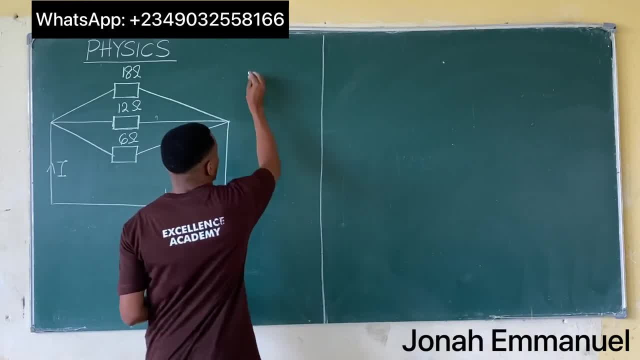 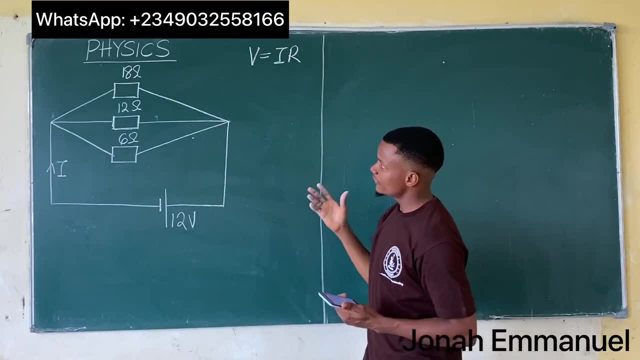 Now, from ohms law, we know that v is equal to an R, So we have this from ohms law. So if we are to solve this question, what exactly do we do? And we have to find the total current. Now we know that. 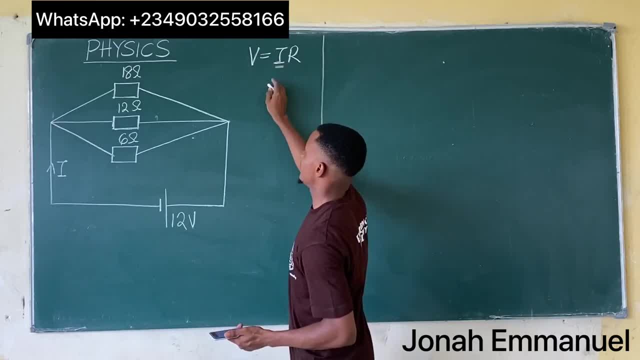 for total current or current as we had there, is equal to: if I should make current subject of the formula, I would divide that by resistance, divide that by resistance, these kinds of things. So current is equal to voltage, all over resistance. 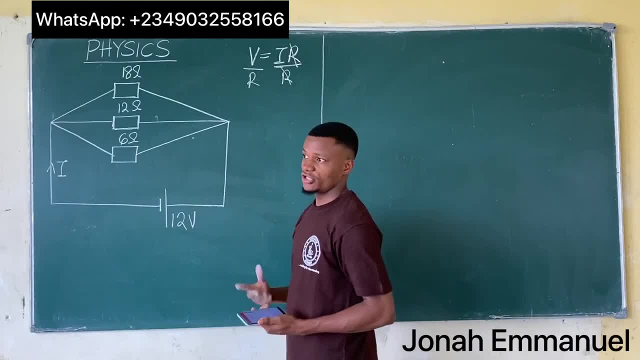 We already have voltage as 12.. But the issue here is that we have, instead of just one resistance, we have three resistances. So my first task would be: I would have to convert one of these three resistances to a particular resistance. 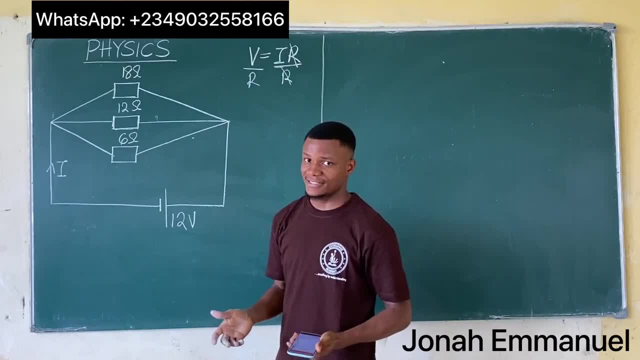 And that would be, I would have to find the equivalent resistance. That's case one. Now for this, if I look at this connection, of course, this one here is a parallel connection of resistance. This is a side-by-side connection. 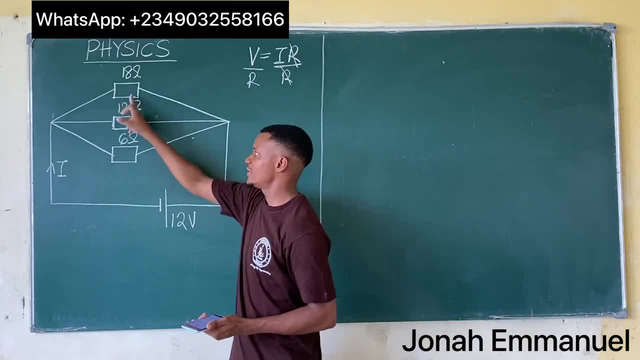 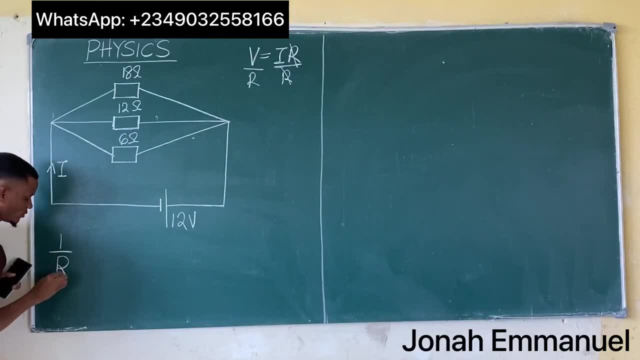 It becomes parallel connections. So find the equivalent of these three in terms of parallel connections. We said for resistance that the equivalent one all over R-E-Q, or let's say one over R here, is equal to one all over. I'm taking this as R-1, 18,. 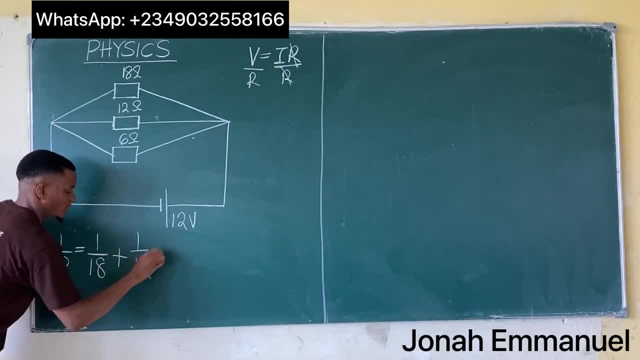 plus I would take this as R-2,, one over 12,. plus I would take this as R-3,, one over 6.. If I take LCM here, LCM of 18,, 12, and 6,- 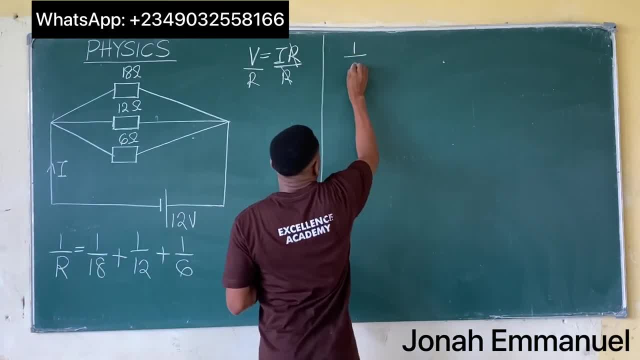 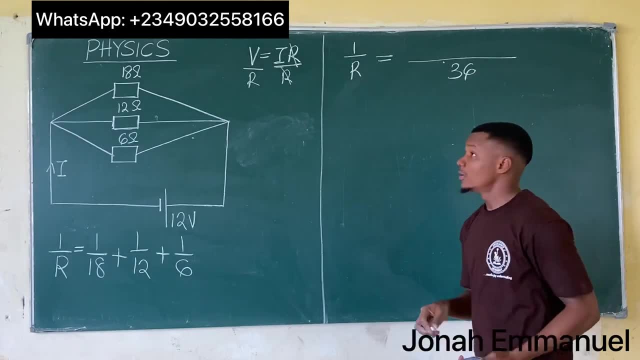 I would have that. one all over R is equal to my LCM, becomes 36.. Alright, so my LCM is 36.. 36 divided by 18 is equal to 2.. 2 times 1 is 2,. 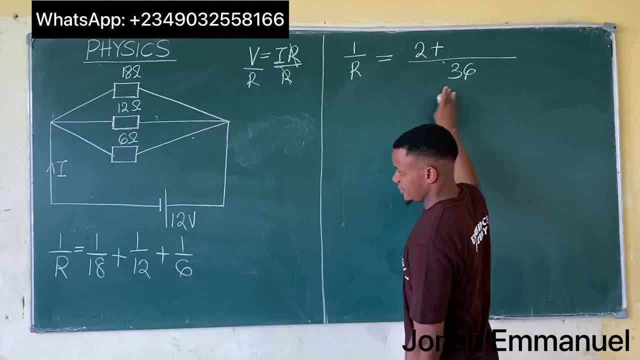 so I have 2,. plus 36 over 12 is 3.. 3 times 1 is 3,, so I have 3, plus 36 over 6 is 6, times 1 is 6,, so I have 6 there. 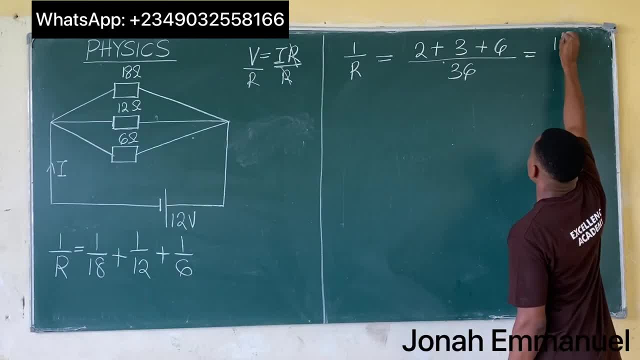 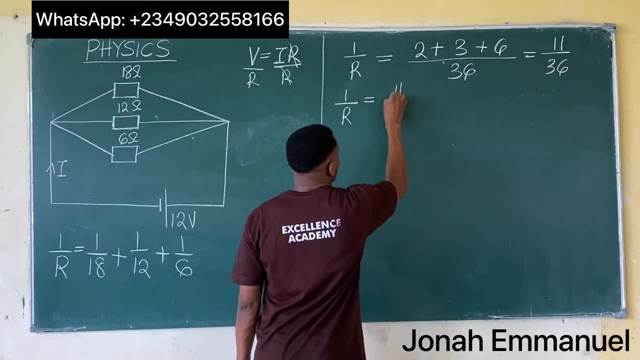 This is equal to this, and this is 5, plus 6,. that means 11 over 36.. So one all over the equivalent resistance is equal to 11 over 36.. That means from here to get R. 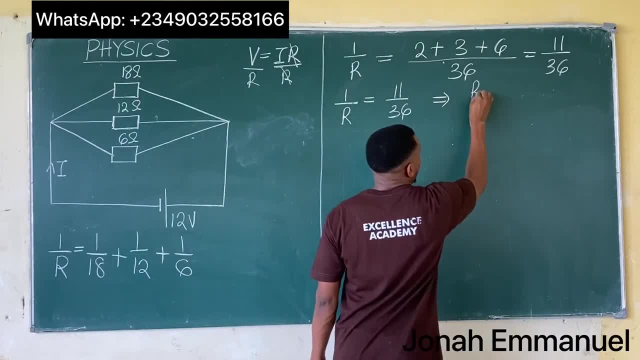 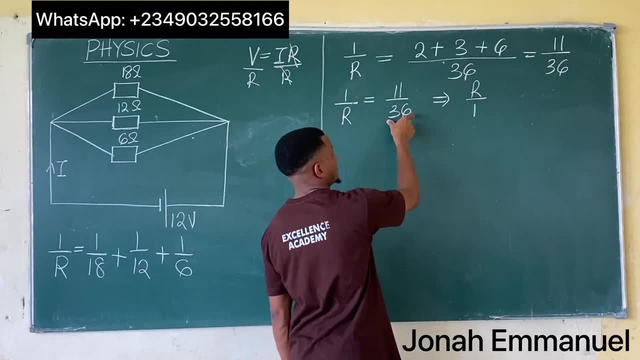 I'll simply invert it. If I invert it, it becomes R over 1,. I'll switch this 2,. it becomes R over 1, also switch this one here. it becomes 36 over 11, so I have it equal to. 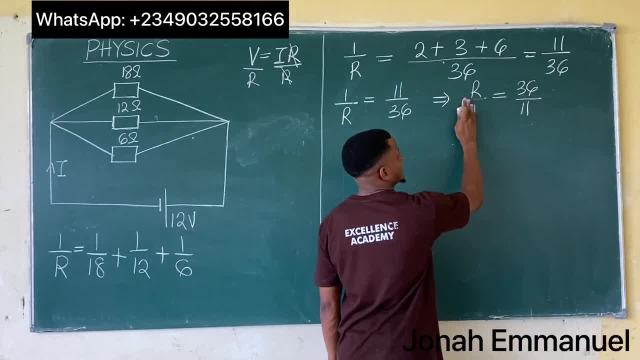 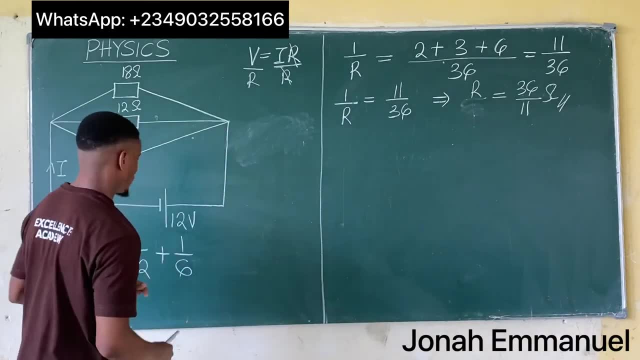 36 over 11.. That means the equivalent resistance R is equal to 36 over 11 volts. So with this, now I've gotten the value of R. My next step is to find. I Also recall, so also recall that we said: 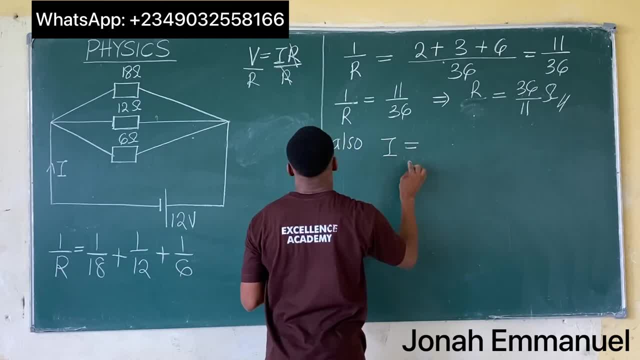 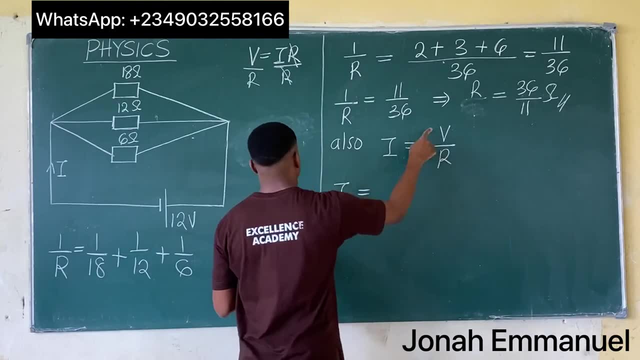 from Ohm's law, the current I is equal to what there V all over R. So let's get this done. That means I is equal to V. V is 12,. that becomes 12, divided by R. 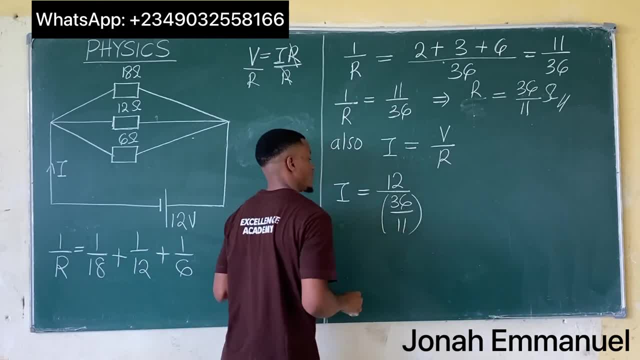 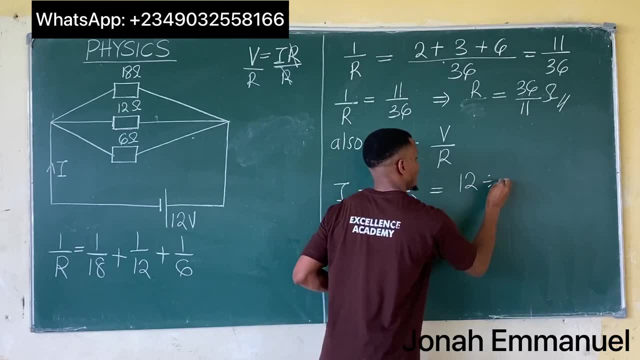 R is 36 all over 11.. So we have this, But I work this out: This is equal to 12, divided by 36, over 11.. So solve this: The current I is equal to. 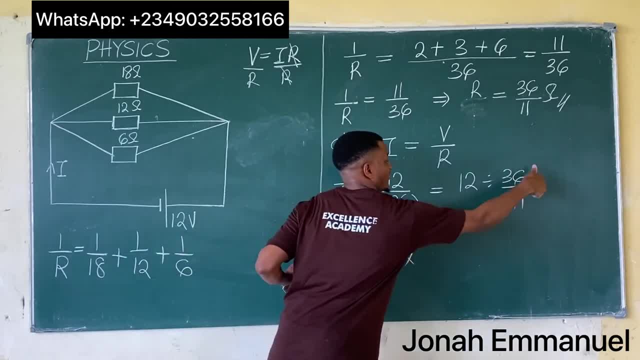 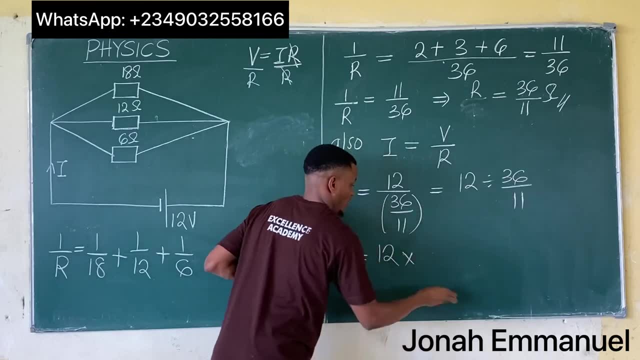 12 times. we'll invert this right. change here to times. This is how you solve this change here to times. invert this. So this one goes up, this comes down, becomes 11 over 36.. This is now equal to. 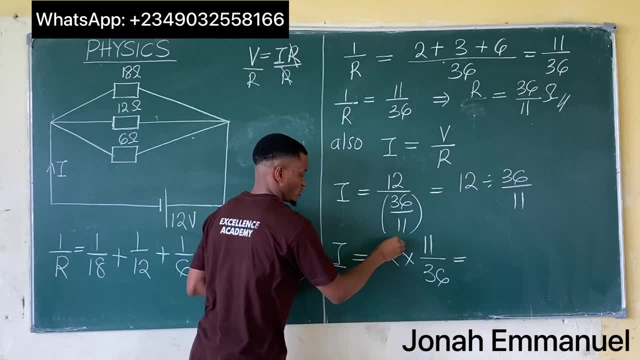 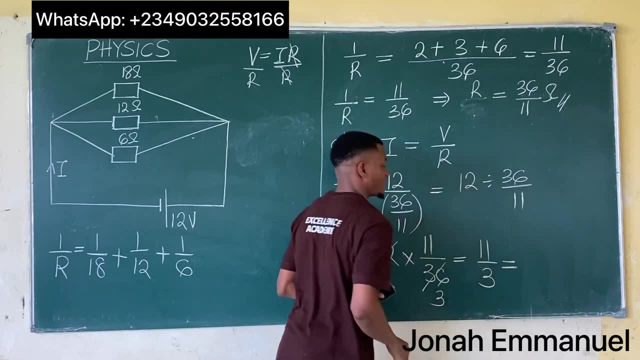 12 here 1,, 12 here 3.. So this now gives you 11 over 3.. If I convert 11 over 3, it becomes 36, R, if I convert 11 over 3,. 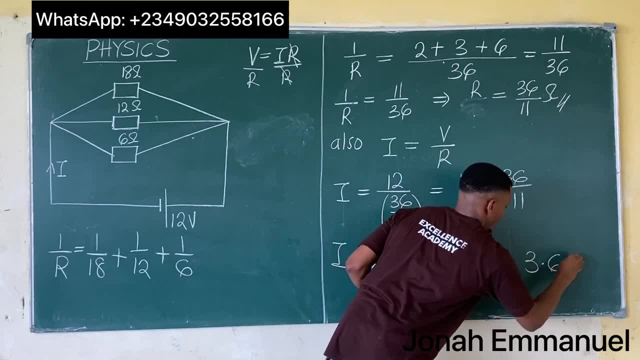 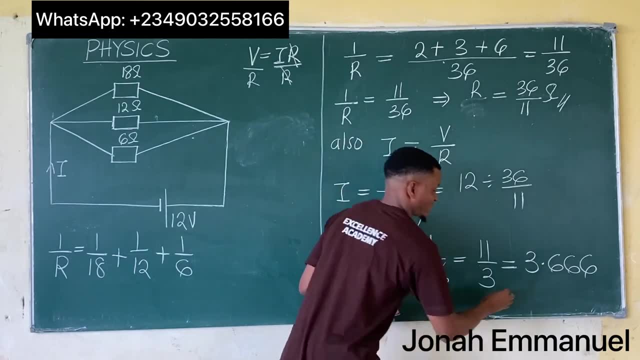 to decimal, it gives me 3.666, and 86. If I convert this to linear, to 1 decimal place, in 1 decimal place, this becomes 3 points. So 1 decimal place gives you. 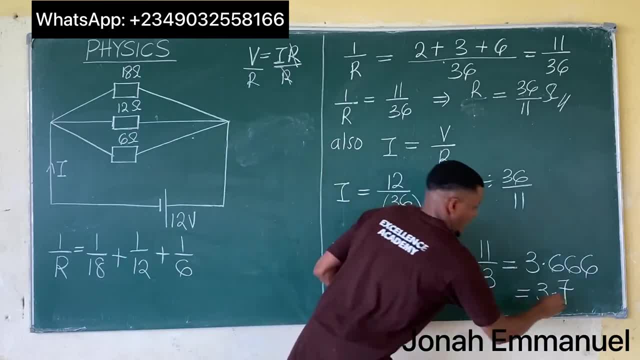 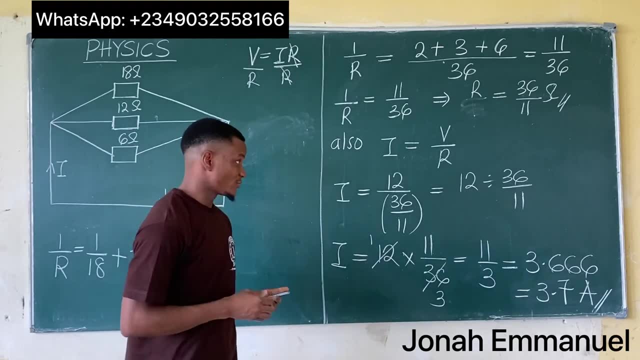 7.. Of course, I'm completely correct. that becomes ampere. So my answer becomes 3.7, ampere, And that's option B. So this is how you solve this question. Alright, let's consider. 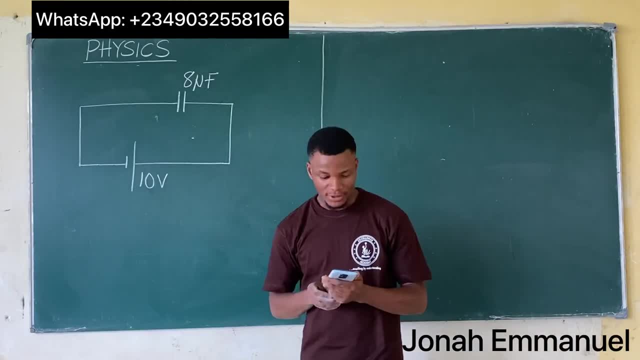 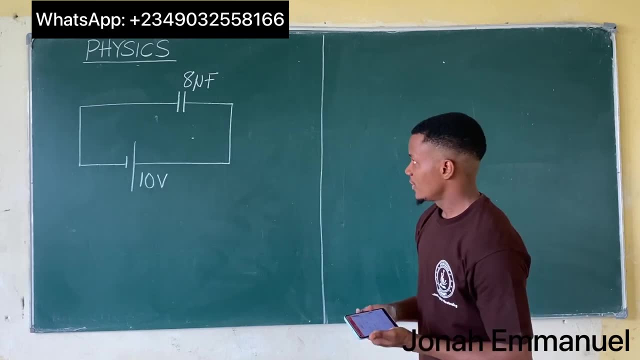 a second example. It says from the diagram above: calculate the energy stored in the capacitor. That's this, Alright, so we have this diagram. again, we have to find the energy stored in the capacitor. Now what we do is this: 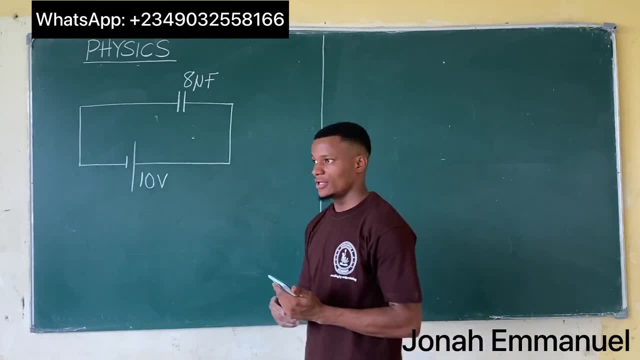 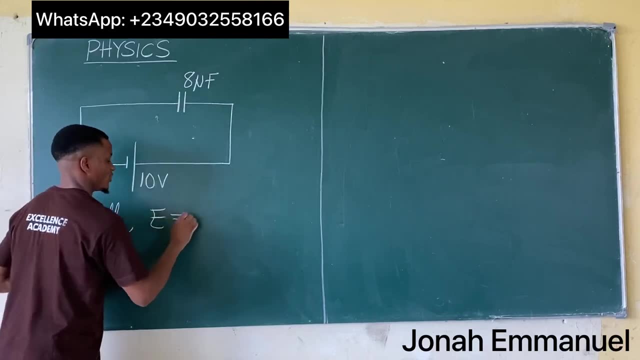 so recall. recall that we said: energy stored in the capacitor E is equal to half C V squared. That is our pickup parameter. Now what we have to do is we have to calculate pickup parameter. 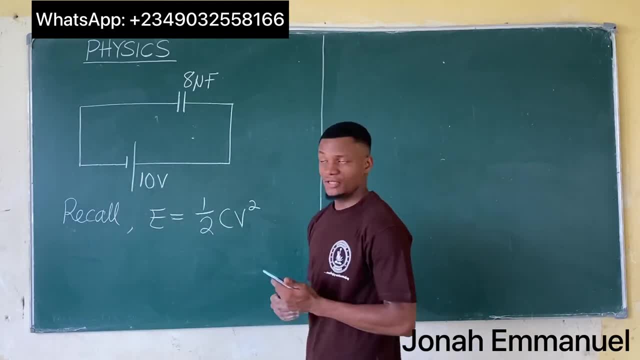 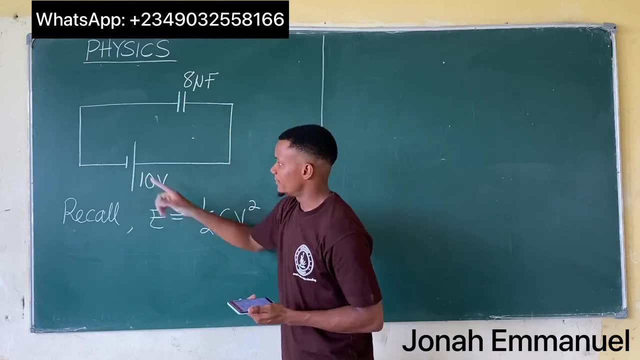 And before I proceed, before I proceed, it's important to note that the second symbol for a capacitor and a key or a battery or a cell, alright, they are almost alike, But the difference is this. 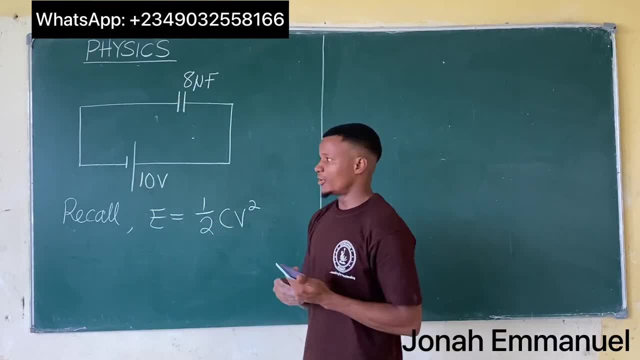 for a capacitor. observe that the lengths are equal for this. look at this: the lengths are equal for a capacitor, While for a cell- alright, potential difference like this. you have that. one, two, three. 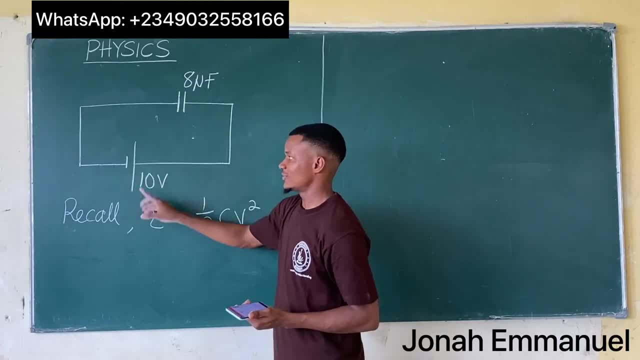 one. one end is longer than the other. So that's the difference between these two. Alright, These two, where the two ends like this, or the two lines are equal, is called a capacitor. That's a capacitor. second symbol: 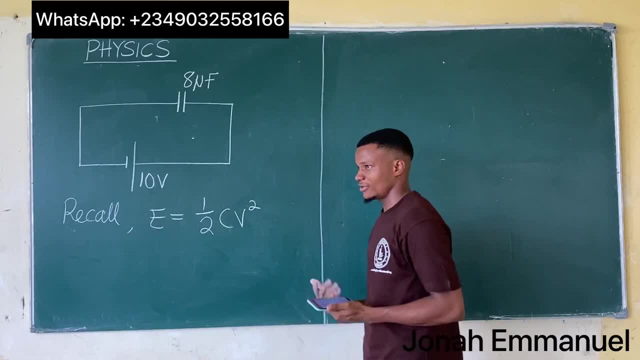 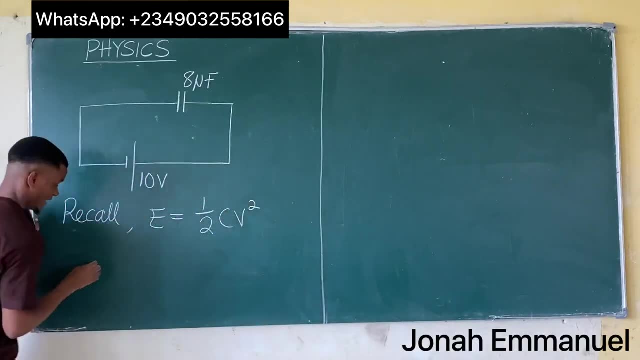 But for this one here, where one is longer than the other, that becomes your cell or your battery or your potential difference, whichever one. Alright with this. now let's solve this question From here. I'm giving that the capacitance. 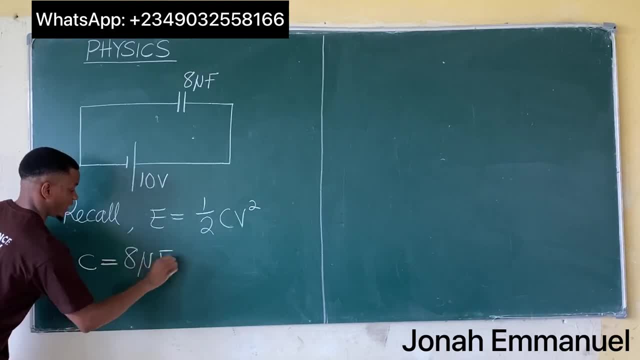 from here is eight micro farad, That's equal to eight times micro. is ten to the power minus six. That becomes ten to the power minus six farad. So please always do your conversion Alright, Micro. 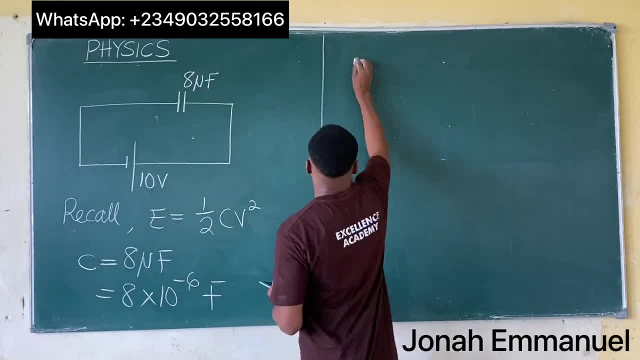 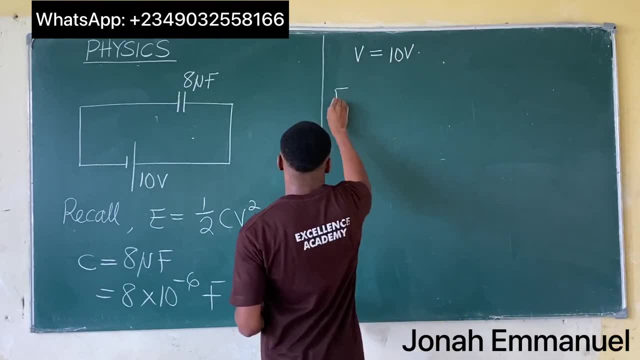 is ten to the power minus six. Next up, I have that the potential difference V is equal to ten volts. Alright, so let's solve this. So hence it means that the energy E is equal to. 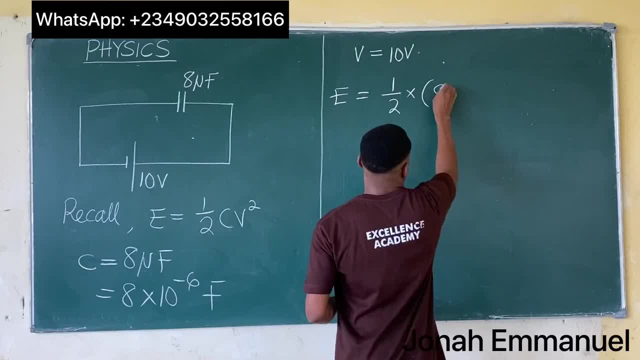 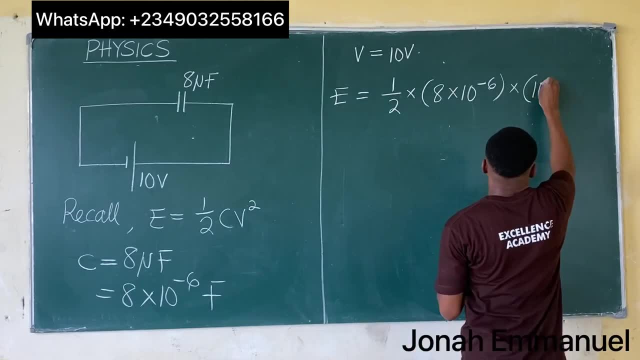 half times C. So this- I'm using the combative value- ten to the power- minus six times V squared, V is ten. That means it's ten squared. If I work this out, this is E. 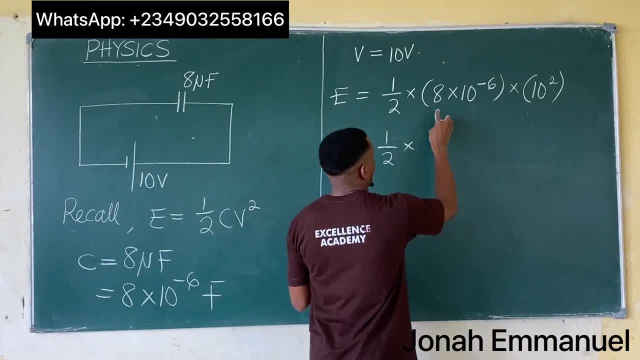 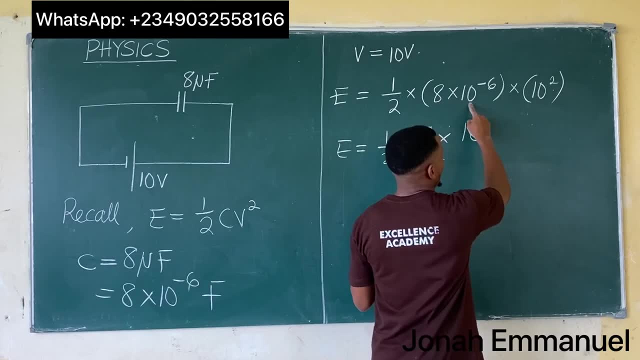 being equal to half times um eight times. what condition is it in That becomes ten. We said from indices: when two um same um base, when two numbers are multiplying, when they are the same. 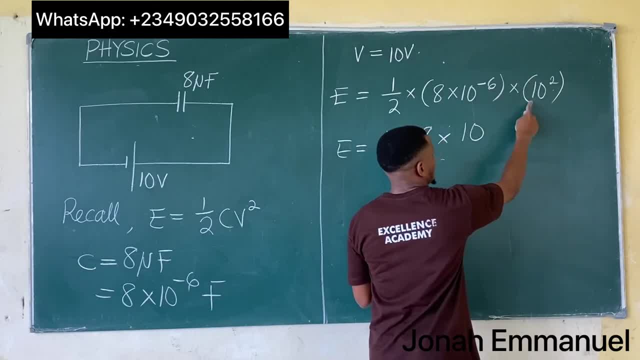 we said: simply add their parts. The same number that we're multiplying ten and ten. add their parts. The part here is minus six. The part here is plus two Minus six. plus two gives you. 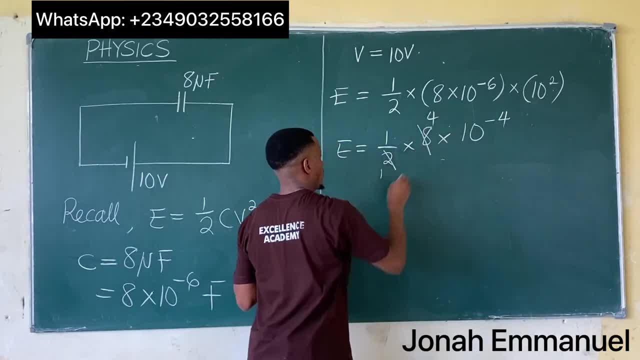 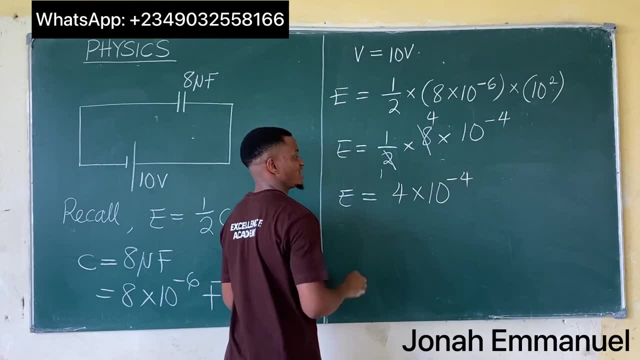 minus four. Okay, also two here one, two here four. So E the energy is equal to four times ten, to the power minus four Energy. that's the answer. Uh, which option is that? 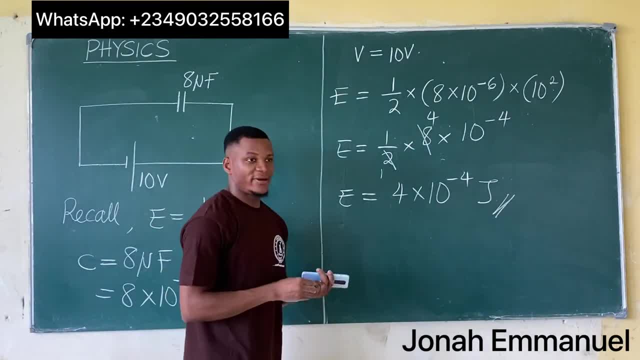 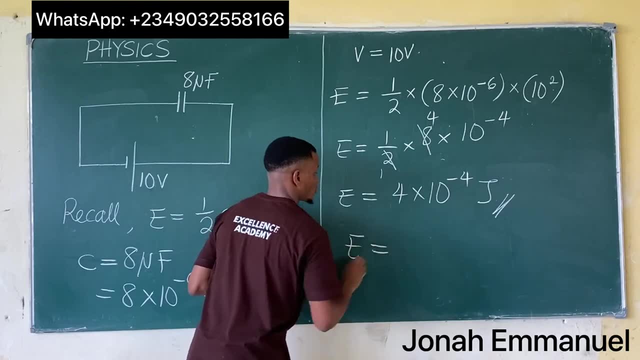 Okay, options are not given, But anyways, this is your answer. So, depending on if you have to give this E, either as standard form or as decimal, As decimal E will be equal to. so we said four. 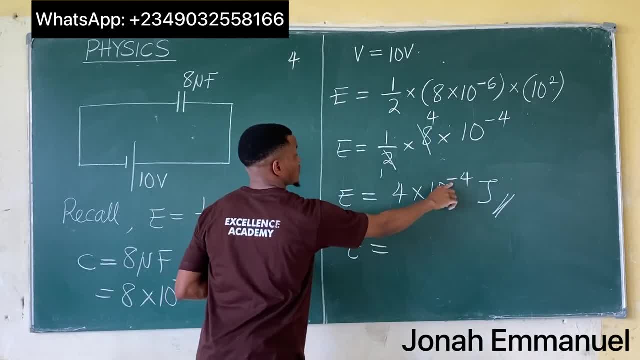 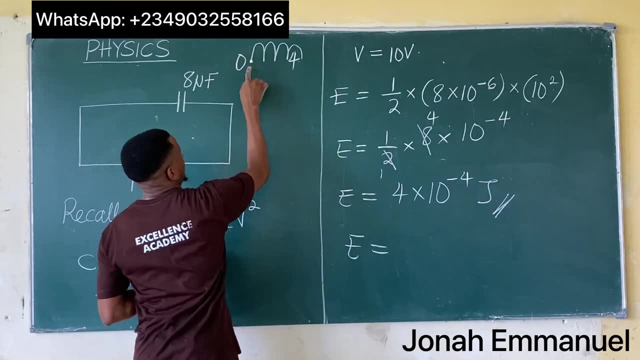 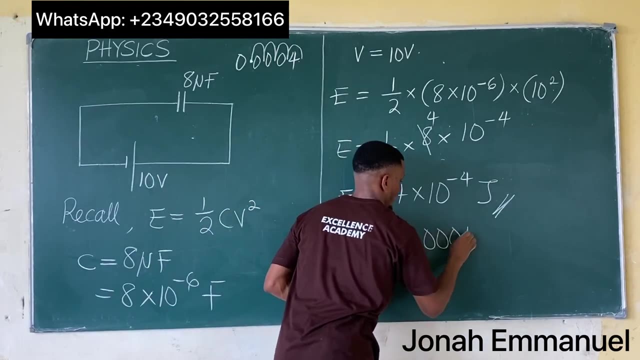 we said times equal to minus four. From here go back four times one, two, three, four. So here it's: minus zero points, zero, zero, zero, zero point, zero, zero zero. 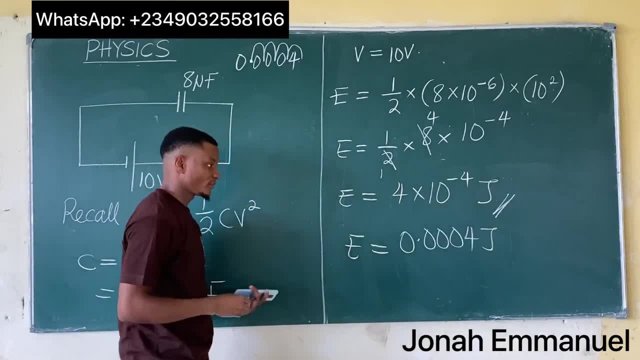 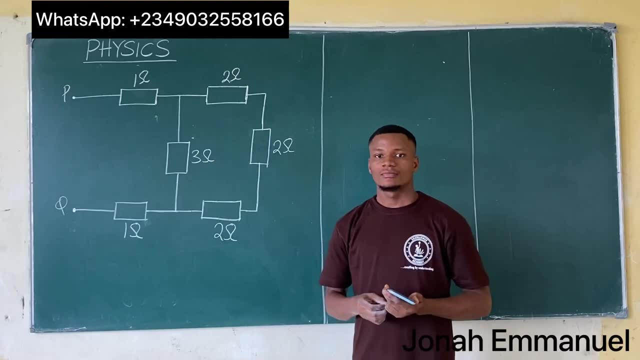 four joules. Uh, these two are the same thing, Right. Alright, so this is how you solve this question. Alright, let's try another example. This question says the total resistance measured at PQ. 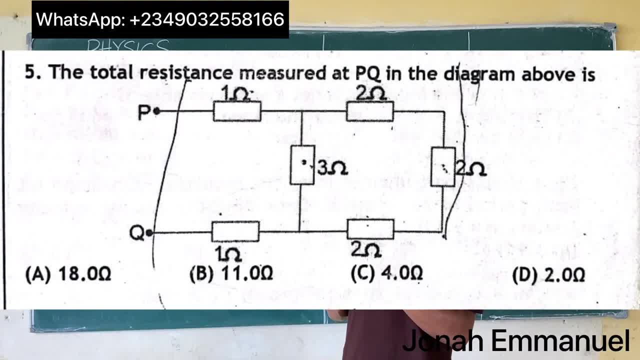 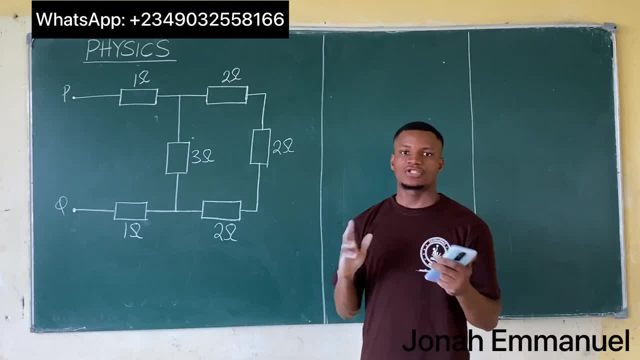 in the diagram above is alright, so here's my diagram. please, Now let me, let me. let me. now let me stress something here: When it comes to measuring total resistance or capacitance, 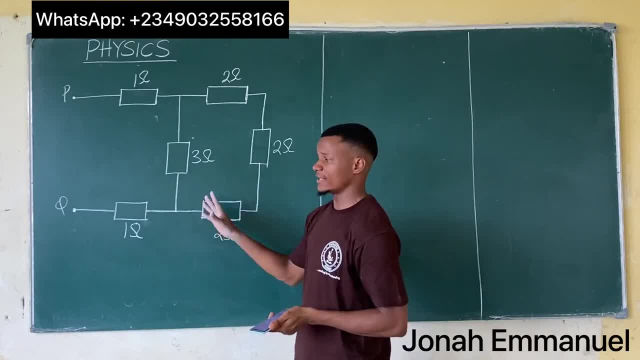 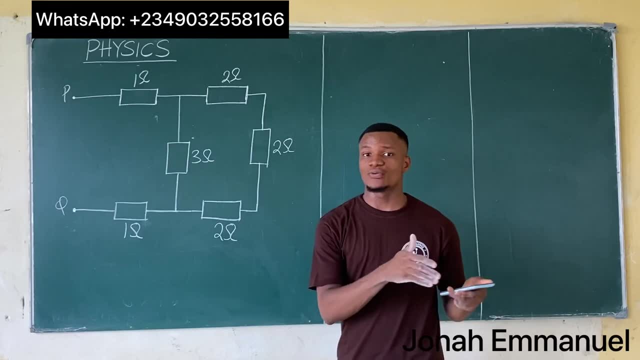 or inductance in figures. that looks like this. now, what you do is this: always start from the closed end and measure up till the open end. Please don't forget that's the pattern of solving: Start from the closed end. 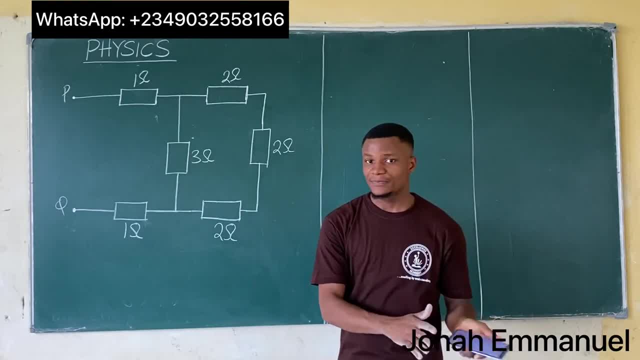 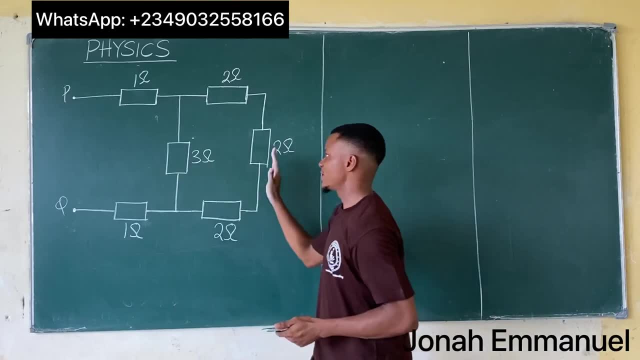 and measure up till you get to the open end. Now what do I mean In this figure here? here's my closed end. here looks open. That means I'll start from this point and I'll keep solving until 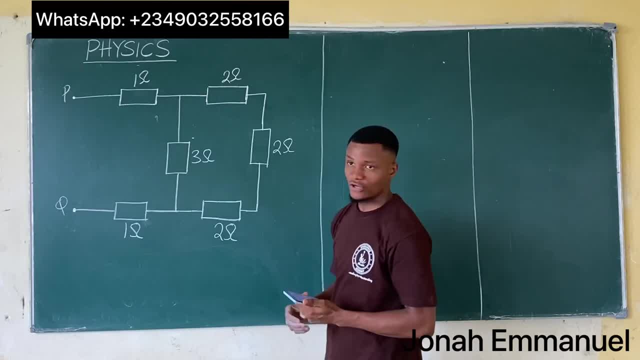 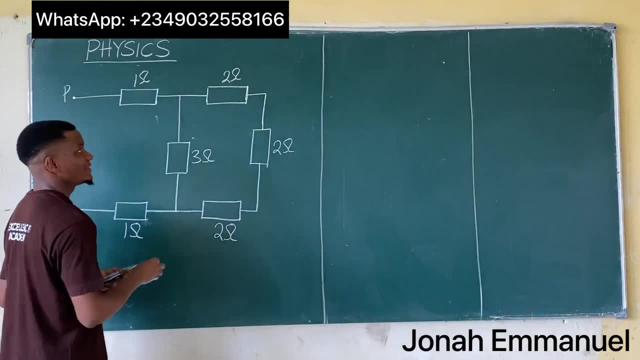 I get to the open end. That's how we solve problems of this nature. So where do I start from This one here? My first task is this: observe that one, two, three are in series. Why? 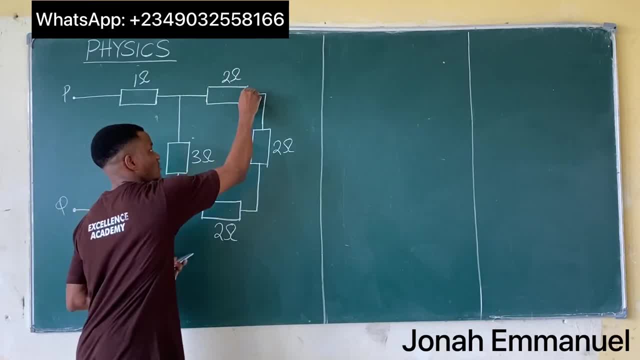 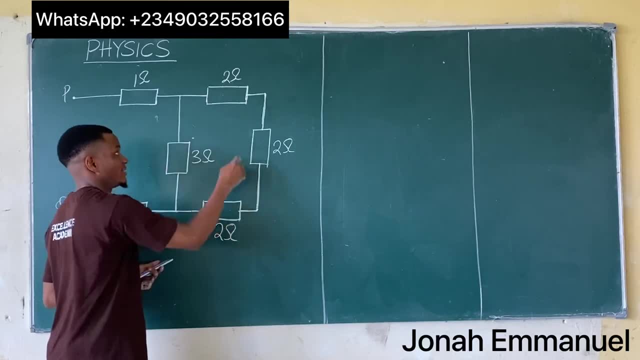 Because we said in series we have an end to end connection, Because this one here, this end, is connected to this end, this end connected to this end. So hence, one, two, three. So let's first of all, 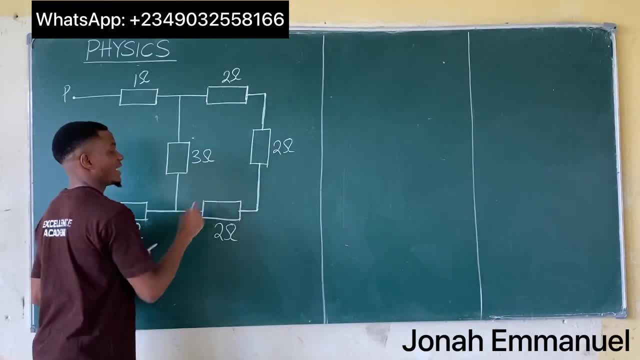 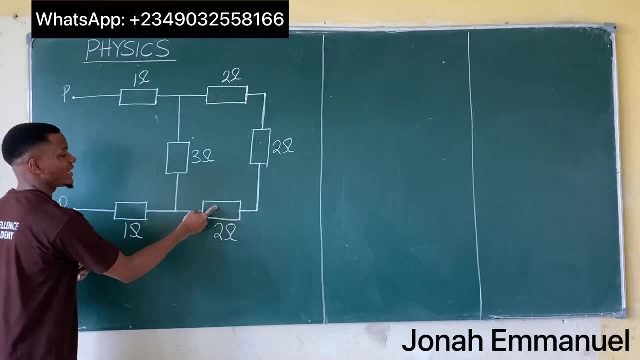 let's figure them, or should we? Okay, let's just proceed. So one, two, three are in series. So I'll now resolve this one here, this one here, this one here in series. Now you may want to ask: 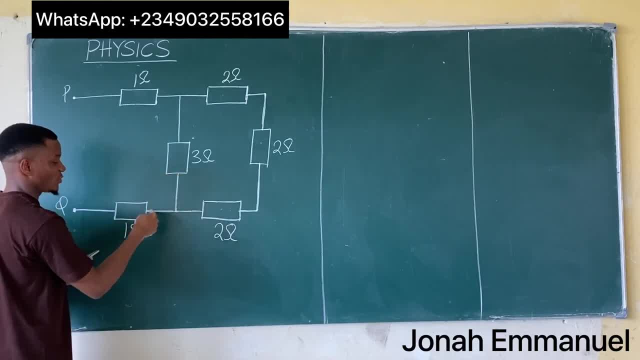 why did I involve this one? Well, this one is kind of complex in the sense that this one, the connection from here, branches to here and here. So in series, let's call this, let's call this R1,. 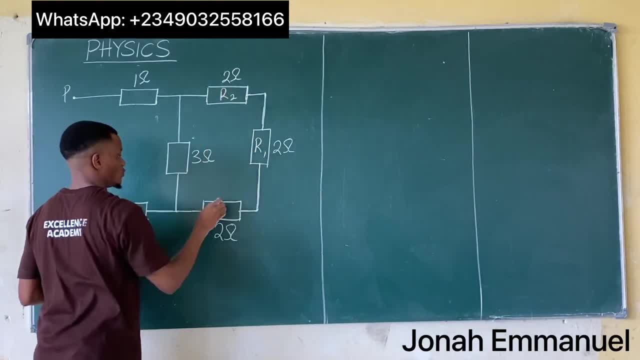 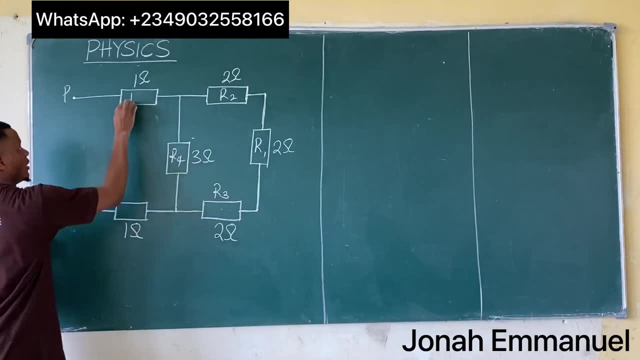 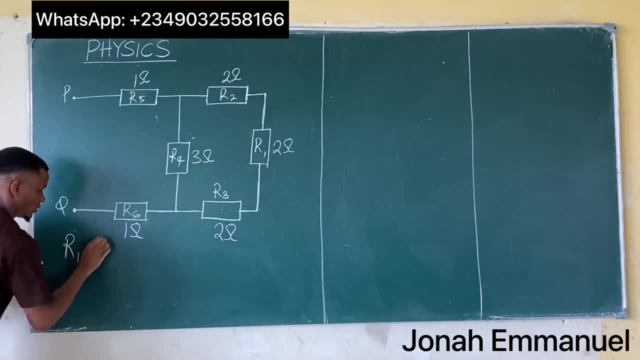 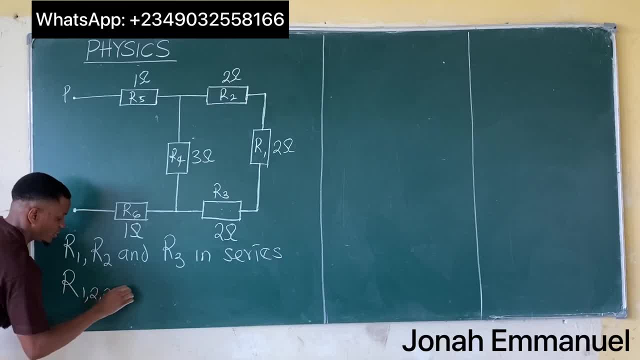 2, 3,, so I'll call it R1,. 2, 3, is equal to. since it's a series connection, I'll just add them straight. that becomes R1, plus R2, plus. 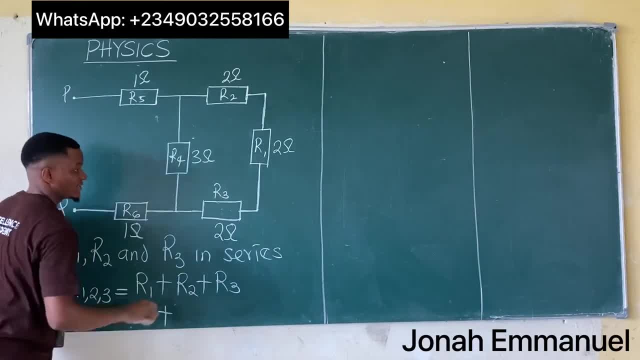 R3.. And that's equal to R1, is 2, plus R2, is 2, R3, is 2.. So this gives you 2,, 4,, 6,, 6 ohm. 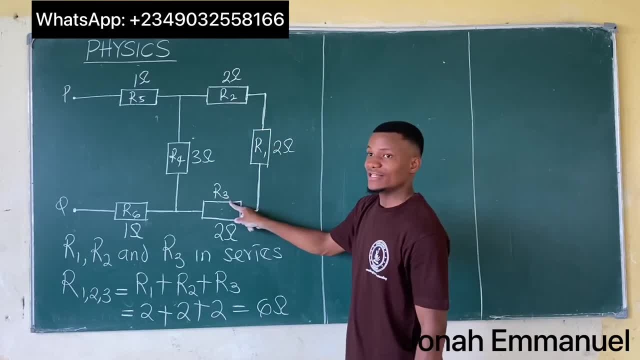 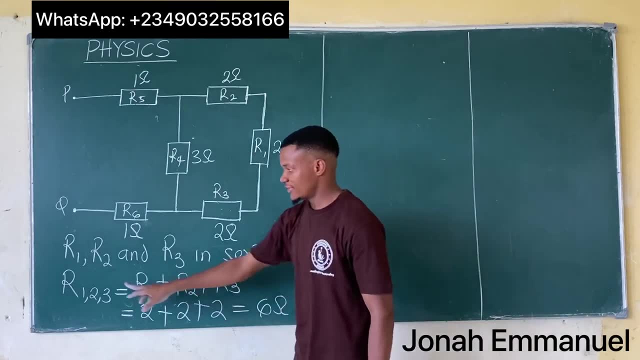 Now, this 6 ohm is the connection for just 1,, 2, 3.. We are still here to resolve 4,, 5, and 6.. So if I'm counting this 6 ohm- 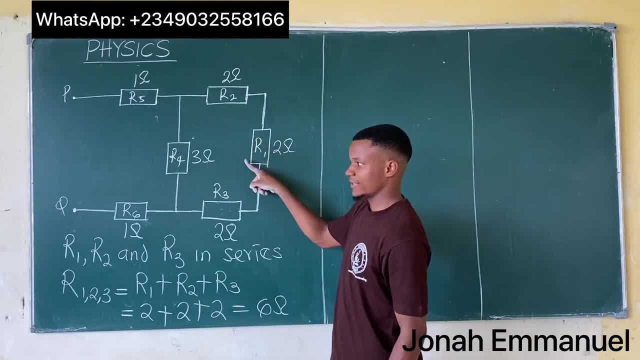 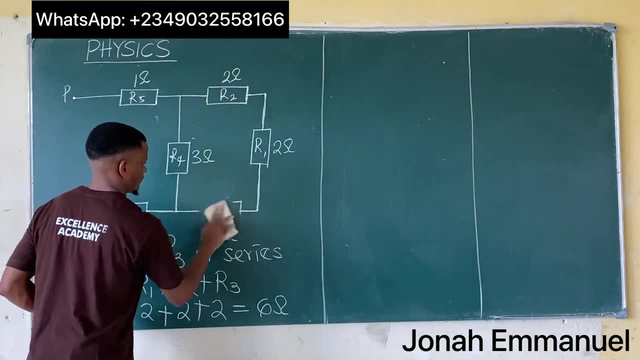 as being the resistance of 1,, 2,, 3, where will this 6 ohm appear? It will appear at this point here, Alright, So I'll tell you where I did this. So when I connect. 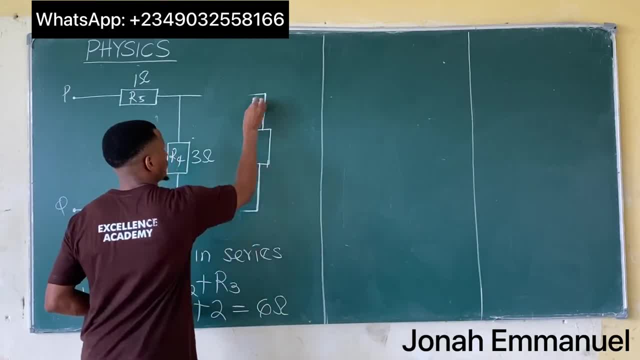 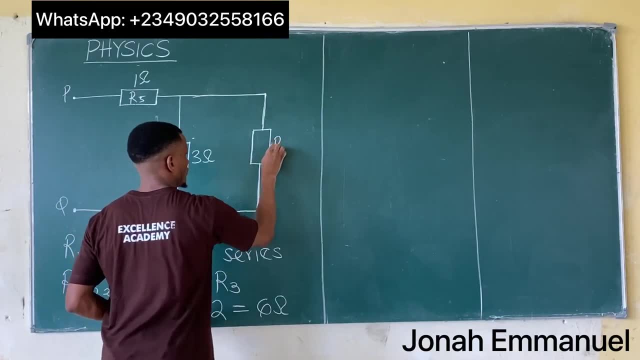 1,. when I connect 1,, 2,, 3,, we have had R1,, R2,, R3,, R4,, R5,, R6,, R7,, R8,, R9,, R10,, R11,. R12,, R13,, R14,, R15,, R16,, R17,, R18,, R19,, R20,, R21,, R22,, R24,, R25,, R26,, R27,, R28,, R29,. R30,, R31,, R32,, R33,, R34,, R35,, R36,, R37,, R38,, R39,, R40,, R41,, R42,, R43,, R44,, R45, R46,. R47,, R48,, R49,, R50,, R51,, R52,, R53,, R54,, R55,, R56,, R57,, R58,, R59,, R60,, R61,, R62,, R62,. R63,, R64,, R65,, R67,, R68,, R69,, R70,, R61,, R62,, R62,, R63,, R64,, R64,, R65,, R67,, R68,, R69,. R70,, R71,, R72,, R72,, R73,, R74,, R74,, R75,, R78,, R78,, R79,, R79,, R80,, R80,, R81,, R82,, R82,. R83,, R83,, R84, R84,, R85,, R86,, R87, R86, R87, R87, R86,, R98,, R89,, R11,, R10,, R12, R12, R13,. R14,, R15,, R16,, R17,, R18,, R19,, R20,, R22,, R23,, R24,, R25,, R26,, R27,, R26,, R27,, R28,, R29,. 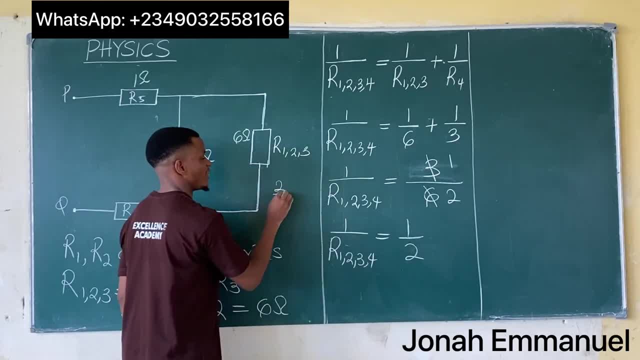 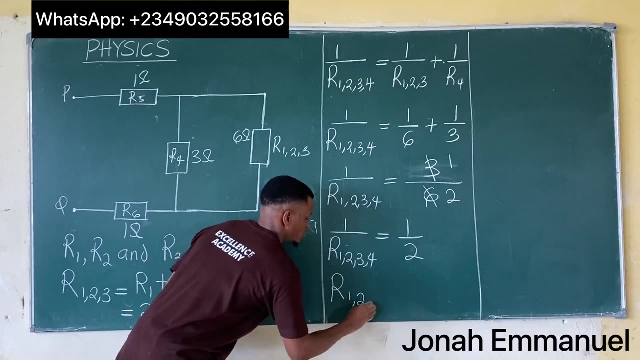 R30,, R31,, R32, R33, is two, a over one is a. so therefore, anything over one is that thing, so hence, in this case, i'll have that this all over one will become itself. so r one, two, three, four will be equal to. 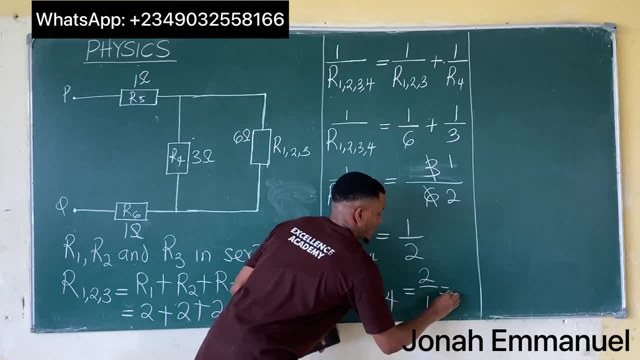 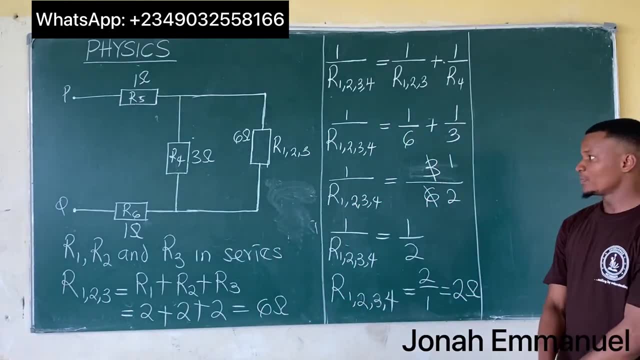 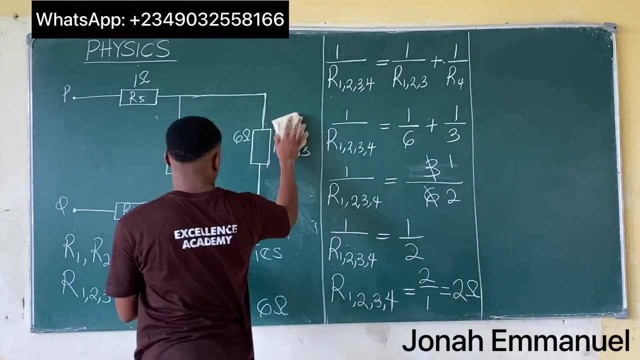 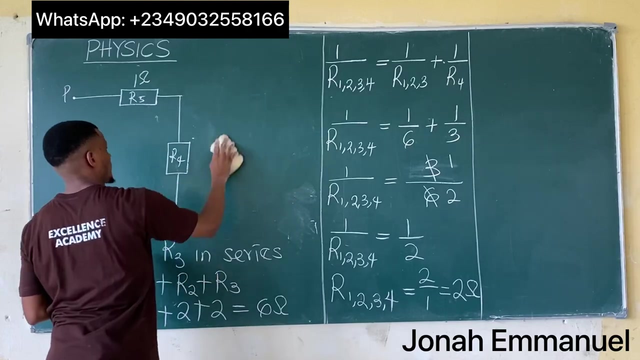 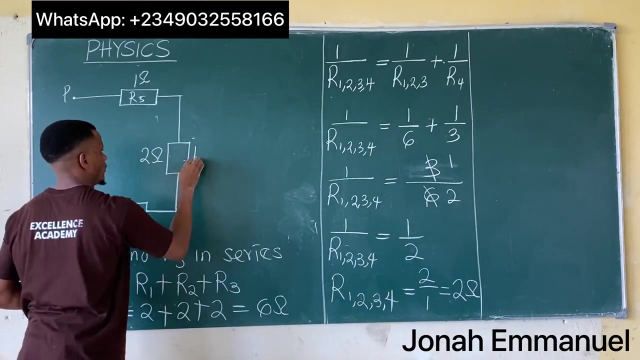 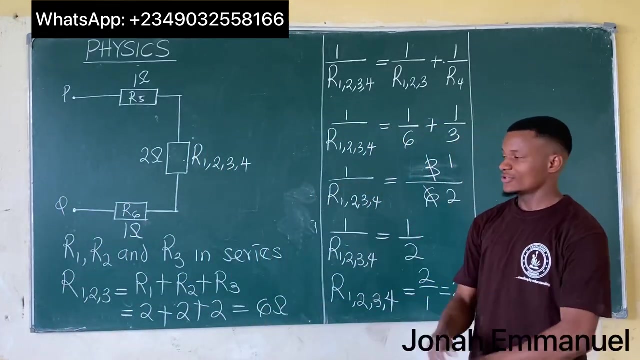 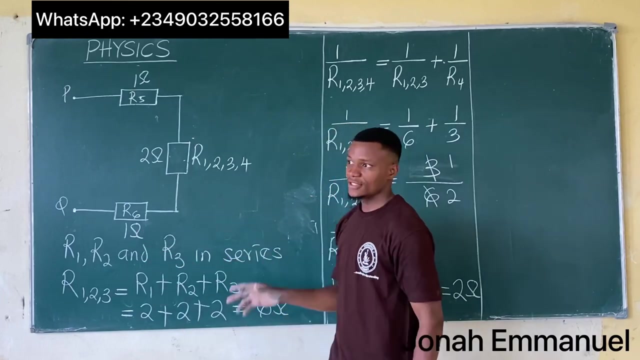 in fact this becomes two all over one. that's equal to two, of course, in both. so, of course, the value of r, one, two, three, four, this value now will now come this way. all right, so see how we've now reduced our settings from that light component up to this smaller component. 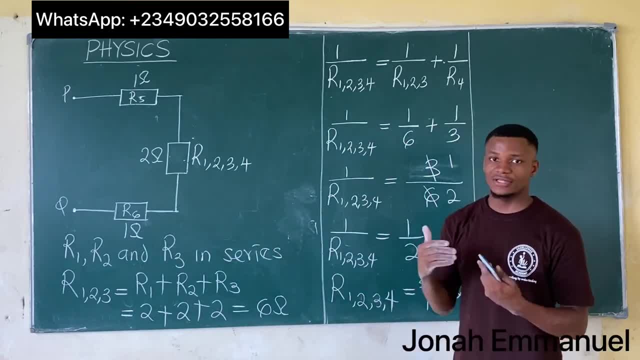 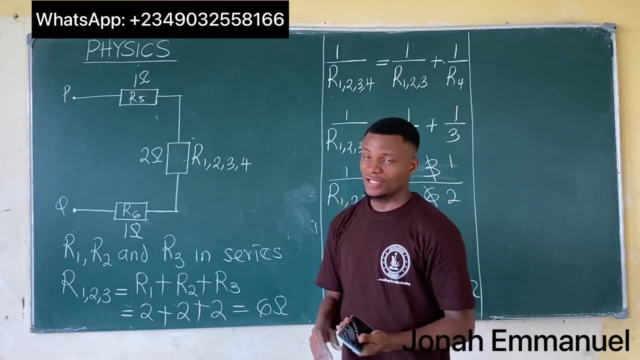 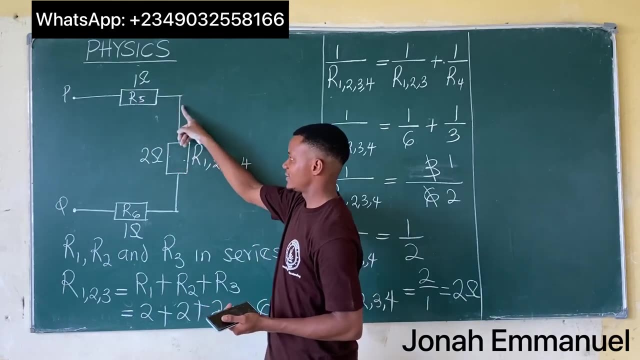 this technique is called the circuit reduction technique. all right, it's used to reduce complex connections to same flowers, as you can see. now, finally, to get my final answer- i can see that i'm fine is connected in series, so i want three, four, also connected in series to rs6. 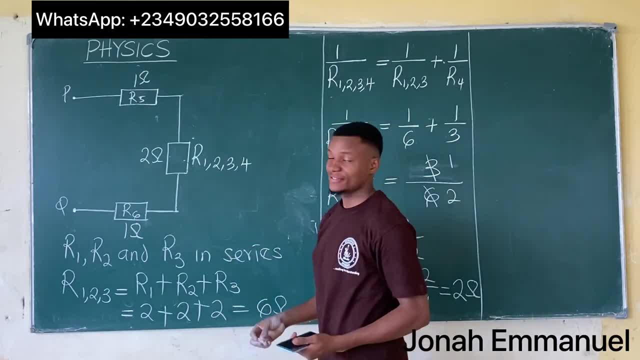 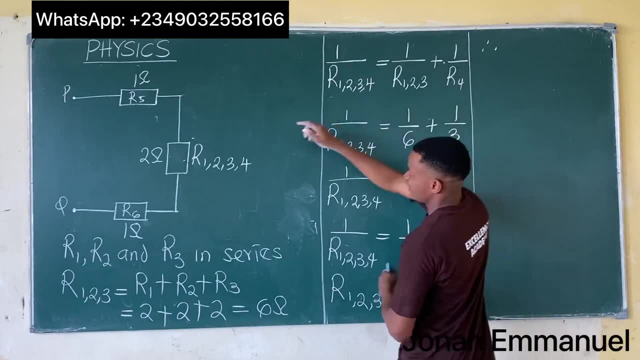 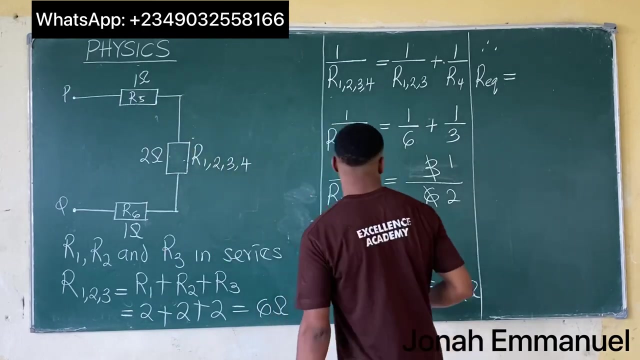 so hence i will now get my final equivalent. so therefore, therefore, the equivalent resistance um. this is series connection. so for series connection i'll have that r? eq is equal to decide for series. just some divided right, just some advantage becomes this value plus this value, plus this value, so it becomes r one, two, three, four. 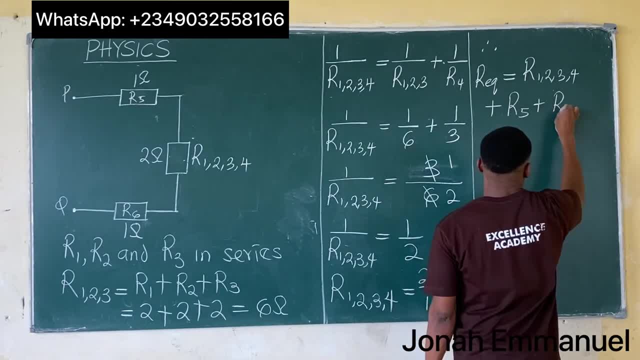 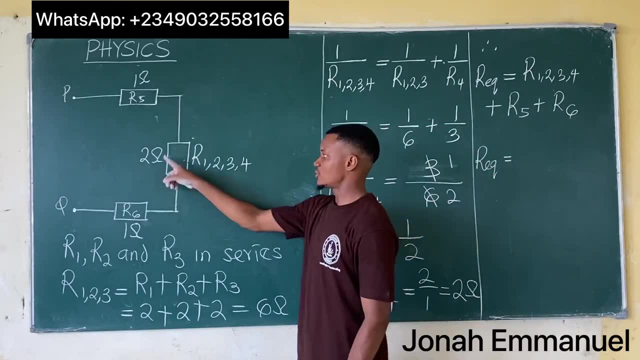 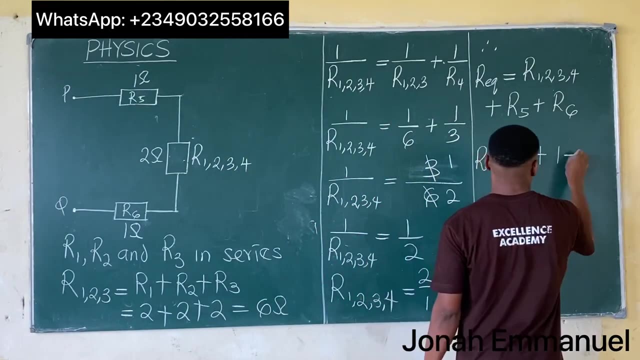 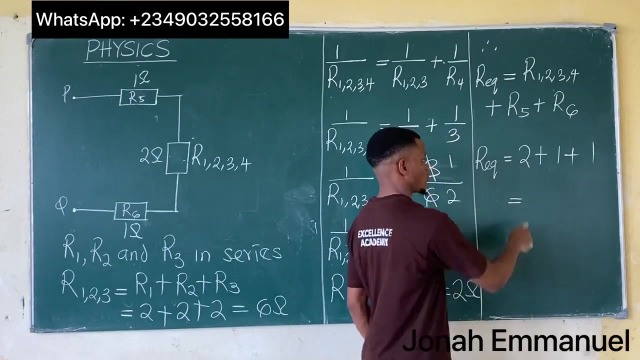 plus r five plus r6, so hence the equivalent resistance is equal to r one, two, three, four. this is two. when it comes, two plus r five is one, so plus one plus r six is also one, so plus one. so hence the equivalent resistance is equal to two plus one is three plus one is four. so my answer is: 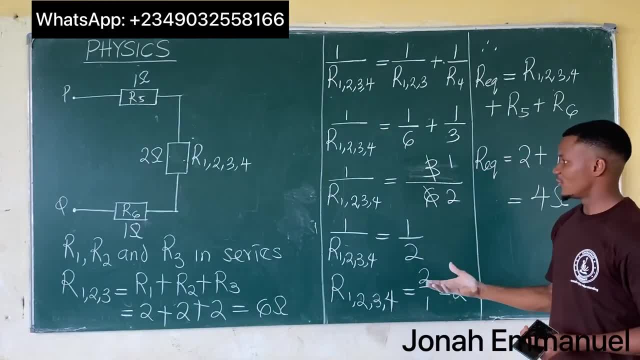 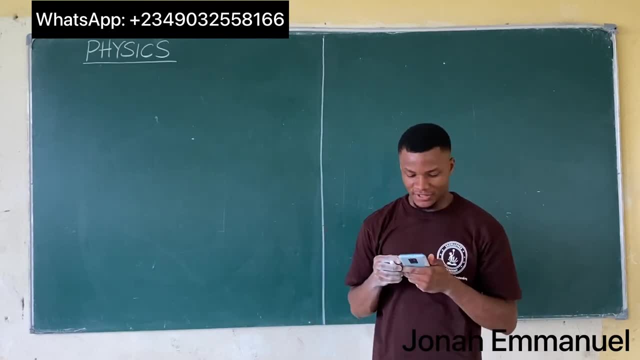 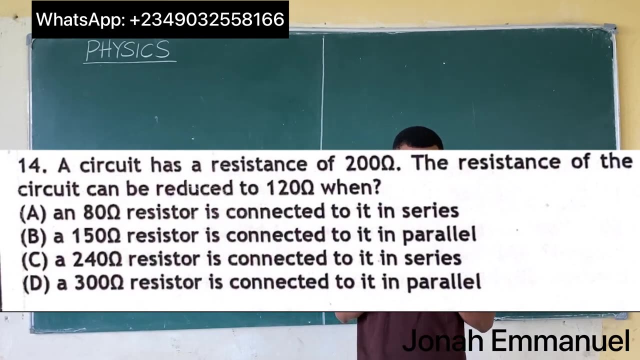 4 ohm. all right, so this is how you solve this question. all right, let's try this question. this question says a circuit has a resistance of 200 ohms, so stop. the resistance of the circuit can be reduced to 120 ohms when you have the option that a an 800 and 80 ohm resistor is. 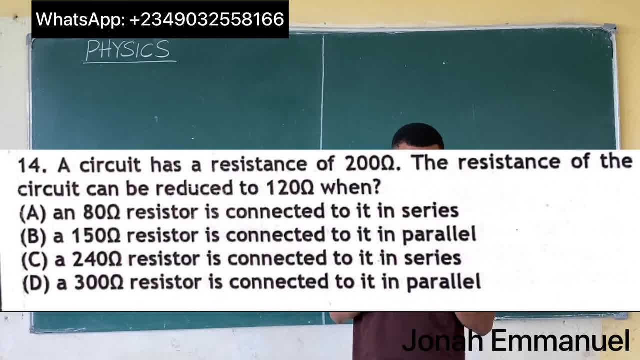 connected to is connected to it in series b: a 150 ohm resistor is connected to it in parallel. c: a 240 ohm resistor is connected to it in series d. a 300 ohm resistor is connected to it in parallel. all right, so let's highlight this question. what would it be? uh, what we have first. first of all, 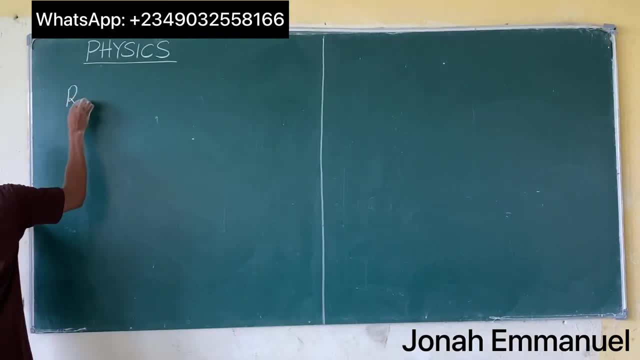 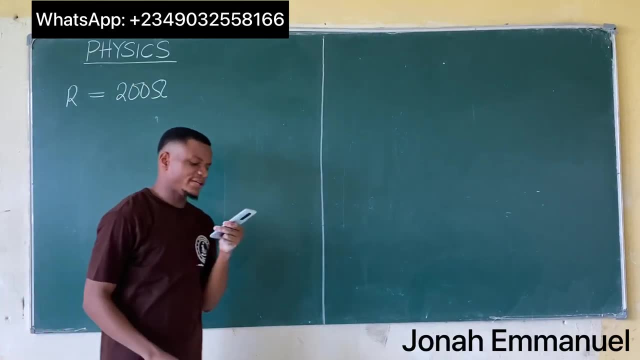 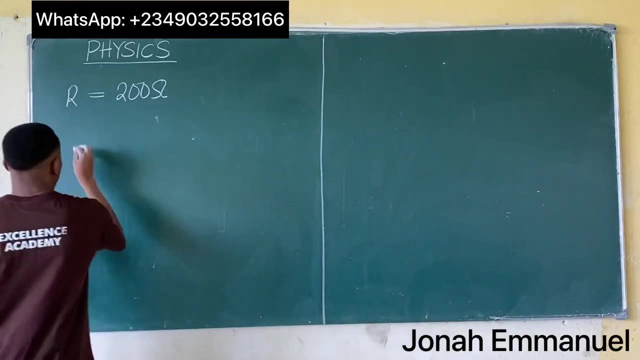 we have a resistance- um, let's call this iron instead of a body- is two ohms, so we have this. all right, let's represent. the resistance of the circuit can be reduced to 120, so let's say we have a second resistance. hence our phone is r1, our product is r2 will be equal to. 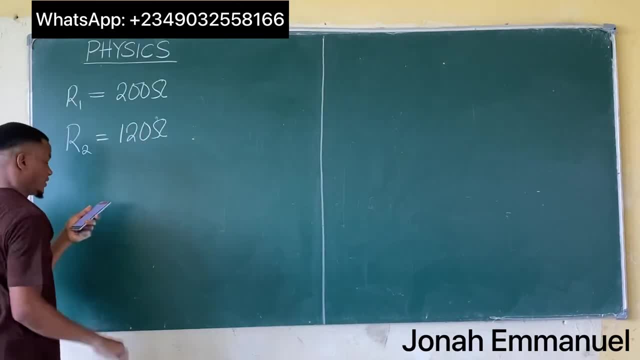 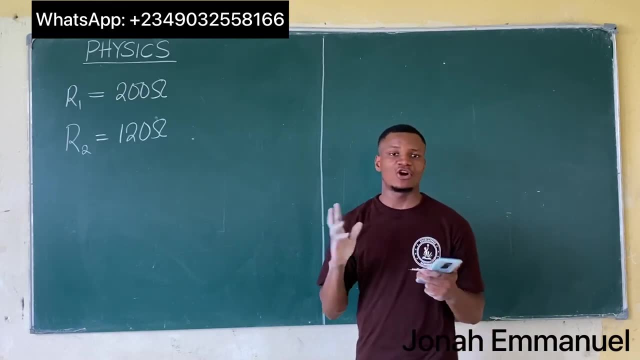 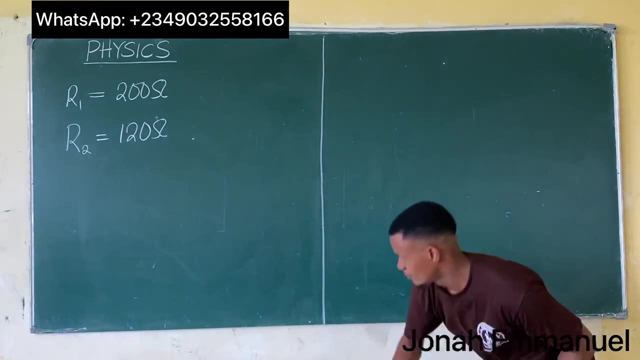 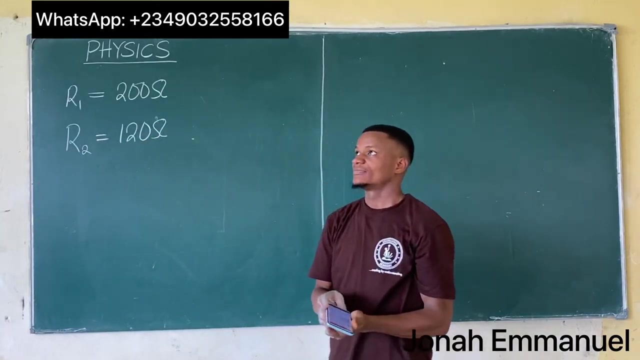 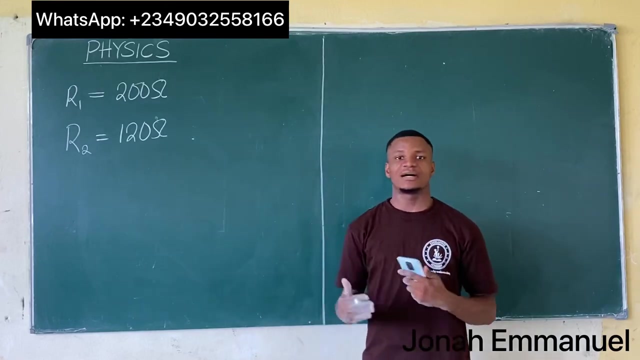 120. this all right, when what happens? that's what's here. um, at this point the picture is quite technical, but you have to understand the concept of resistance and how it works. resistance can be added in two ways. so we said at this point you have to understand how. 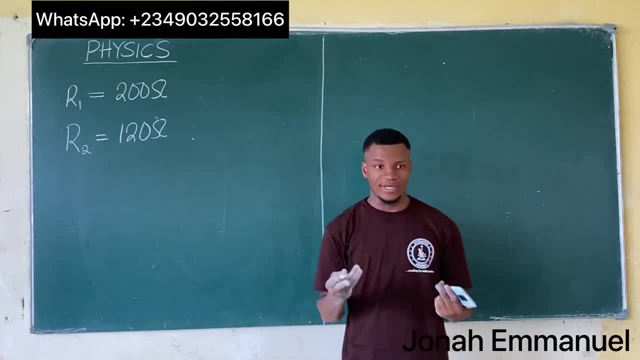 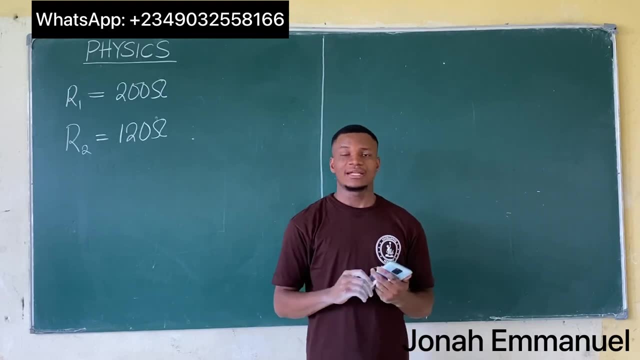 resistors work all right. resistors can be added in two ways: either in series or in parallel. when it comes to series connection, we add the values straight up. so in that case that means if i use series connection i will only increase the value of resistance, for instance. 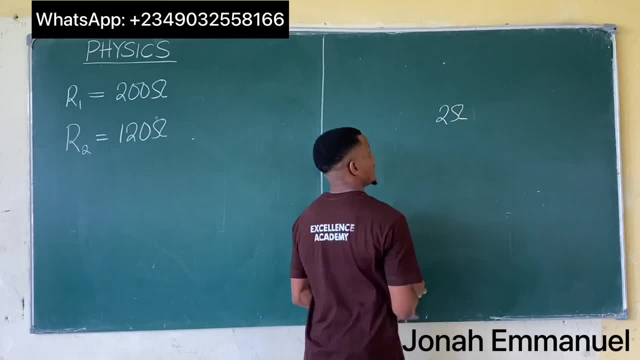 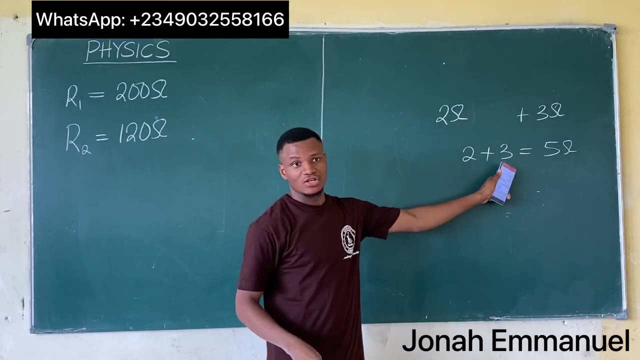 i have the resistance of, let's say, two ohms. let me connect a three ohm resistor in series. in series would mean i'm adding them straight, so it becomes two plus three, that's five holes. so whenever you connect resistance in series you only increase the resistance. But if you connect it in parallel, 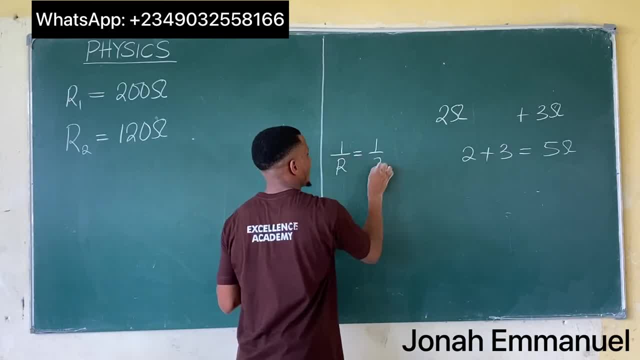 let's say 1 over R is equal to 1 over 2 plus 1 over 3.. If I take LCM, 6, 6 divided by 2, 3 times 1, 3, plus 6 divided by 3, 2 times 1, 2,, that's equal to 5 over 6.. This is the 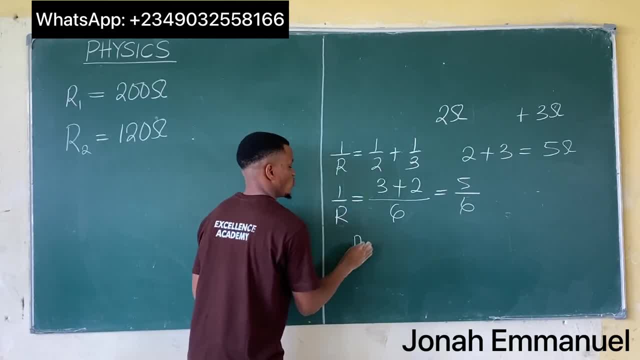 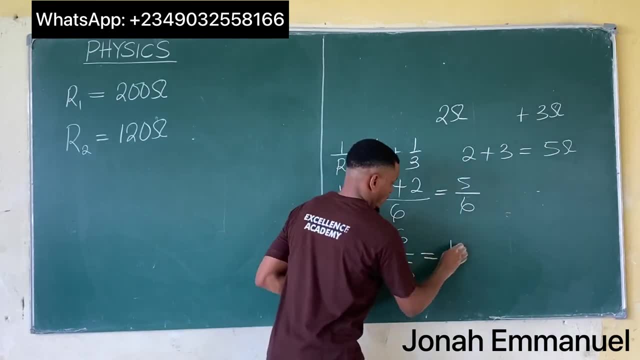 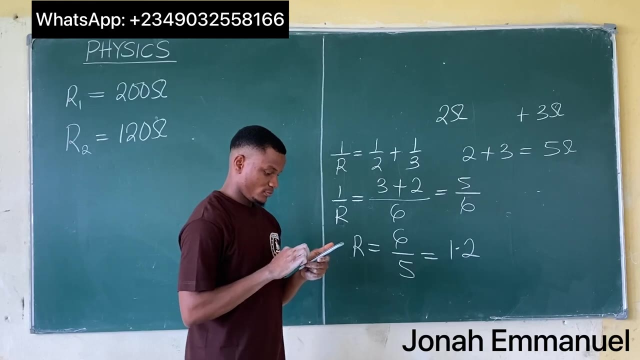 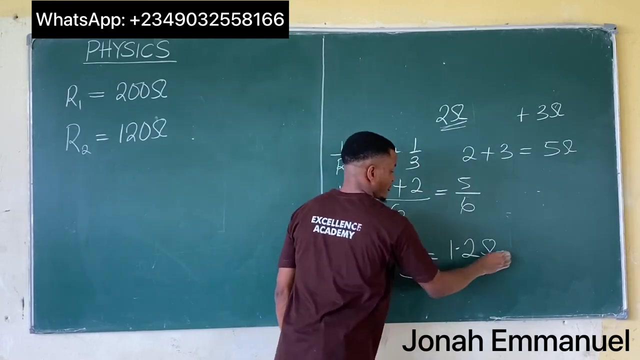 value of 1 over R. To get R we have to invert. That becomes 6 over 5.. 6 over 5 to the decimal is 1.2.. That becomes 1.20.. So observe that the initial value has been reduced Hence. 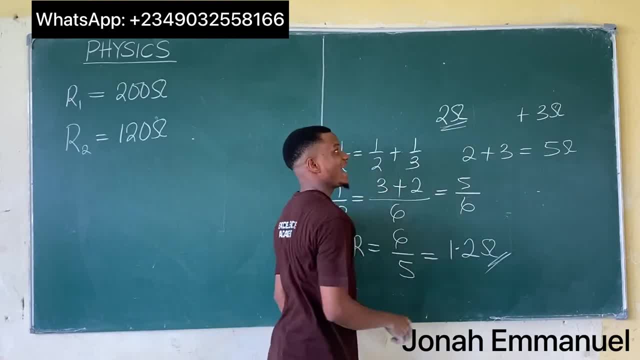 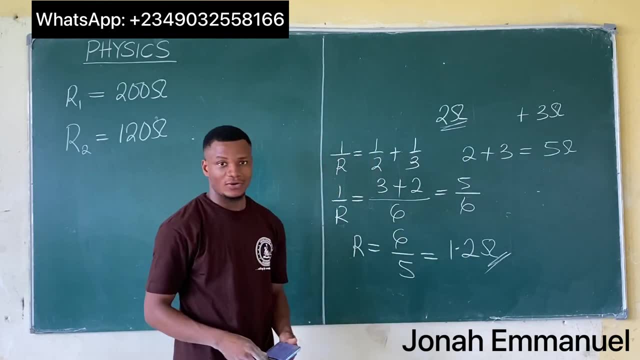 if I want to reduce the value of the resistance, I have to connect that resistance or dowel resistor, let's say in parallel to another resistor. That means from what I have there. I have four options. My answer has to be in parallel connection. 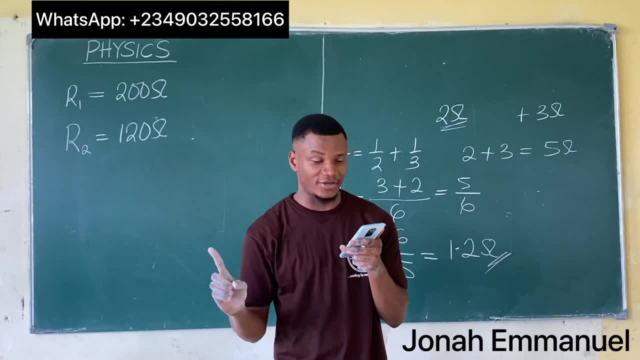 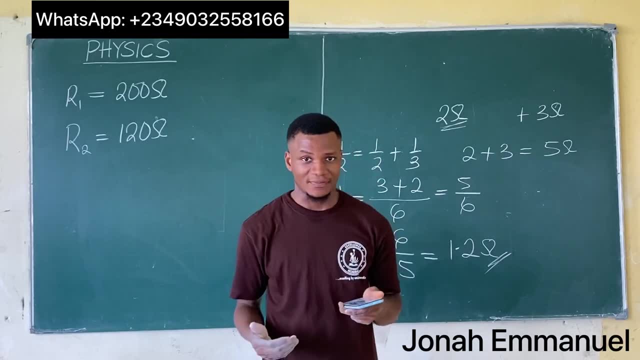 That means A cannot be the answer because A says in series. Also C cannot be the answer because C also says in series. So my answer is between B or D. Now I just taught you a technique. I just taught you a technique now used in answering OBJ questions. 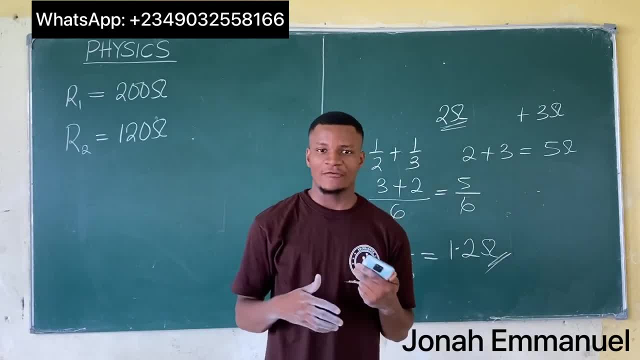 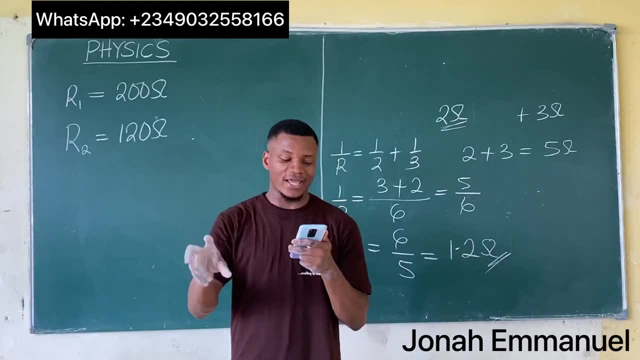 So if I'm giving you obvious equations there, one of the easiest way for you to answer it is to eliminate the options that cannot even be the answer, Just like in this case, option A and C cannot be the answer. I've explained why. So it has to be in parallel connection. 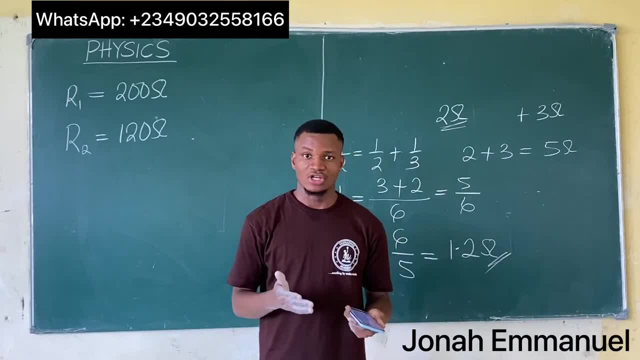 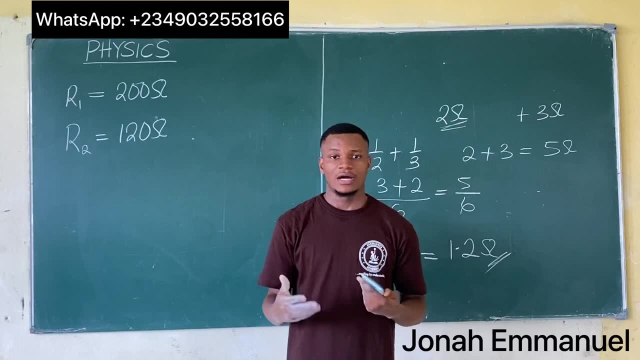 At this point I have between B and D to choose, So I now have a 50-50% chance of getting the correct answer. So it's a technique used in answering OBJ questions. Try to eliminate the options that cannot be the answer. It's a good technique for answering OBJ questions. 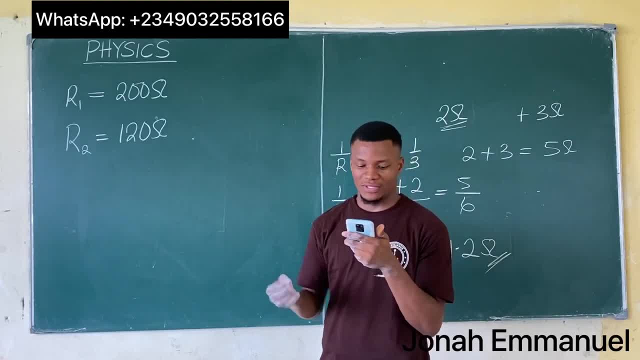 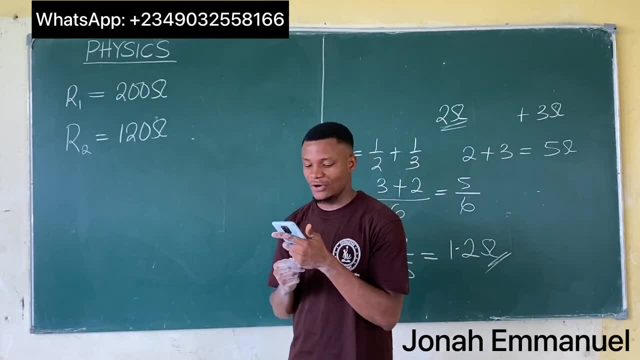 All right, Let's move on to our work. So my options are between B and D. So which will it be? Let's use B and C. B says let's connect a 150-ohm resistor in parallel, So this will. 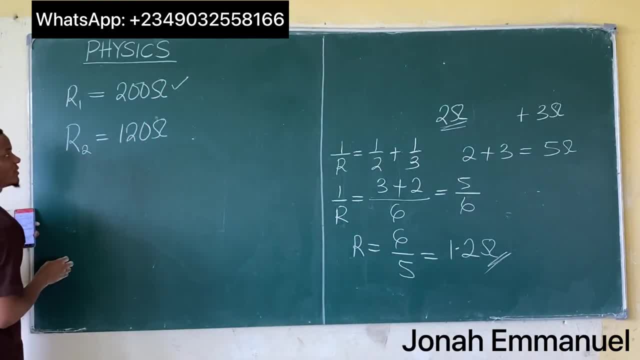 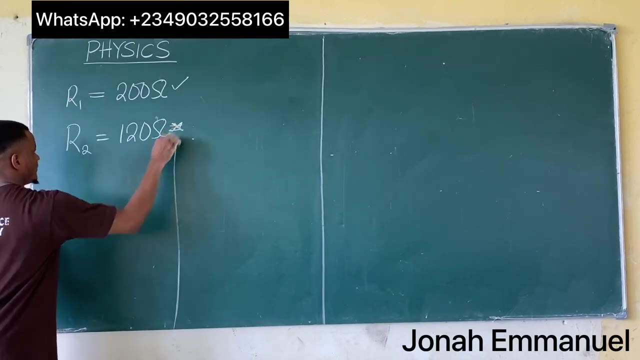 now be. Now, this was my initial resistor. So if I connect 150 in parallel, what do I have? I'll take this out first. All right, So let me connect 150 to this in parallel And see if I will get this as my answer. This one here, So I'm having 1 over R- is equal. 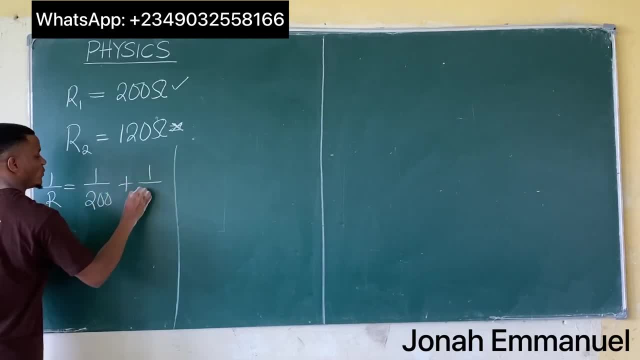 to 1 over 200 plus 1 over 150.. I'm taking inverse to show parallel connection. So 1 over R is equal to my LCM. here is 600.. All right, 600 over 200 gives you what 3 times? 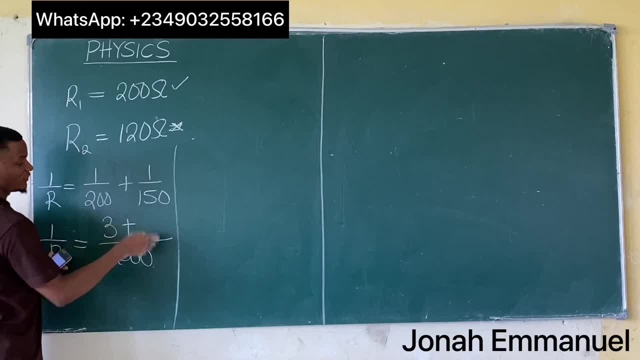 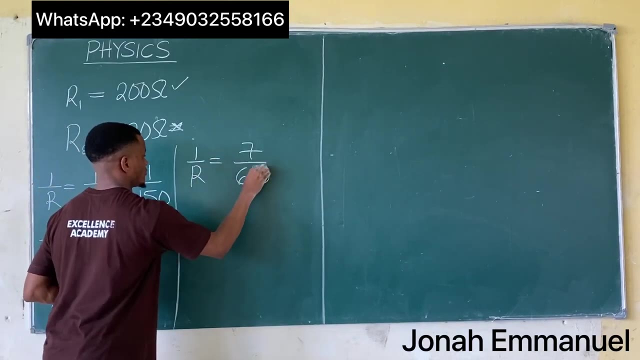 1. 3 plus 600.. 1 over 150 gives you what there 4.. So 1 over R is equal to 3 plus 4. 7 over 600.. So I have 1 over R is equal to 7 over 600.. Don't get R. So if you take inverse, So R is equal. 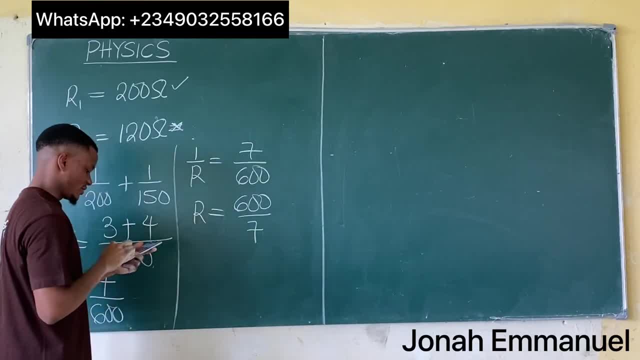 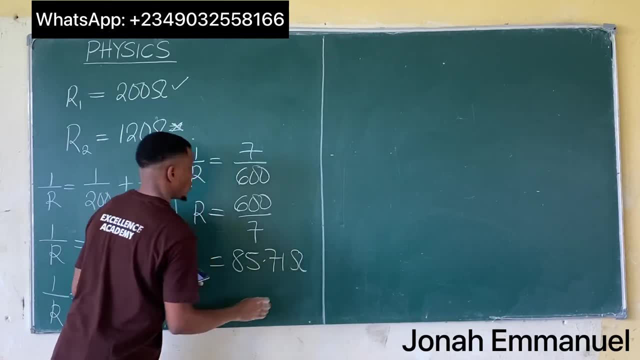 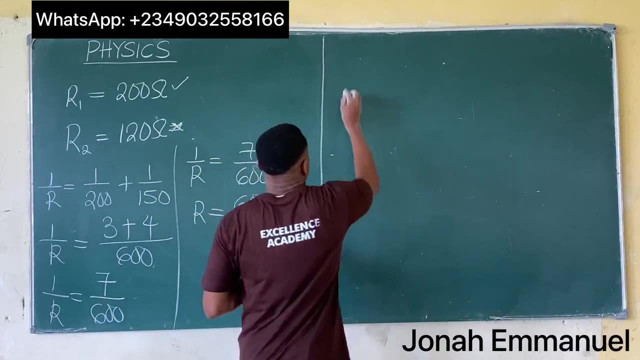 to 600 over 7.. Let's punch this 600 over 7.. That gives me about 85.71 ohm, which is not what you're looking for. So this is not it. So perhaps D might be an answer, But let's confirm. So, let's confirm. 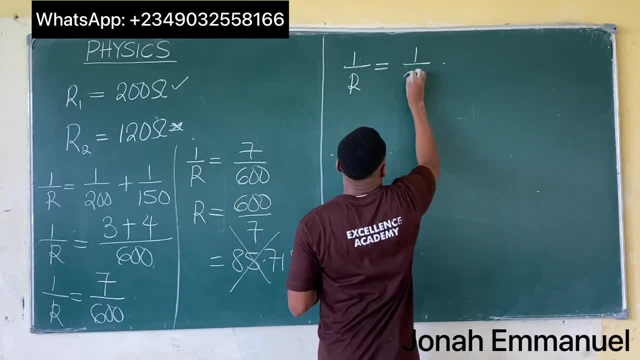 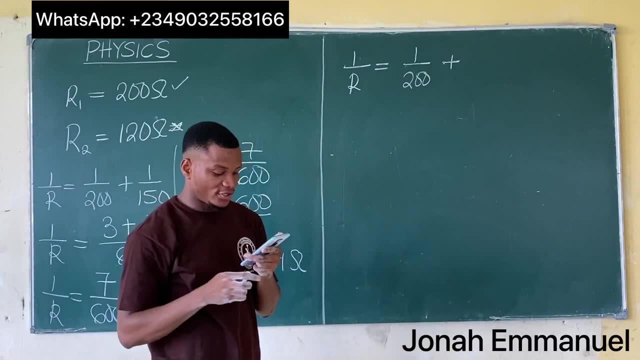 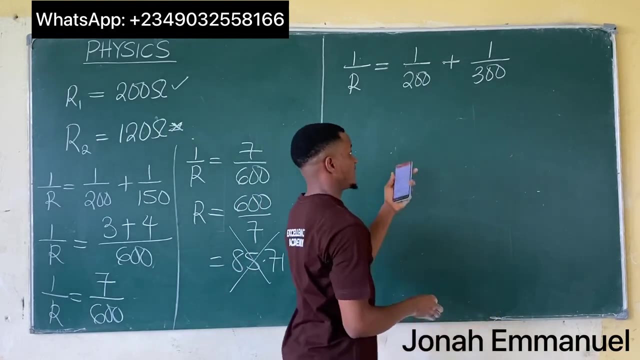 D. 1 over R is equal to 1 over 200 plus for D. they said a 300 ohm resistor connected in parallel, So 1 over. let's connect 300 in parallel. That becomes this: So 1 over. 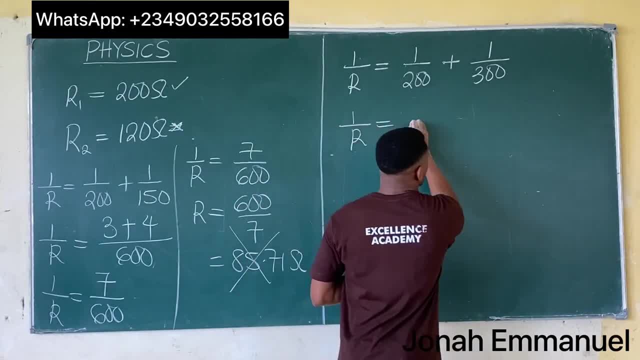 R is equal to LCM. of these two, to give you 600.. All right, So this is not it. So perhaps D might be an answer, But let's confirm. So let's retrieve the rest of all that I've got. Let's continue. 600 over 300, give you 600. 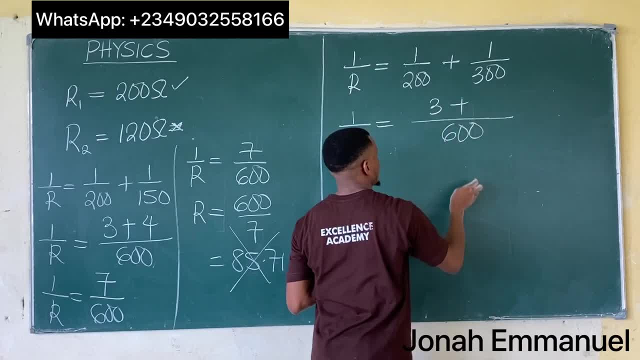 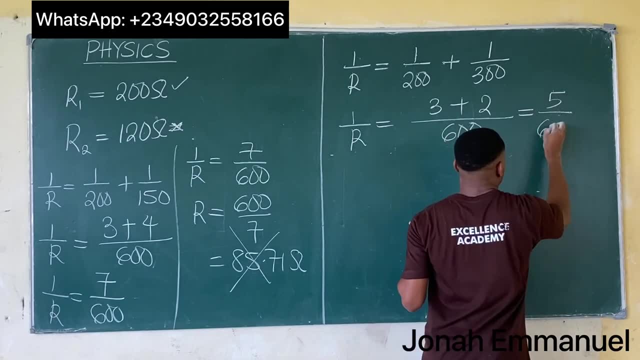 600 over 200 is 3 times 1.. It's 3 plus 600 over 300 is 2 times 1, is 2.. That gives you 5 over 600.. So I have: 1 over R is equal to 5 over 600.. 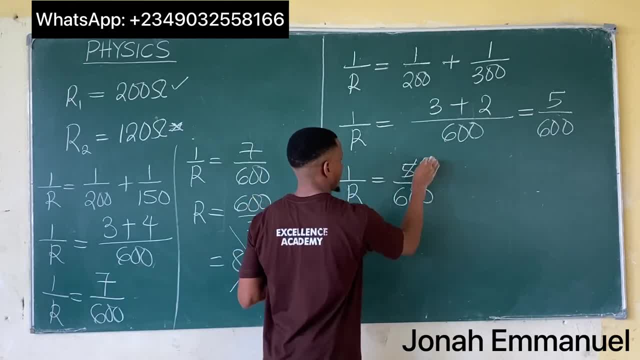 In the worst case, this here is 1.. This here is 120.. So you need to do: 1 over R is equal to 120.. Well, 1 over R gives 600.. This one I said было R� designing. All I said was cuatro. 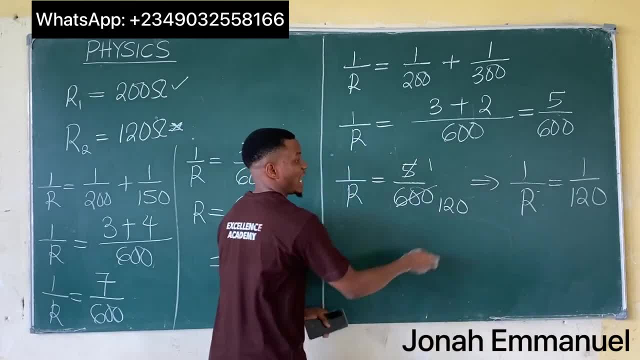 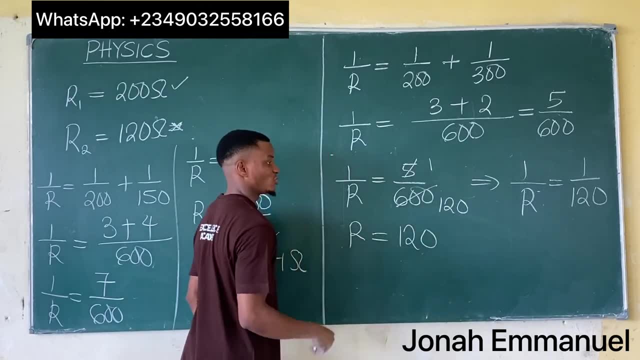 1 all over 120.. So let's get R. I will impact this. It becomes R over 1, which is R is equal to 120 over 1, which is 120.. So I'm having 120 there. So the answer is D. 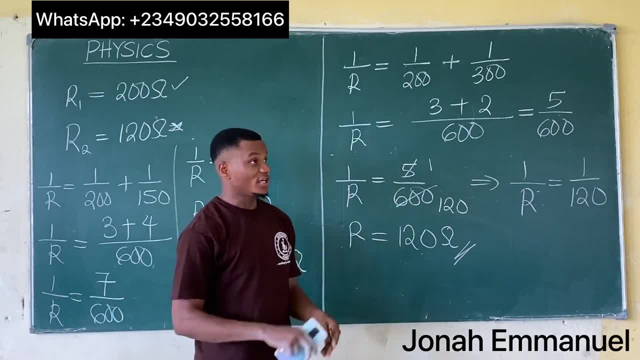 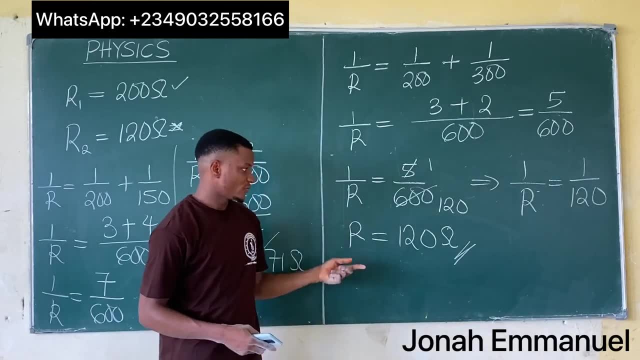 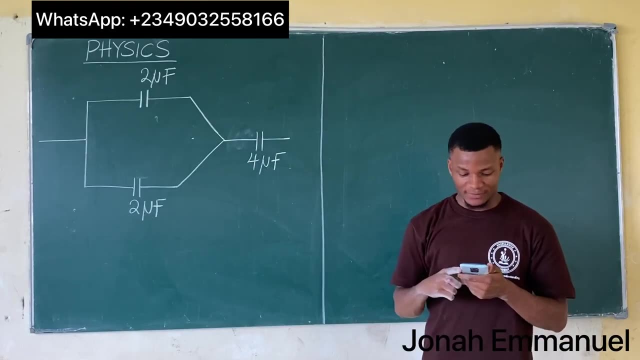 By connecting a 300-ohm resistor in parallel to this, we'll have the required reduced value of 120 ohm. So that's how you solve this question. All right, so let's try another question. This question says the net capacitance in the circuit above is: 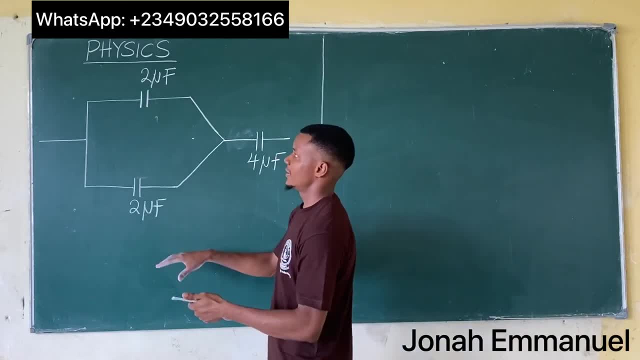 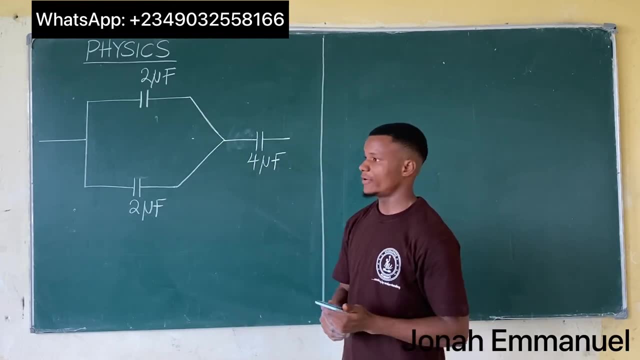 So that's my circuit. If I look at this, this is in connection of capacitors: 2 microfarad, 2 microfarad, 4 microfarad. Now I said, when you're solving things of this nature, 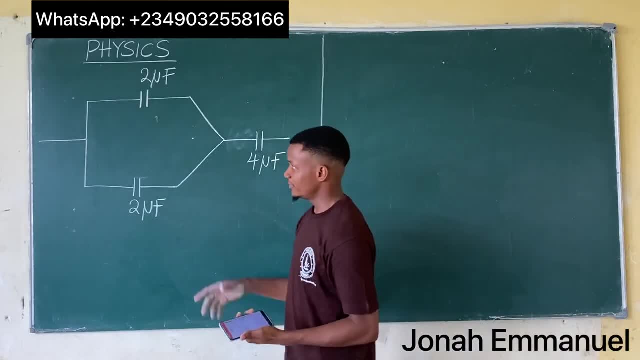 start from the closed end to the open end. For this one here, there is no real closed end and no real open end, So you have to figure out. where should this be? Where should you start from? For this case, I'm starting from this end to this way. 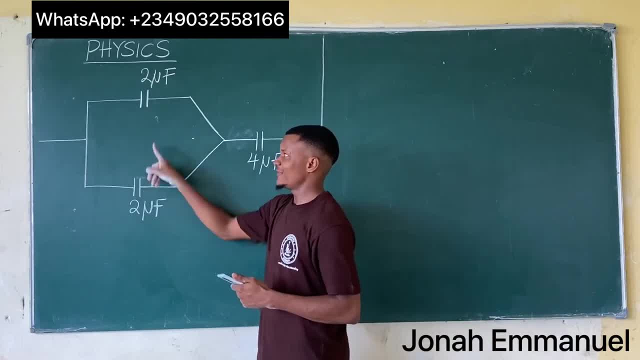 Now, in this case, my first stance is to resolve these two. If I look at these two capacitors, this and this are in parallel, So first of all, find the equivalent of these two in parallel. So let's call this C1.. 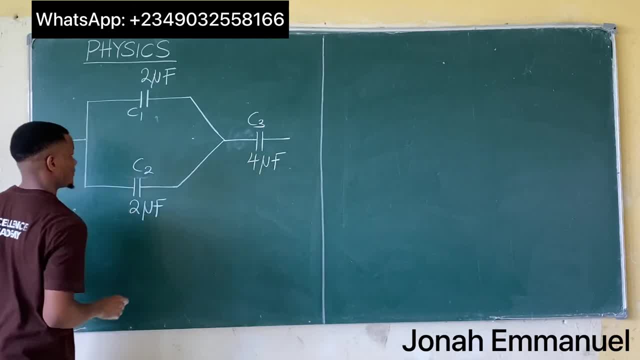 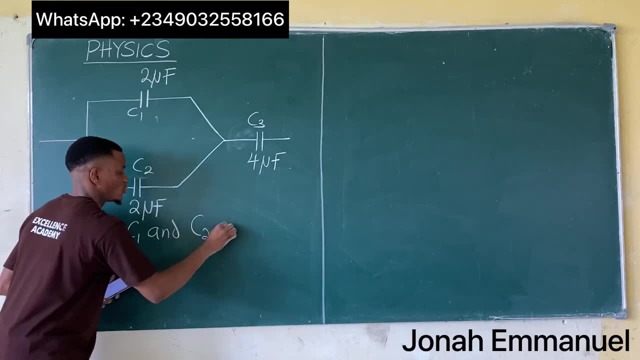 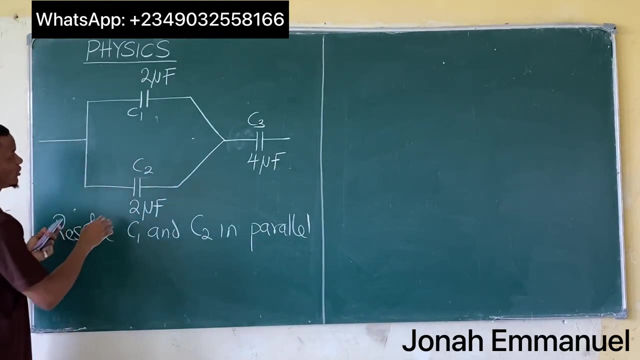 Let's call this C2.. Let's call this C3.. So let's resolve: Resolve C1 and C2 in parallel, Resolve C1 and C2 in parallel. So what do I have there? I have that in parallel connection of capacitors. 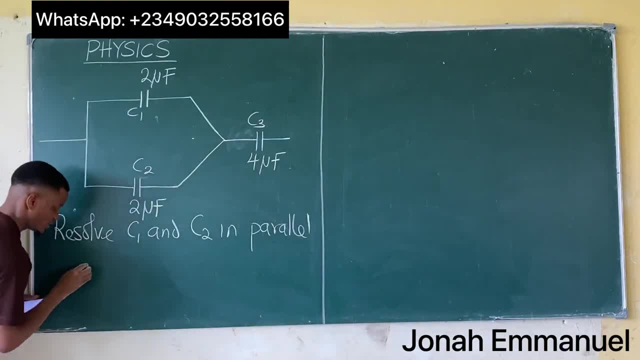 we said, we sum them up directly. So C1, 2, that's the equivalent, the equivalent capacitors of C1 and C2 is equal to C1 plus C2, as we discussed earlier. This is equal to C1 is 2 plus C2 is 2.. 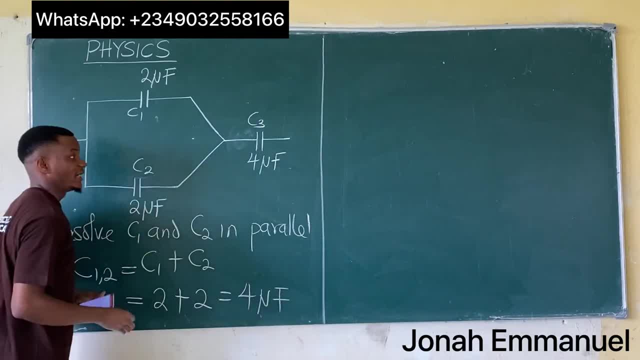 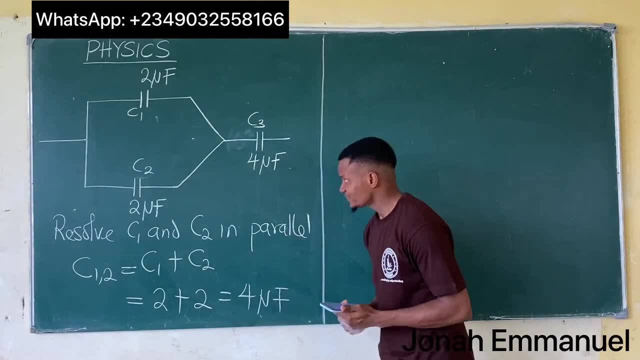 This gives you 4 microfarads. This gives you 4 microfarads. I agree I don't really have to compare here because they are all in the same unit, So we don't need to compare. So I have this. 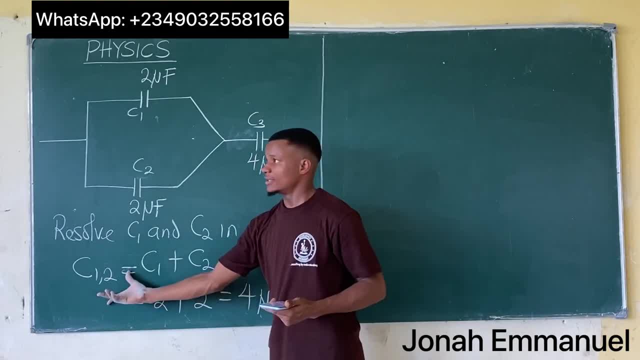 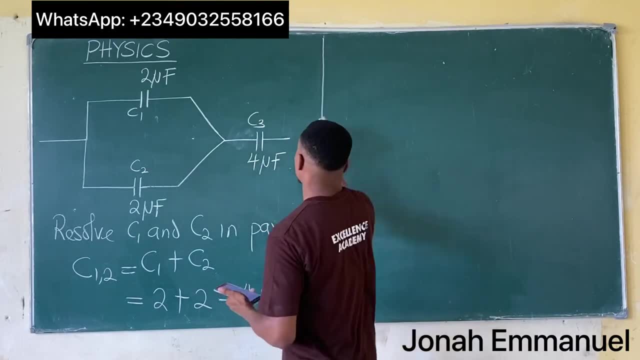 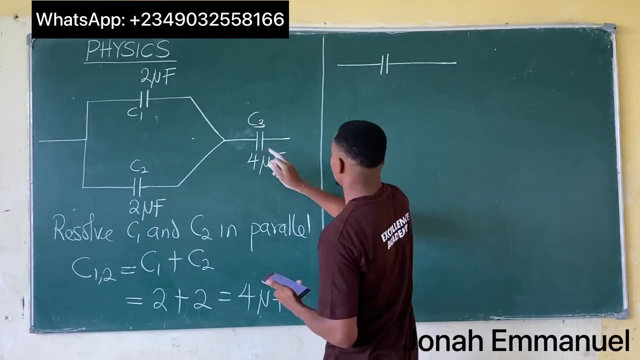 So if I'm putting this one here, how would this be placed Now? now, when we combine these two, these two becomes one here. So I will now have this: This two becomes one. That's this and this straight line to this one here. 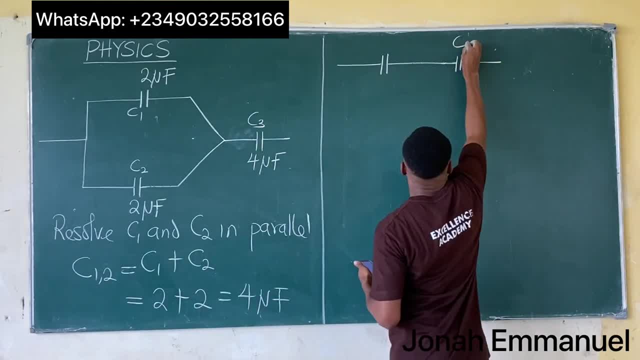 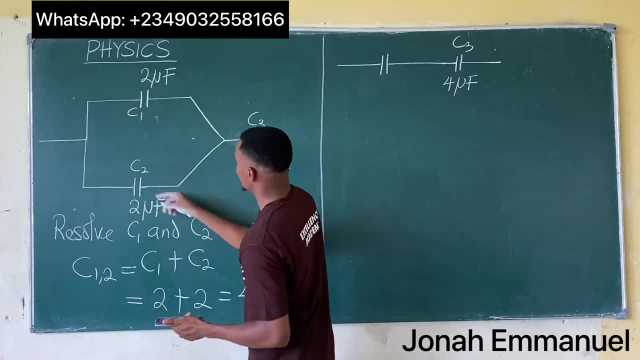 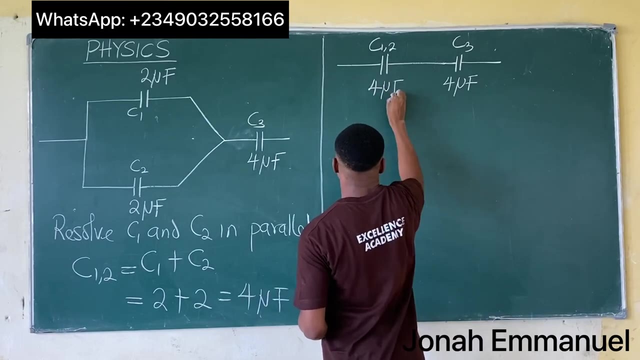 This and this, then this. This one here is C3, which value 4 microfarads. This one here is the combination of these two, That's C1, 2, whose value we got here as 4 microfarads. All right, so my final task will be to combine these two. 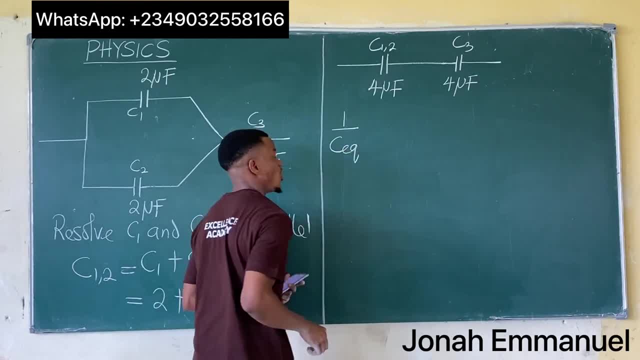 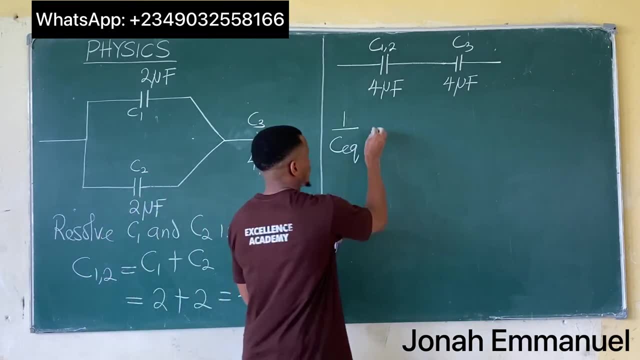 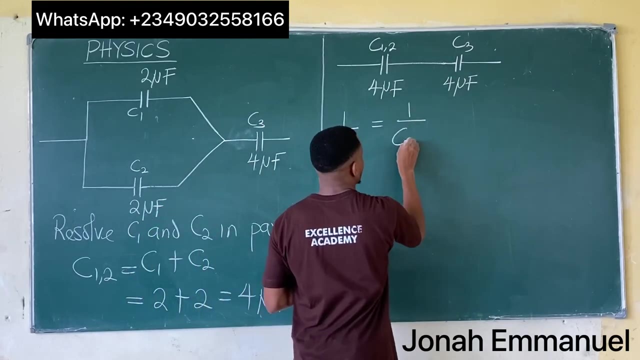 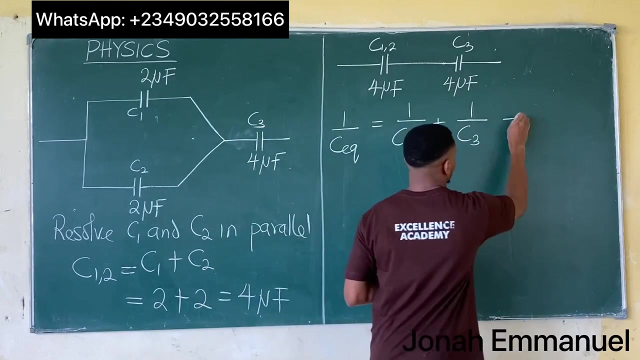 So hence one all over my equivalent or my net. When they say five net capacitors or equivalent capacitors, they mean four. they are the same thing. so this is now equal to for series connection of capacitors we said: take inverse becomes 1 over c12 plus 1 over c3. so if i sum this up, this is equal to 1 over c12, is 4 plus. 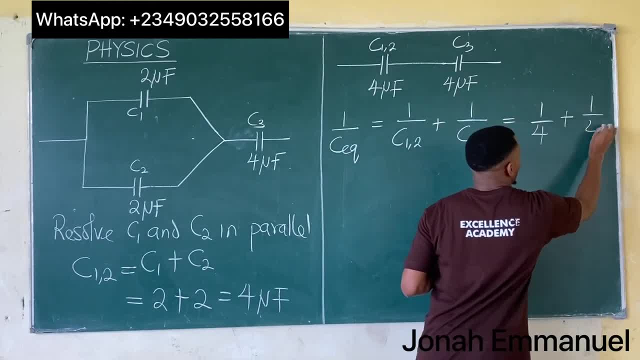 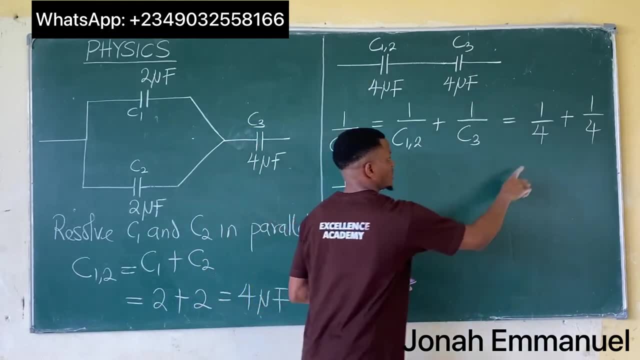 c3, you can see there is also 4.. all right with this. now i have that. 1 all over ceq is equal to the lc of 1- 4. my lcf is 4. 4 divided by 4 gives you 1 times 1 is 1 plus 4 divided by 4 gives you 1. 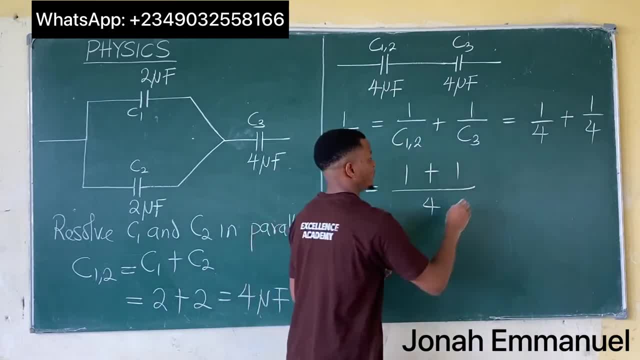 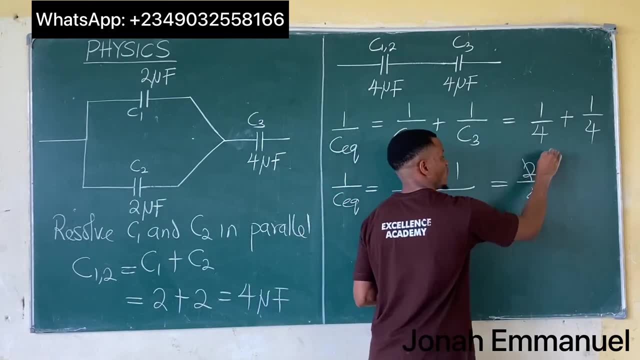 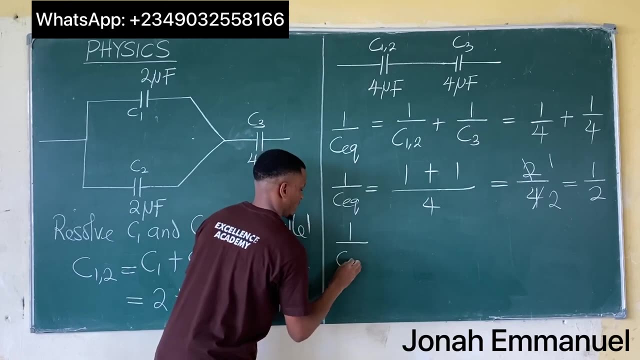 times 1 is 1. so it happens, if i combine this is equal to 1 plus 1 is 2 all over 4. in the 2 here 1, 2 here 2. that's equal to 1 over 2, so hence 1 all over the equivalent is equal to. 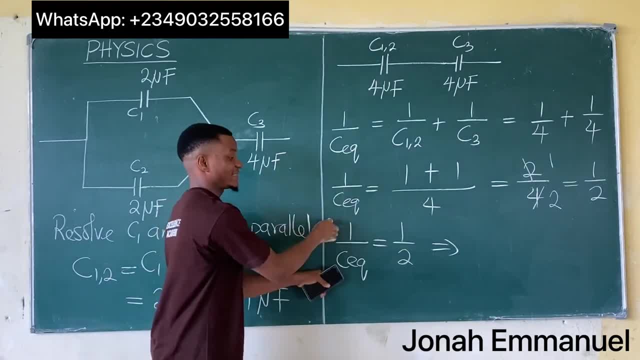 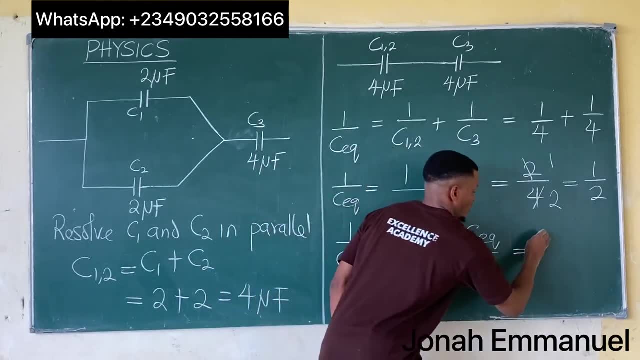 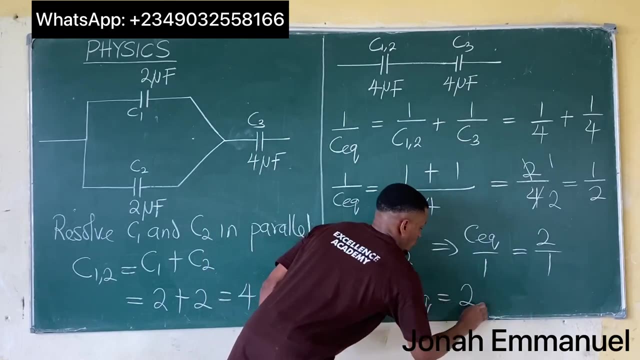 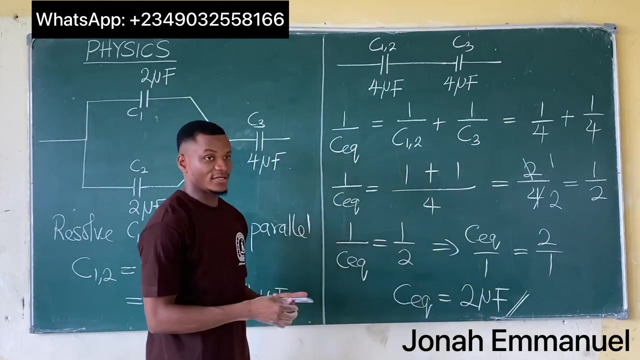 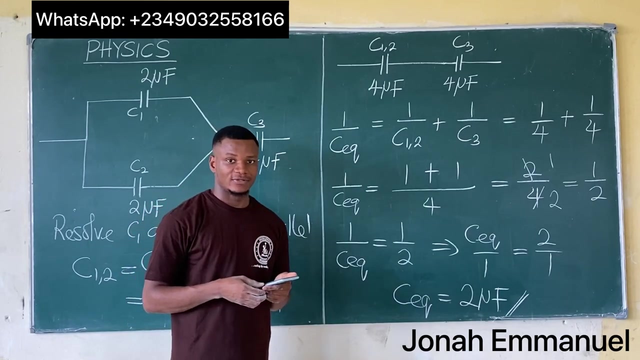 1 over 2. to get my equivalent, simply invert. that means ceq over 1 is equal to inverse. these two becomes 2 over 1, hence the equivalent capacitor or the net capacitor is equal to 2, my new, so my answer is 2 micro farad and that's option d, 2.0 micro farad. that's how you solve this question. 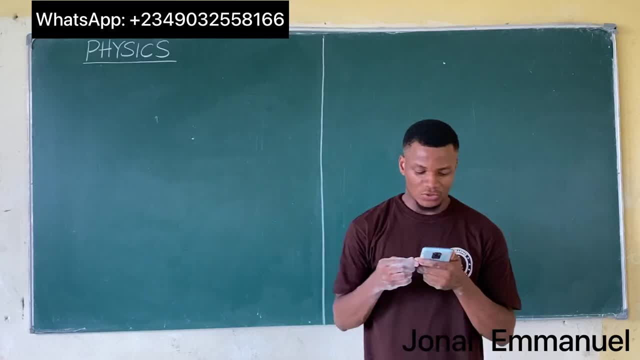 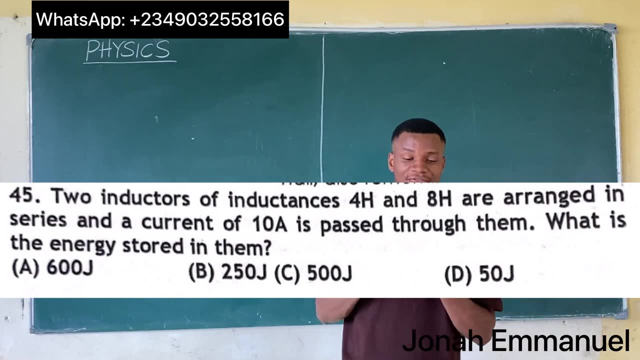 all right, let's try another question. it says two inductors of inductances, 4 henry and 8 henry, are arranged in series and a current of 10- happens- is passed through them to stop. what is the energy stored in them? that's the question, all resolution. my first task is to 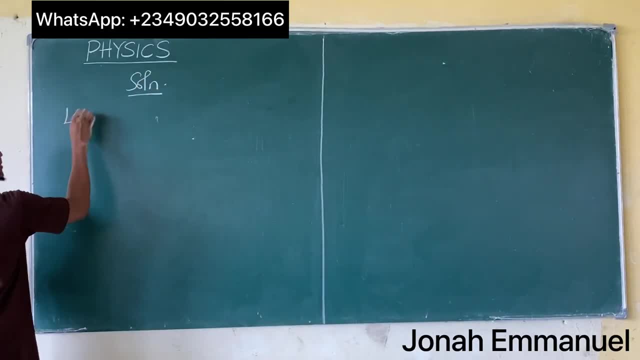 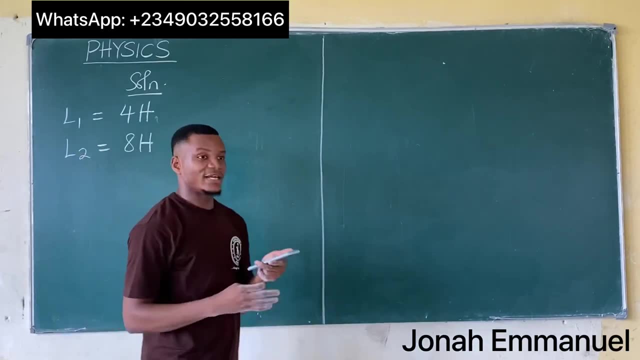 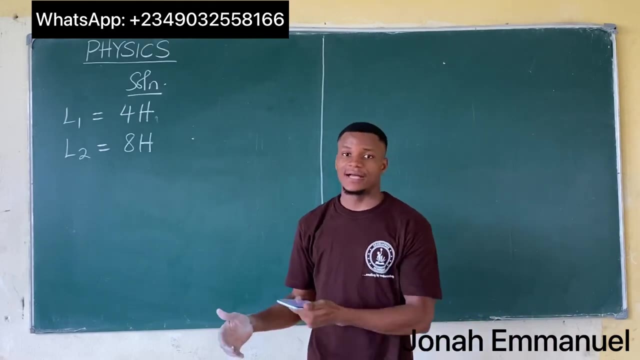 list out my inductors from giving my first inductor as 4 henry and my second inductor as 8 henry. but he said they are arranged in series and we said inductance on inductor in series is the same thing as, or the same pattern as, resistors in series. that means i'll just combine. 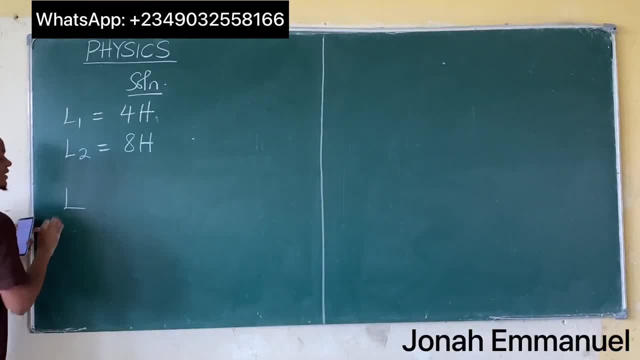 them straight on. ok, now we read the body of the inductor and we say what is the energy stored in? So hence my equivalent inductance is equal to simply sum these two. If I sum them, I have L1 as 4 plus L2 dash 8.. This gives you 12 henry. So this is my equivalent inductance. 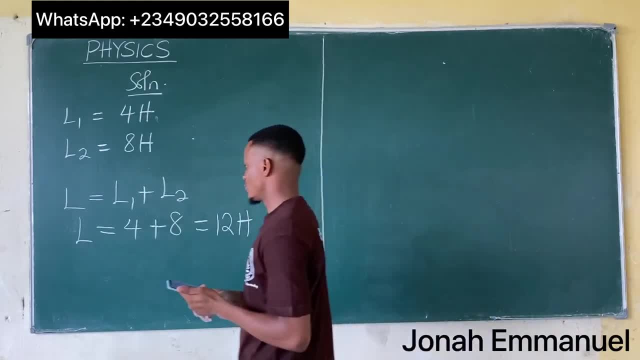 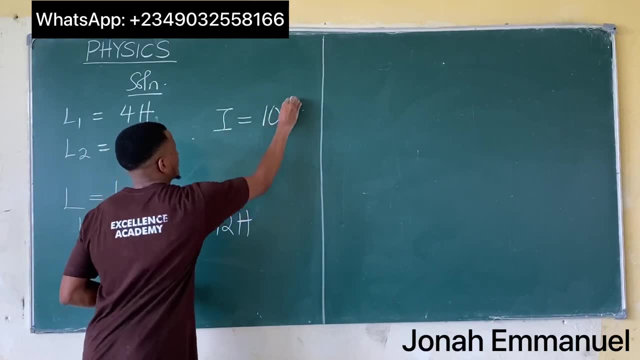 Next, let's see if you find the empty stone in there. So recall, Alright. Also, given the current, I has been equal to 10 amperes, So the current is 10 amperes, So let's get this done. 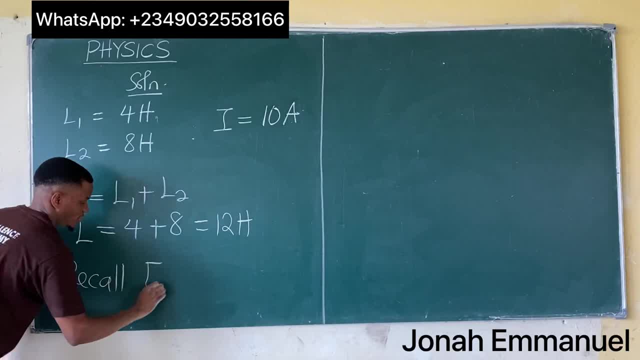 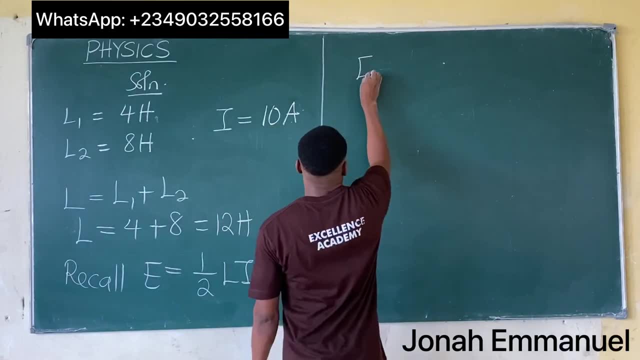 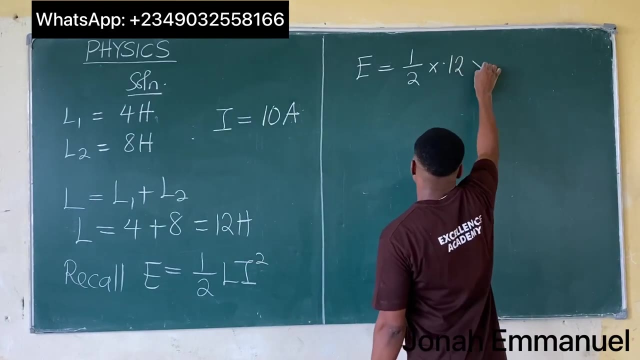 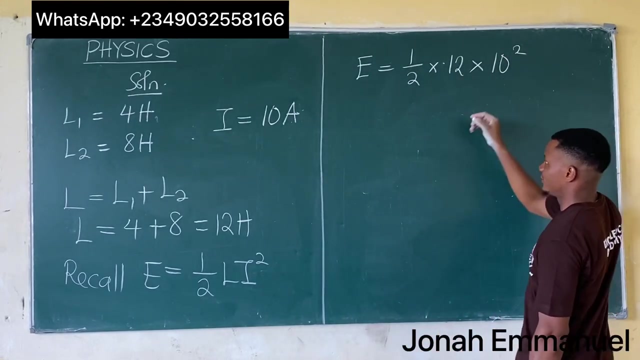 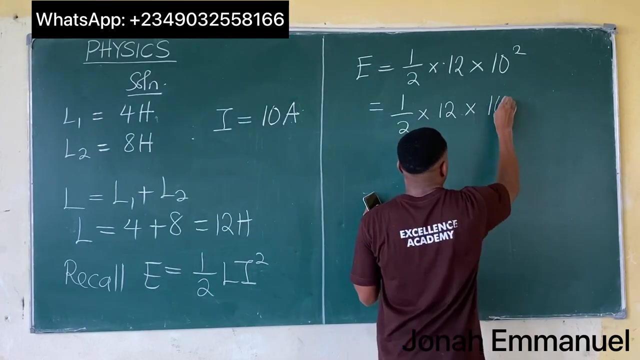 So recall that we said energy E is equal to half Li squared for an inductor. So hence E is equal to half times L. equivalent inductance 12 henry times the current, That's 10 squared. So half Li squared, This is equal to half times L12 times 10 squared is 100.. 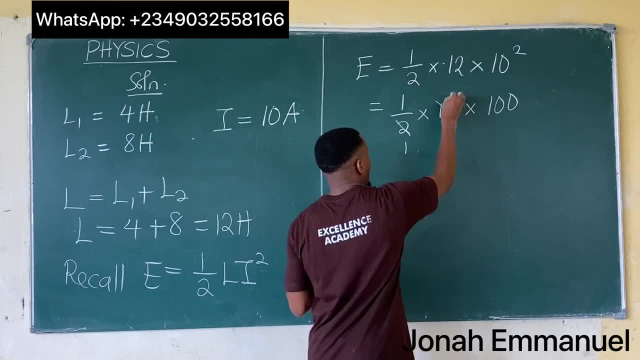 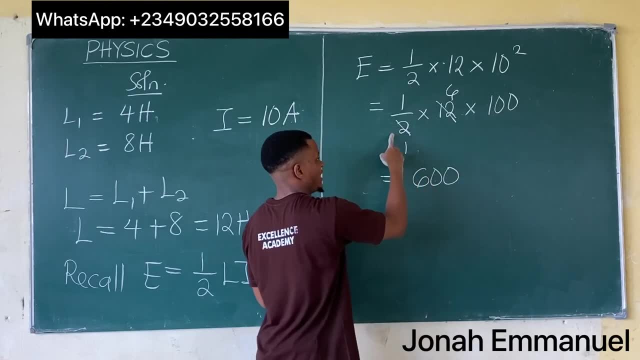 So let's get this done. 2 here 1.. 2 here 6.. 1 times 6,, 6 times 100.. That's equal to 600.. Of course, divided by 1,, which is 600 in joules. 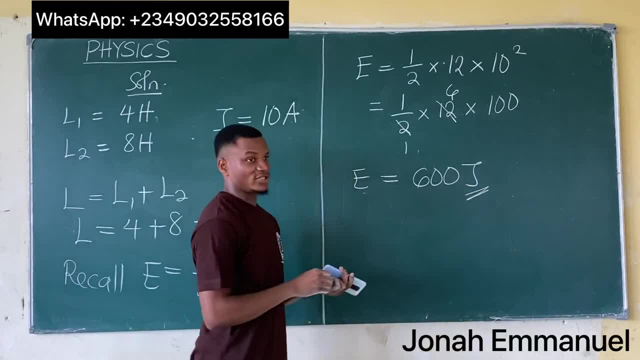 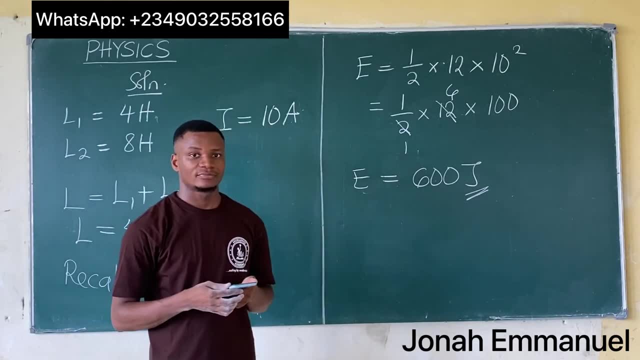 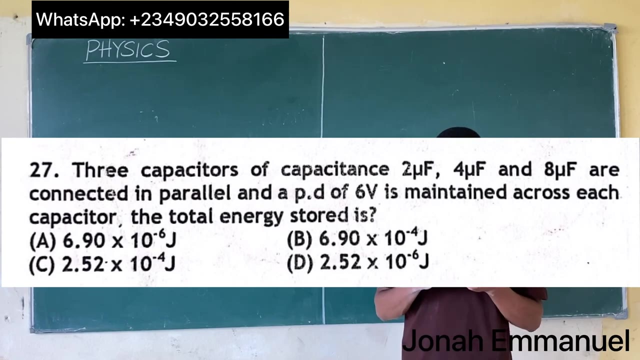 So hence the energy is 600 joules. That's the answer And that's option A: 600 joules. So this question says: 3 capacitors of capacitance, 2 microfarad, 4 microfarad and 8 microfarad are connected in parallel and a potential difference of 6 volts is maintained across each capacitor. 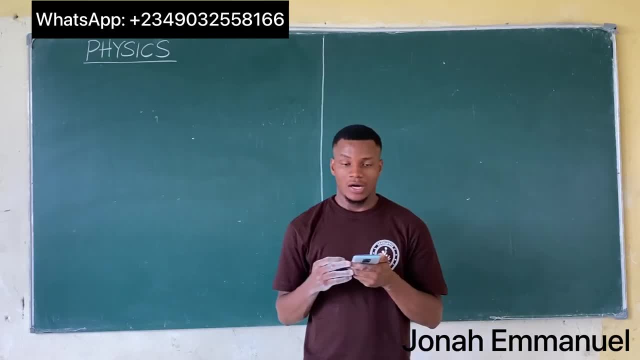 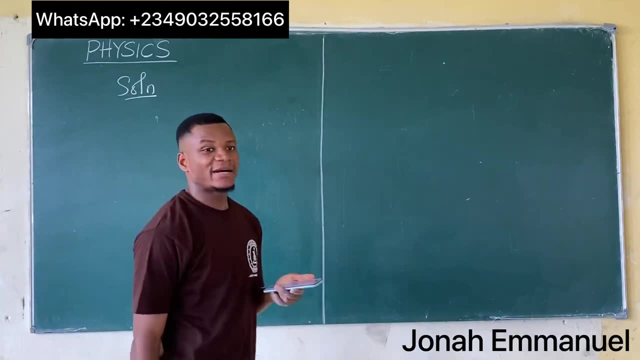 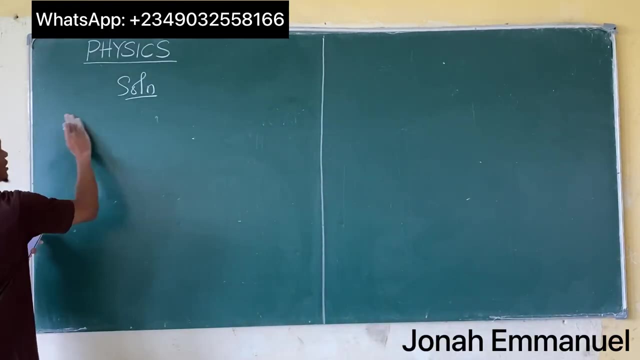 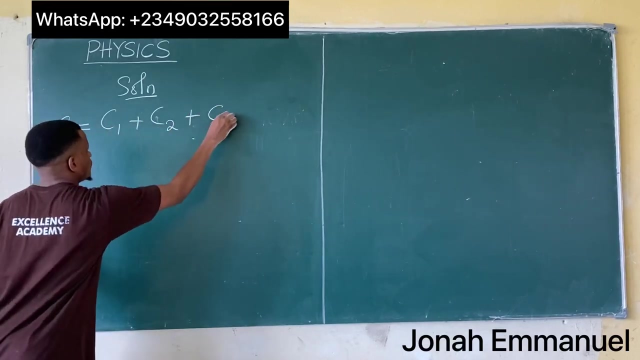 The total energy stored is- let's get this done um solution. so, given three capacitors having capacitors of two, four and eight micro farad, so we said capacitors in parallel, so i'll have that in parallel. my equivalent capacitor c is equal to c1 plus c2 plus c3 for capacitors in. 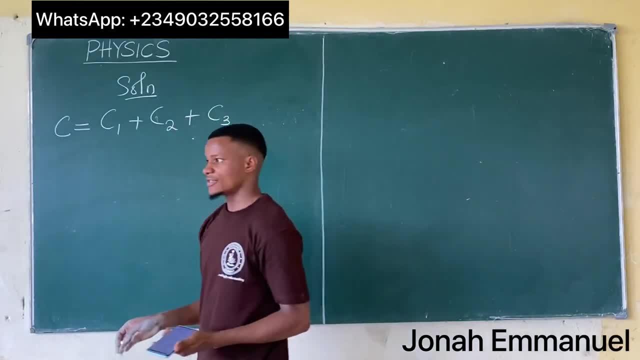 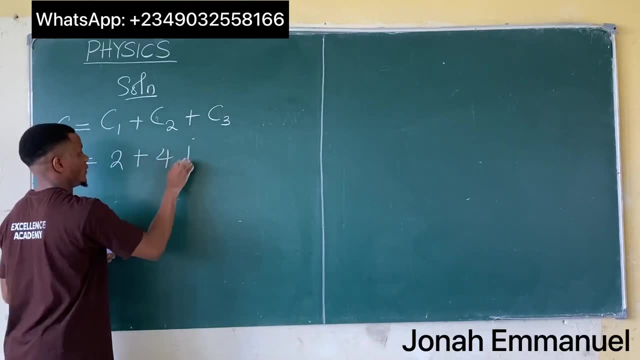 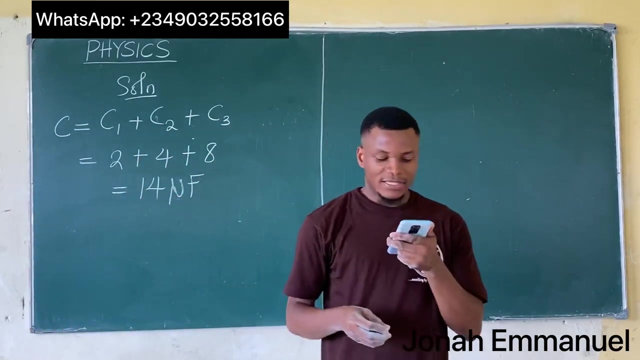 parallel. we said something of strength, so i have this. so this is now equal to c1. the first thing then is 2 plus c2 is four plus c3 is eight. if i combine this, it gives me fourteen microfarad. so my Rick blueprint is 14 microfarad. next up, it gives us potential. 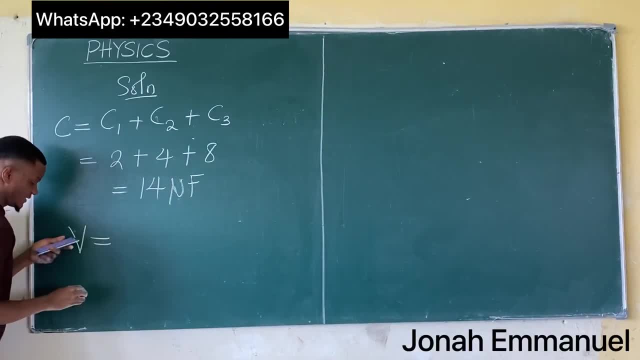 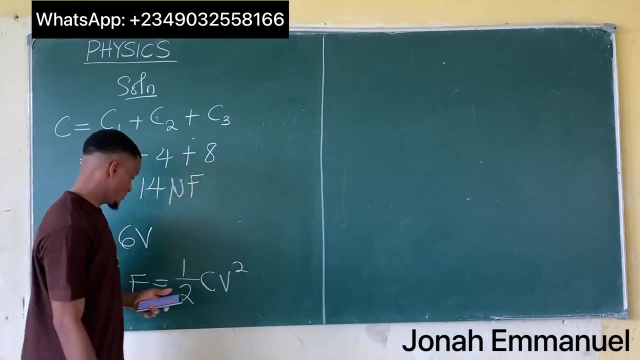 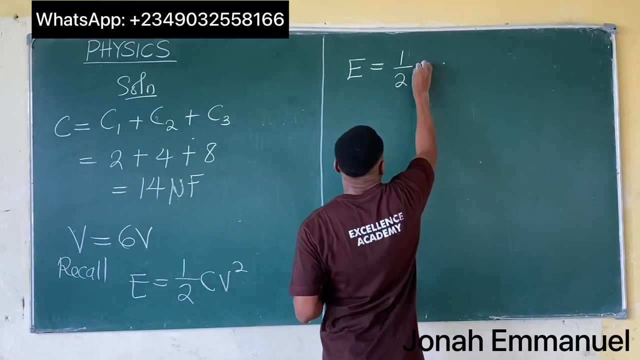 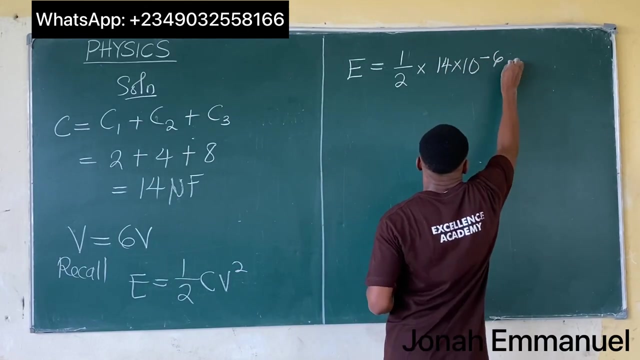 difference of the voltage v as 6 volts. you'll also find the energy store in primary and secondary depuis point c, fase capacitor. so recall, recall that we say energy store in capacitors. e is equal to half c v squared. so so e is equal to half times c, equivalent capacitance 14 times k to power minus 6 times. 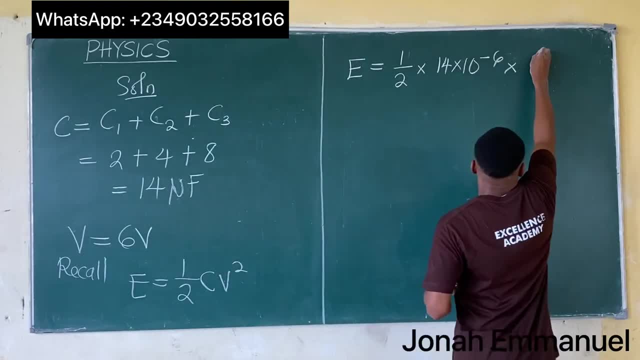 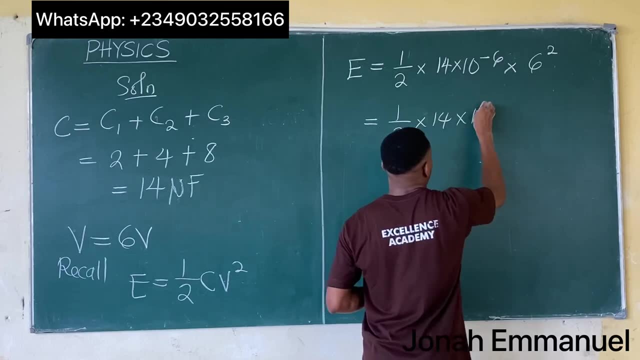 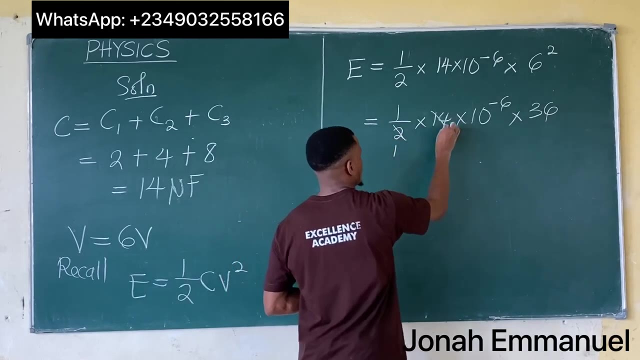 v squared. v is 6, it becomes 6 squared. so this is now equal to half times 14 times 10, to the power minus 6 times 6 squared is 36.. so 2 here 1, 2 here 7.. if i multiply this is equal to: 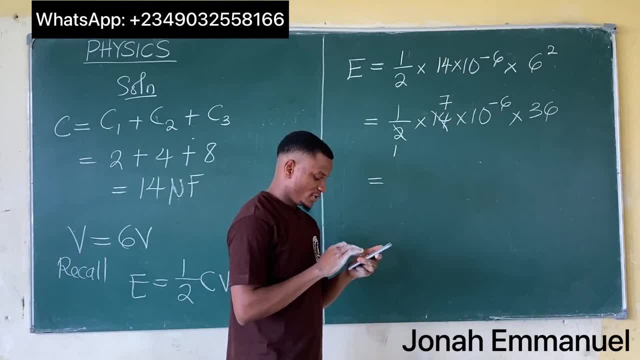 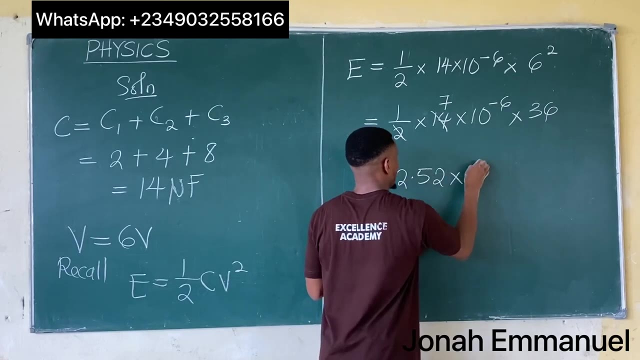 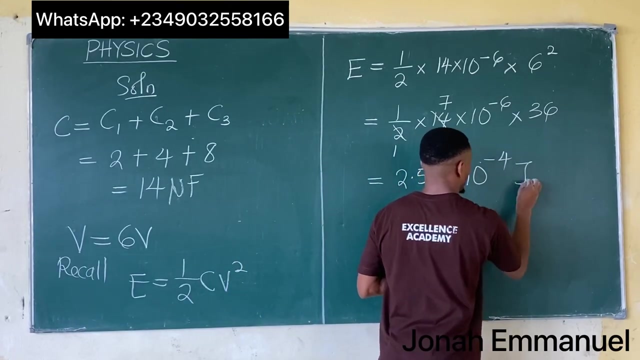 seven times seven times 10 to the power minus 6 times 36. so i have 2.52 times 10 to the power 1, 2, 3, 4 minus 4 joules. so that's the value of this: 2.52 times to the power minus 4. 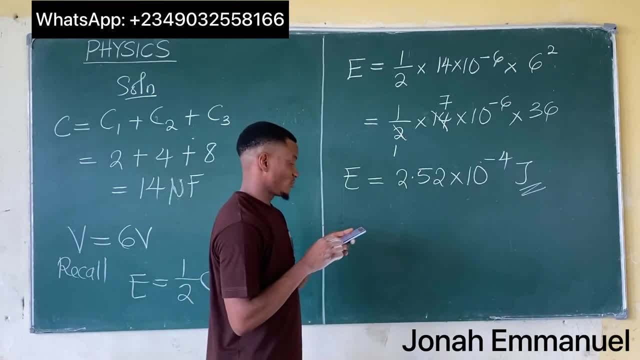 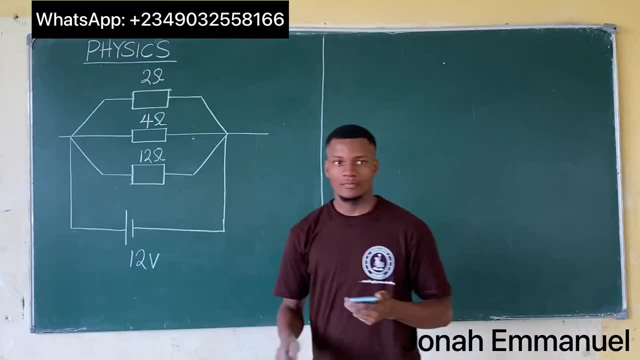 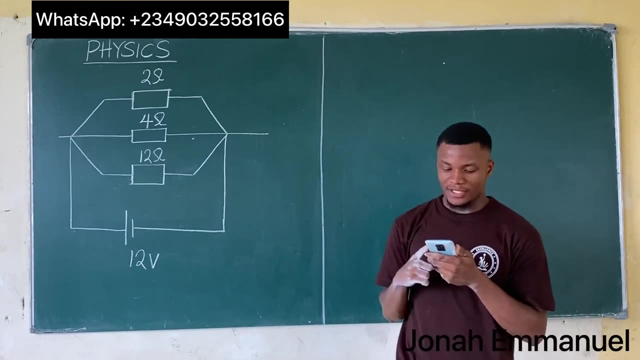 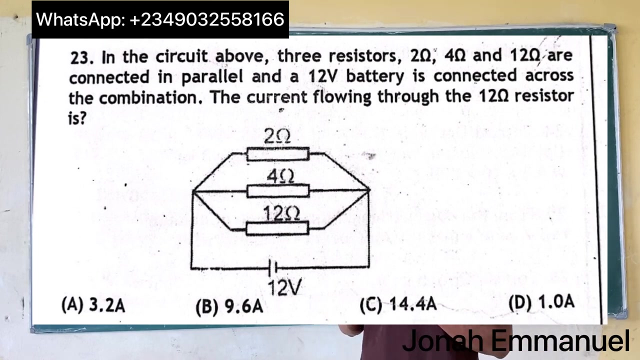 that's the value. that's option c: 2.52 times to the power minus 4. so this is how you solve this question. all right, so let's look at another question here. it says in the circuitry, three resistors- two ohm, four ohms and 12 ohms are connected in parallel and a 12 volt battery is connected. 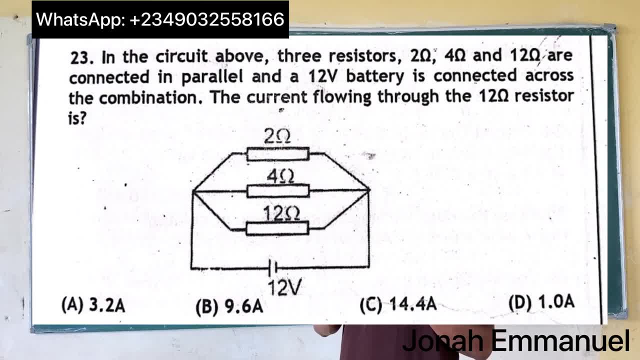 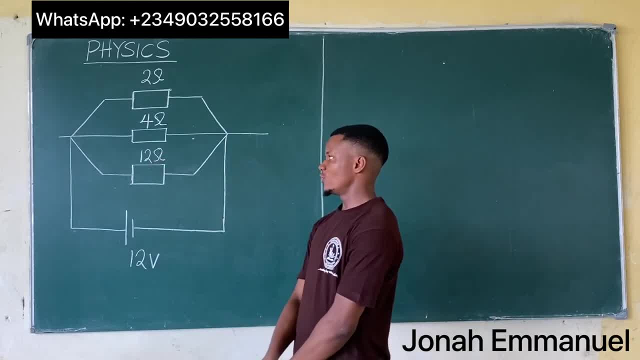 across the combination. the current flowing to the 12 ohm resistor is all right, so we have to find the current flowing through this one here, the 12 ohm resistor. now here's what you should note. note that in a connection like this or in parallel connection, 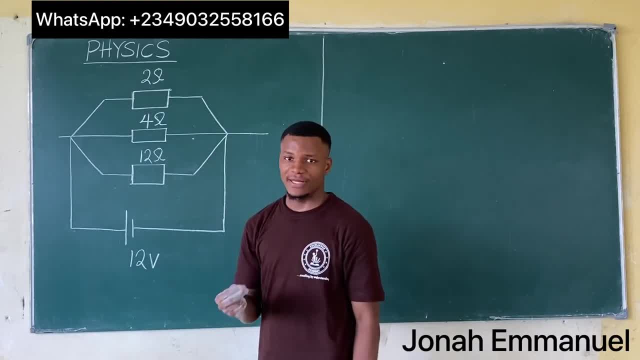 of resistance. note that the same potential difference or the same voltage flows through each of the resistor. that means the potential difference here is what you have here as well. it's people difference here: 12 is what you have here, the potential difference. the potential difference 12 is still what you have here. also, the potential difference here is still what you have here. so 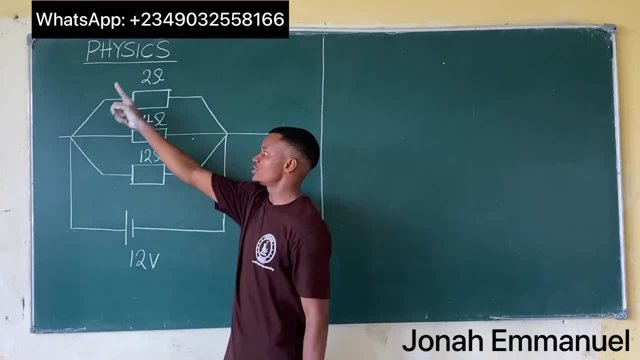 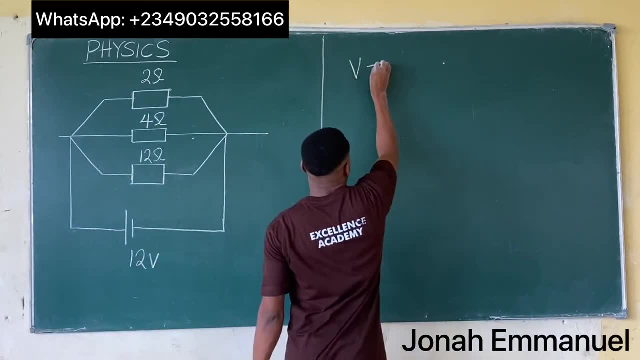 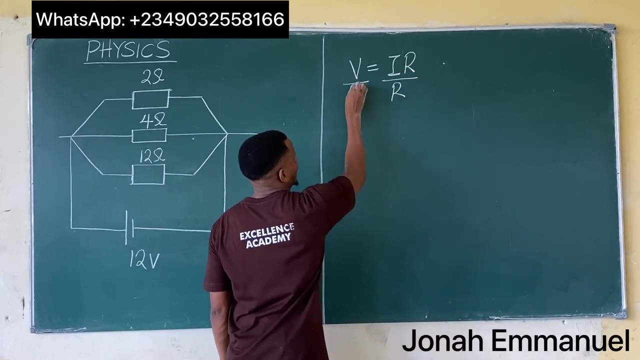 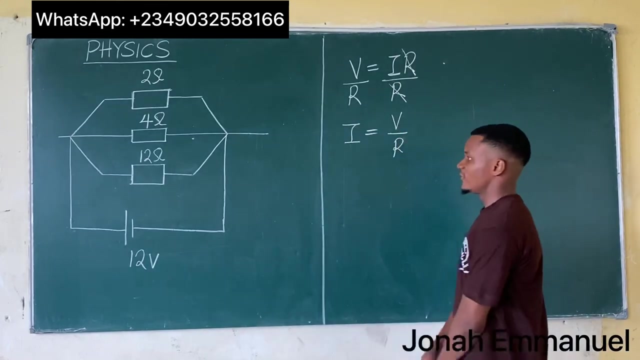 this same potential difference or voltage flows across each of the capacitors here. so hence, if you have that from ohms law, if you have that, v is equal to i root, and we say that i divided by f against i, divided by r against i, i is equal to v over r. this passes it. so i is v over r, if you. 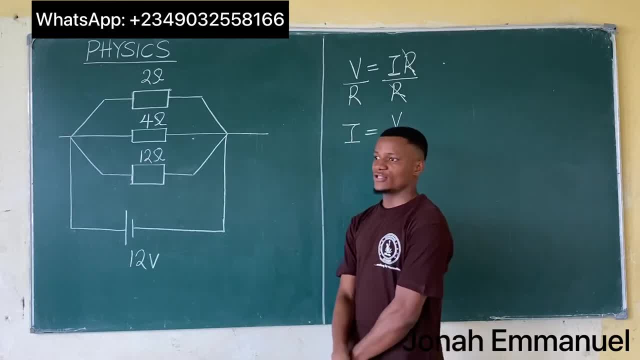 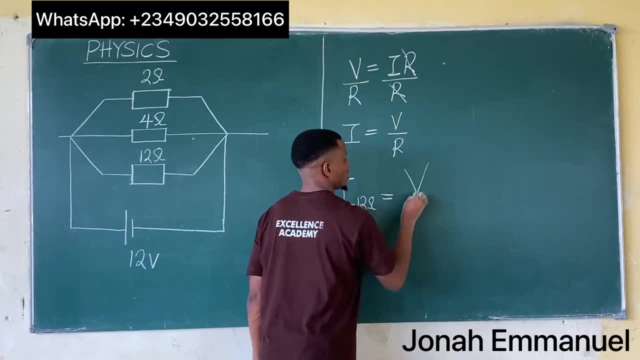 actually find the current flowing through the 12 ohm resistor. so i'll say current flowing through the 12 ohm resistor is equal to the potential difference of the 12 ohm resistor all over the resistance of the 12 ohm resistor. it's this simple, all right. 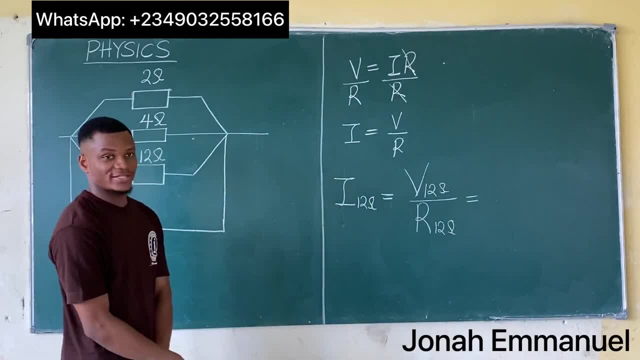 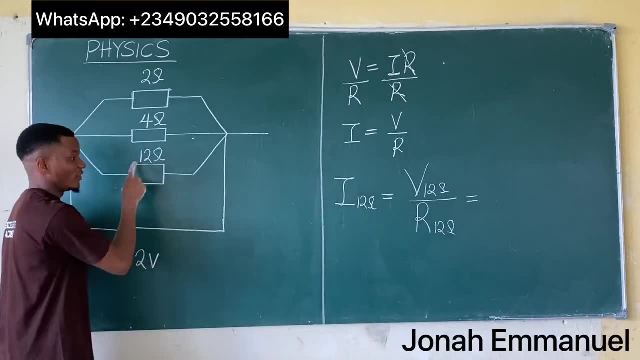 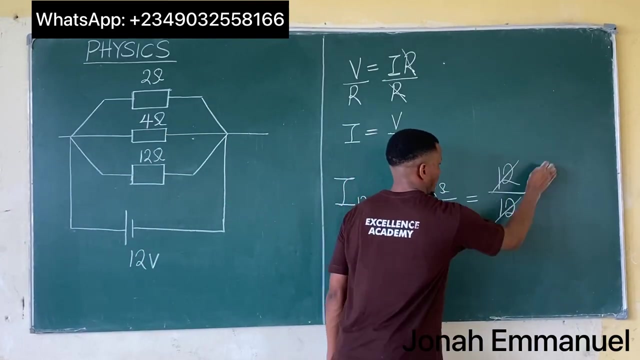 so you express this formula in terms of the 12 ohm resistor. since you said the same potential difference or the same voltage flows across each of them, then that means v12 is equal to what i have here, 12 volts all over the resistance of the 12 ohms resistance is 12, so 12 here, 12 here 1. 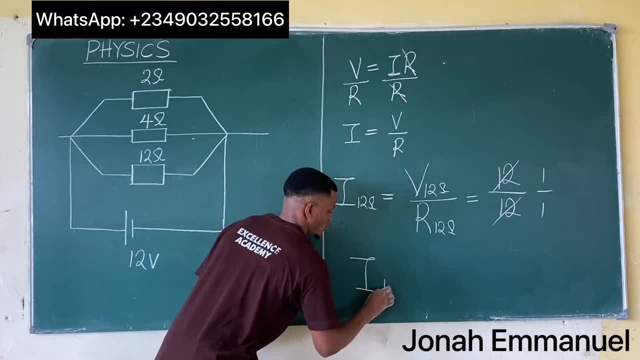 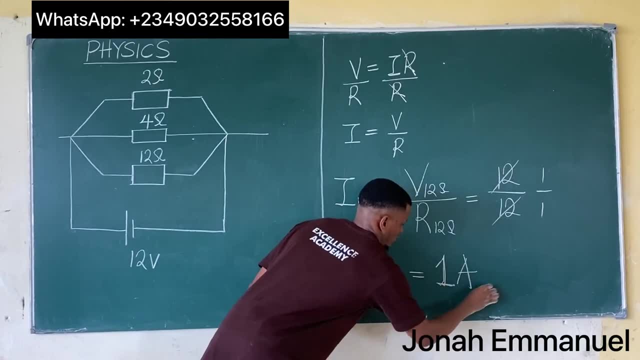 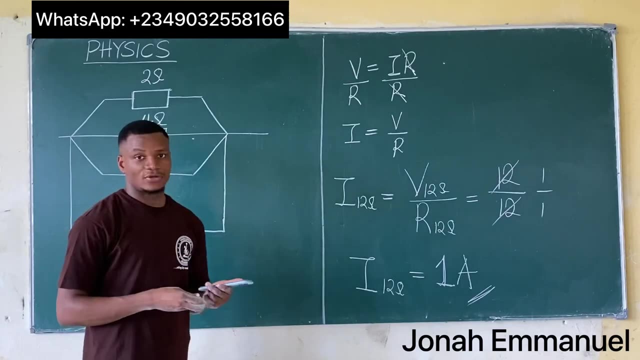 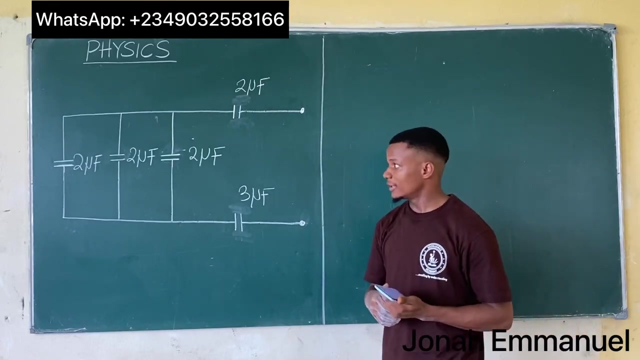 all over 1, hence the current flowing through the 12 ohm capacitor is 1 ampere. so the answer is 1 ampere and this is option d, 1.0 a. so that's your answer. this is how you solve this. all right, let's try another question. um, it says: calculate the effective. 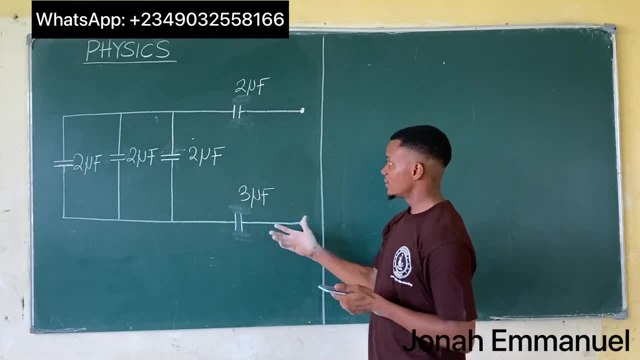 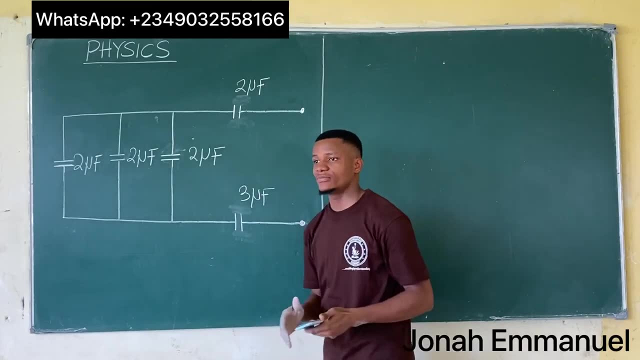 capacitance of the circuit above. so we have this section. we have to find the equivalent capacitor. now we said, for structures of this nature, we start from the closed end to the open end, which in this case is from here to this point. so how do you analyze this? i'll tell you that one, two, three are in parallel. all right, i would say for. 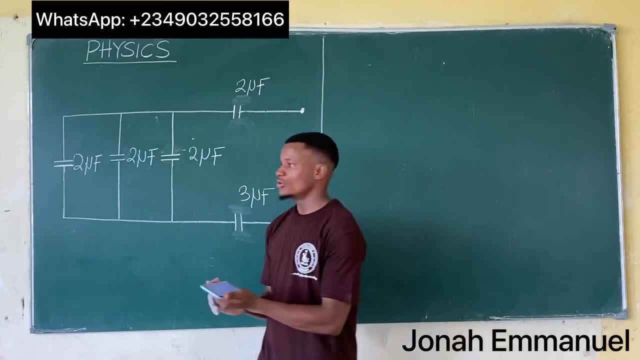 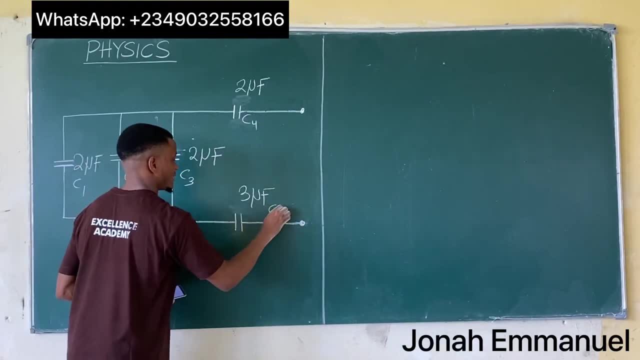 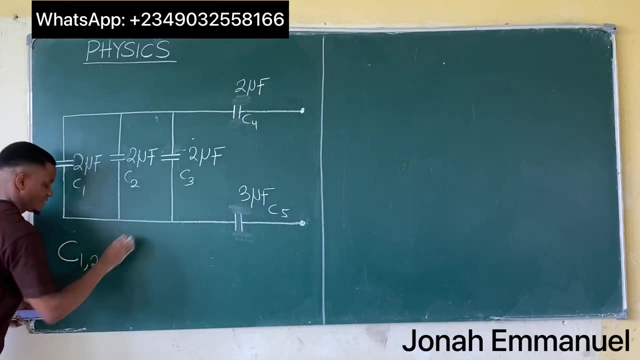 parallel connection of capacitance. simply add up the value, so i'll have that if i call this c1, c2, c3, c4 and c5, i'll have that the equivalent of c1 and c2 and c3 is equal to c1 plus c2 plus c3. this parallel 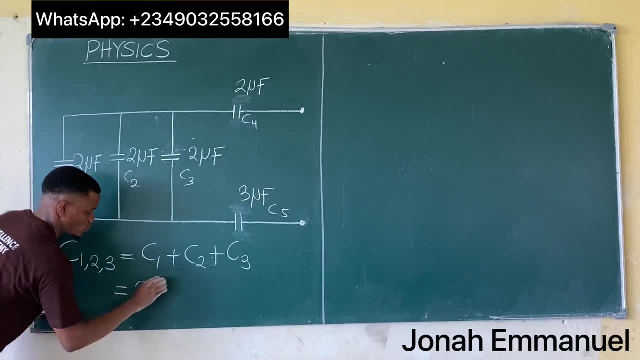 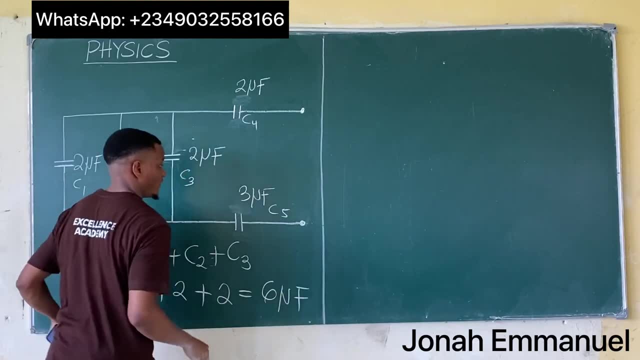 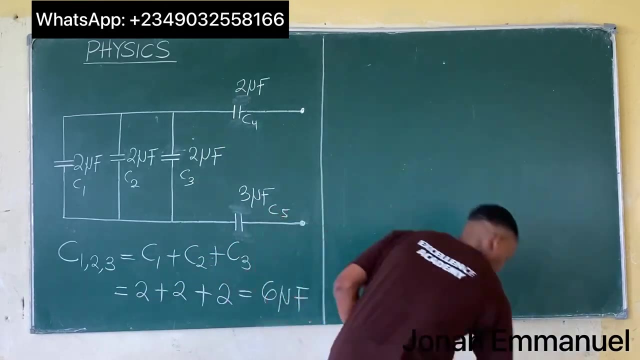 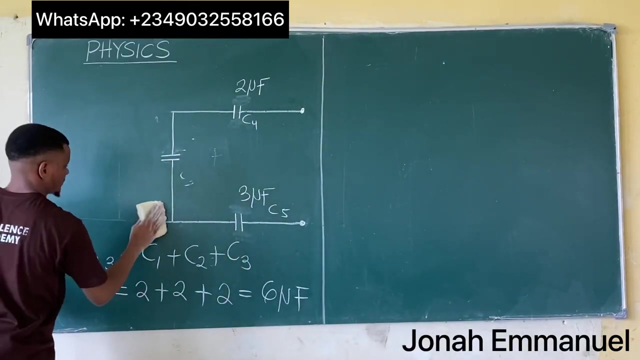 condition of capacitance. that's equal to 2 plus 2 plus 2, that's equal to 6 micro farad. this value. now c123 will now come this way. so, as you can see, c1 square now comes this way here. so this is now in series with c4. 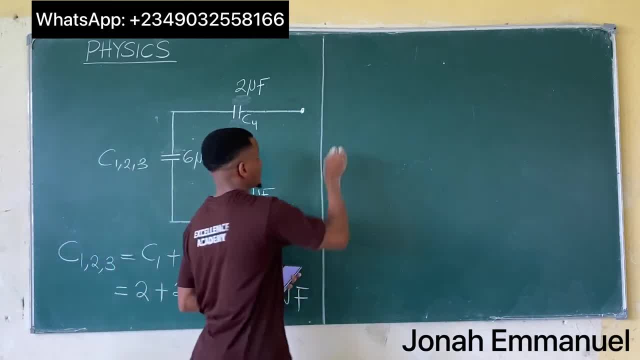 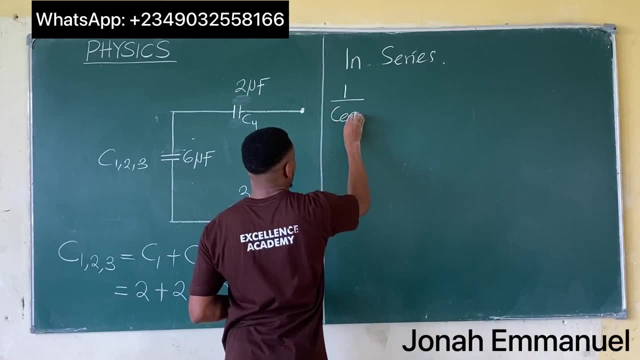 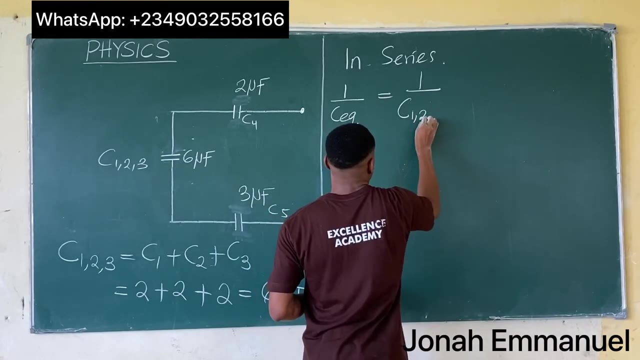 and c5, so hence in series. so this is now in series with c4 and c5, so hence in series. so hence in series, in series. i will now have that. my equivalent capacitance, don't forget we said series capacitor will take in that. so it's equal to 1 over c123. that's this plus this. 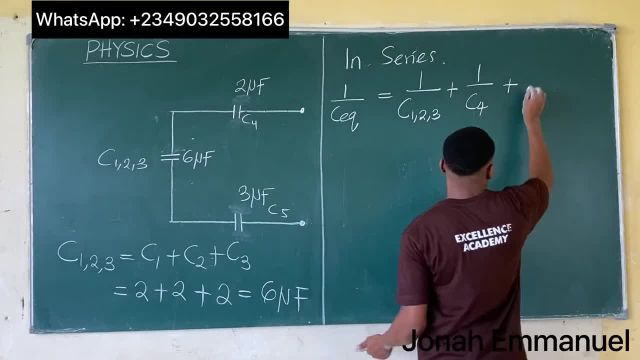 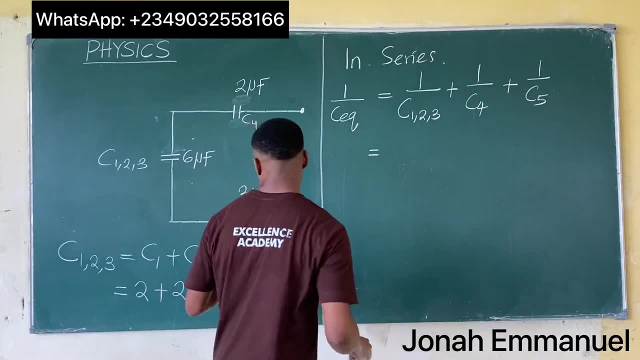 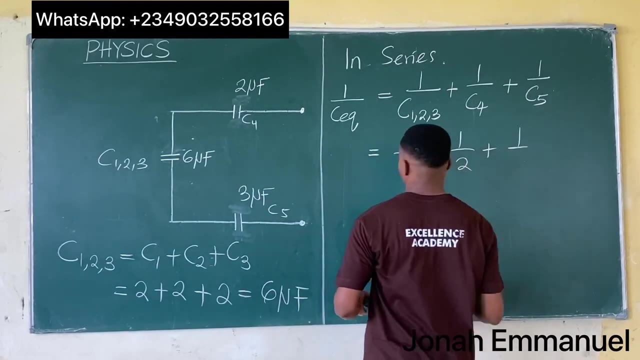 1 over c4 plus this 1 over c5. all right, so i have this is equal to 1 over c123 is 6, so 1 over 6 plus 1 over c4 plus c2 plus 1 over 3, all right. 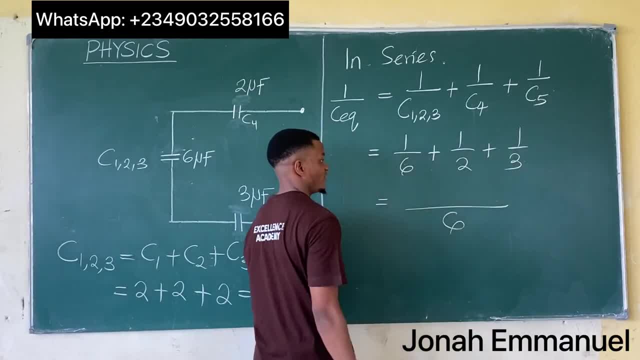 from here. obviously the lcm is 6, lcm 6236: 6 over 6 is 1 times 1. 1 plus 6 over 2 is 3 times 1. 3 plus 6 over 3 is 2 times 1. 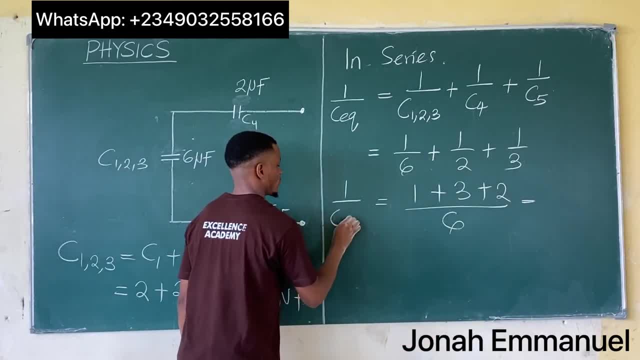 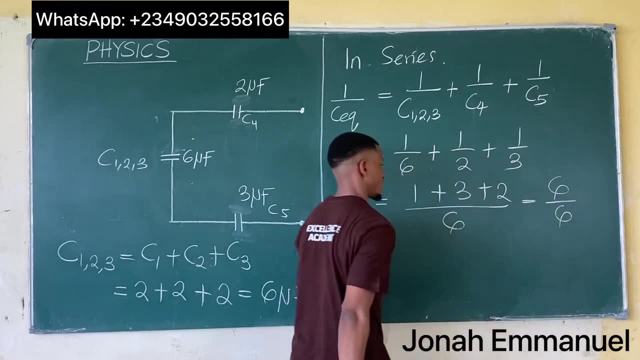 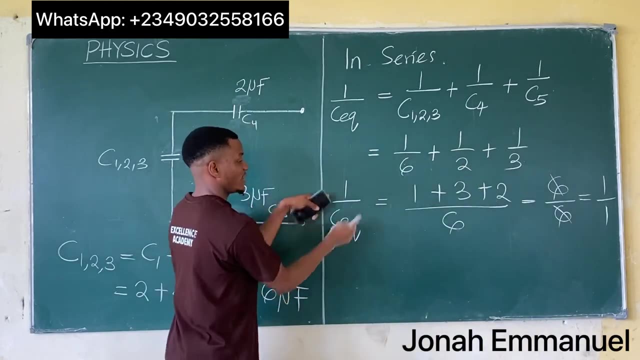 so that's equal to: so i have 1 over to 1 plus 3, 4 plus 2, 6 over 6. So this is equal to 1 over 1.. We can't start to give you 1 over 1.. So guess, if you take inverse. 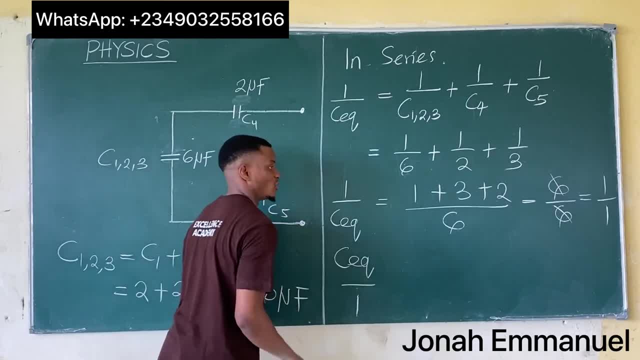 So CEQ over 1, which is CEQ, that's equivalent capacitance, is equal to 1 over 1.. So hence, of course, this over 1 is itself. So the equivalent capacitance is equal to 1 over 1.. 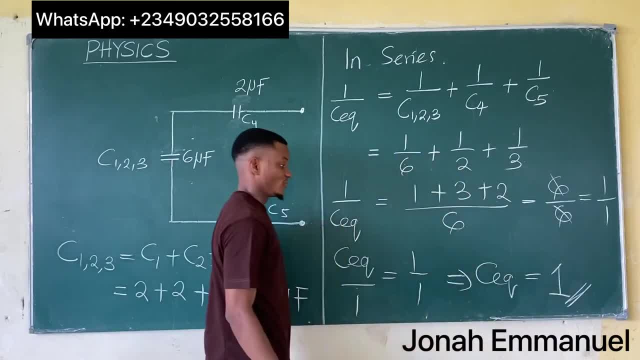 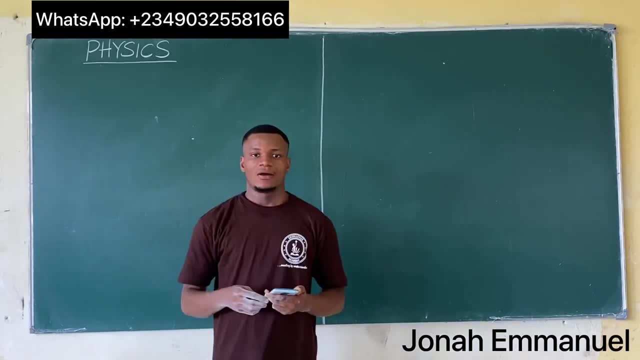 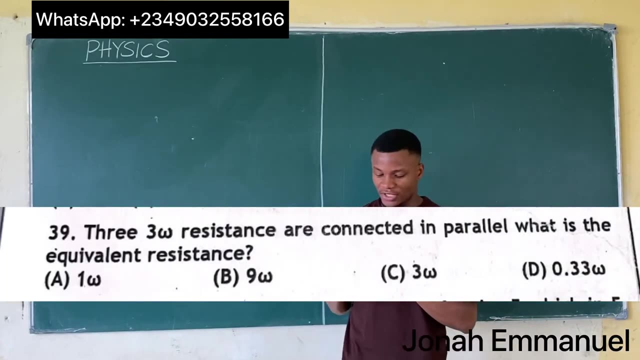 And that's what I have, this value. So this is how you solve this. We'll take one final example and we're done for this class, Alright. so we'll take one final example for today's class. Our discussion says 3, 3-ohm resistance. 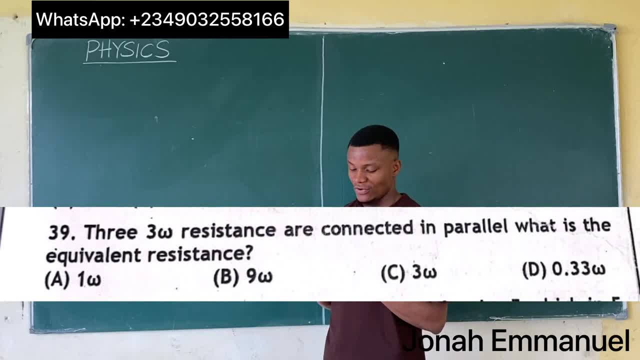 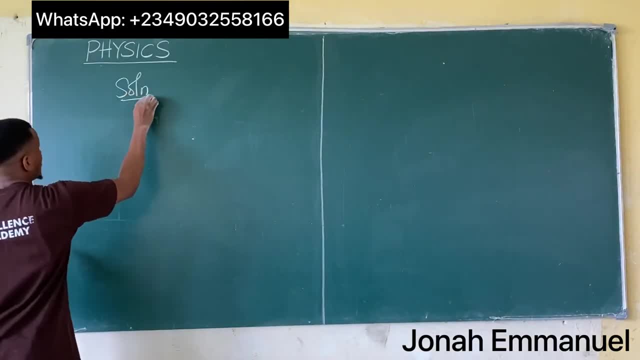 which should be resistances- are connected in parallel. What is the equivalent resistance? Quite simple, So solution: so we said 3, 3-ohm resistances. So R1 is equal to 3, that should be ohm, not omega. 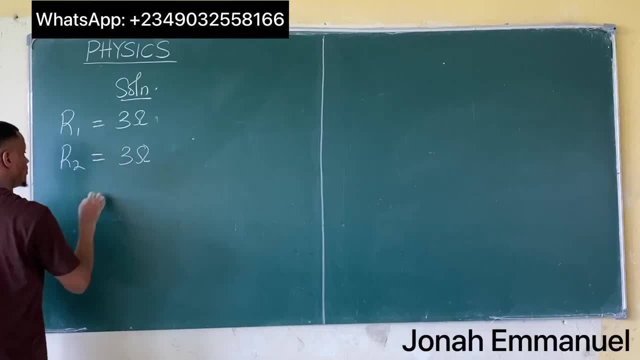 R2 is 3-ohm and R3 is 3-ohm, So that is 3, 3-ohm resistances are connected in what? Parallel? Alright, so parallel connection. we have that So that one over the equivalent is equal to 1 over R1 plus 1 over R2 plus 1 over R3..